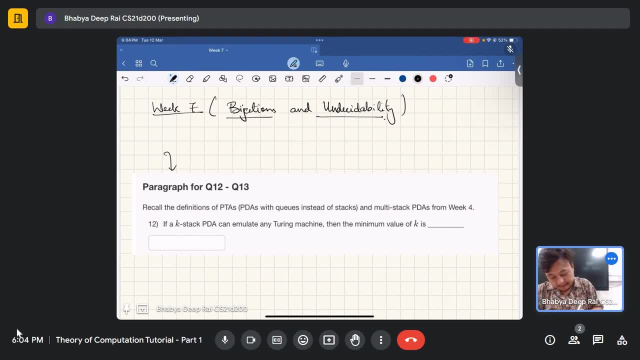 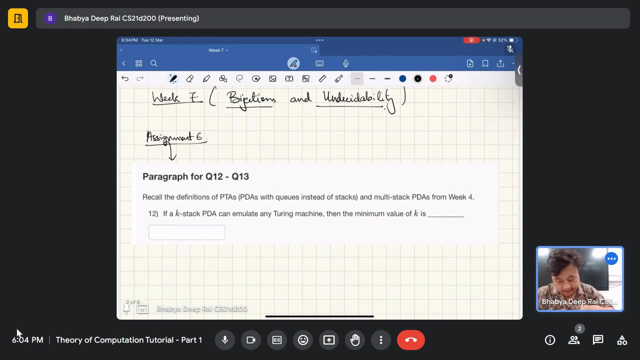 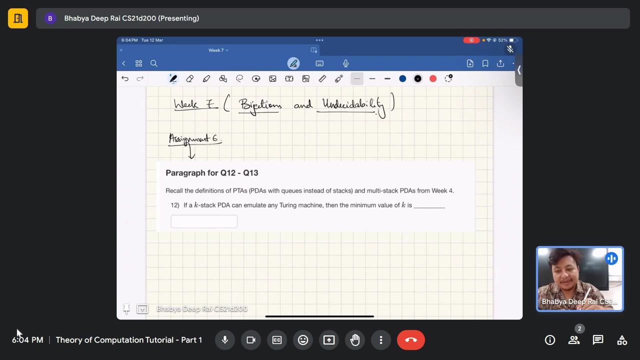 from the previous assignment. This is from assignment 6.. I will leave out the simpler ones for you and we will discuss only the tougher ones. So I have picked these two questions- questions 12 and 13- from the assignment 6.. So let me begin with the discussion. 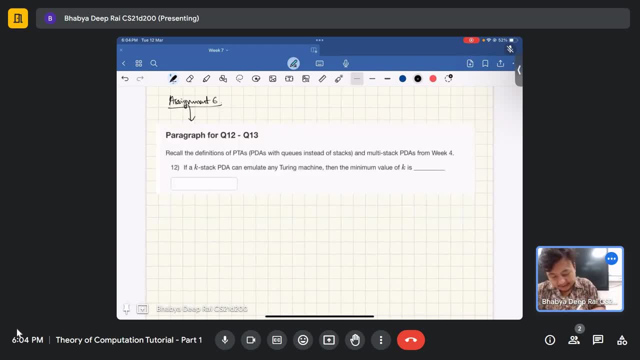 So the question says the following: Recall the definitions of PTAs. Now, what are PTAs? PTAs are just PDAs with queues instead of stacks And multi-stack PDA from week 4.. So I think you guys remember, but I will just repeat: PTA is again what This is, just a PDA. 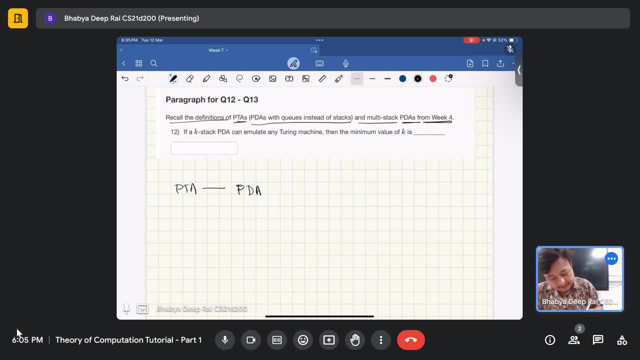 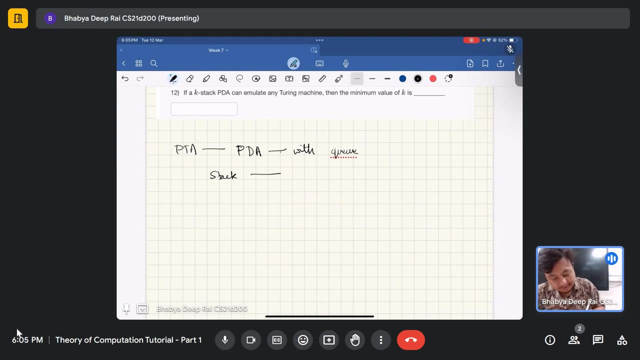 See normally, what does PDA have? PDA has a stack right, But with queue instead of a stack. What is stack? Well, stack is also what is called the first in first in last out. So the idea is that PDA has a stack right, But with queues instead of a stack. What is stack? Well, stack is also what is called the first in, first in last out. 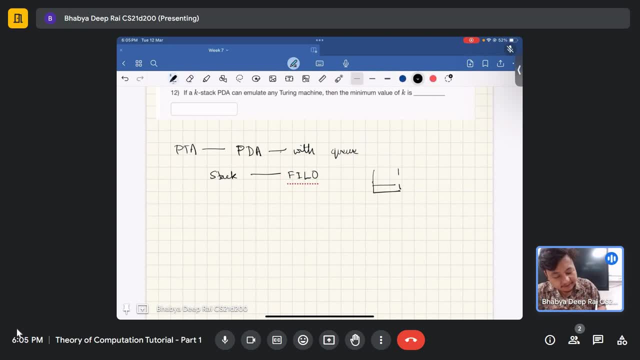 And you can just keep. I just keep what is called the push operation. I can keep pushing and then I pop. Or instead of saying first in last out, I can even say last in first out. I think that is how it is generally called. 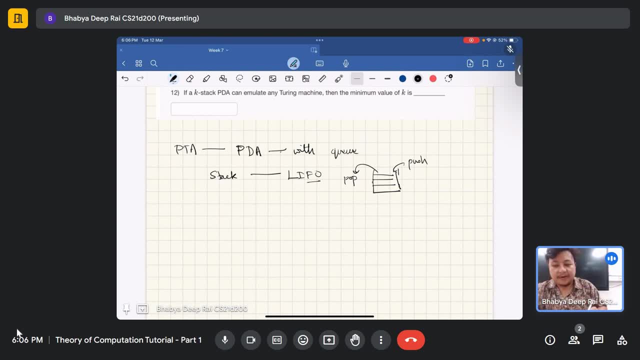 The last to be pushed is the first to be popped, Okay. And whereas, what is a queue? A queue is Like a queue of people, right? So the first person to go in is the first person to come out. So the pushing happens at the end, right, And the popping happens at the back. 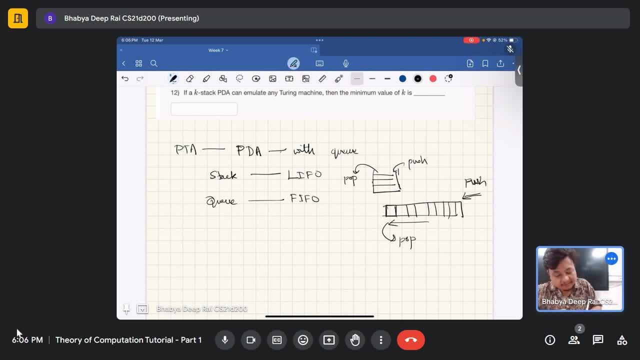 So queue is an example of a first in, first out system data structure. First to go in is the first to come out. Now, what are PDAs? PDAs are like DFA's right: You go from one state to another. It is just another computational machine. 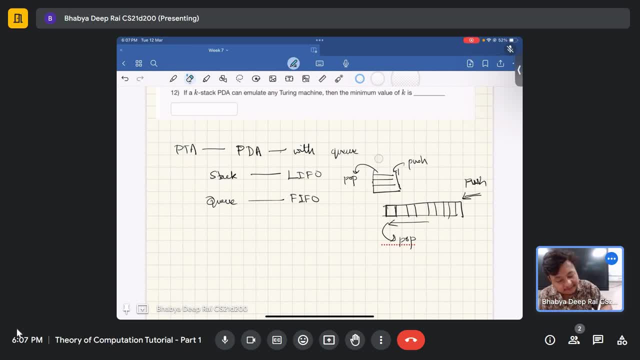 But the machine has a special memory which is of the form of a stack, And whereas PTAs we are saying, instead of a stack, we have a queue. Everything else remains the same. There are number states and some kind of tape alphabet where you can. 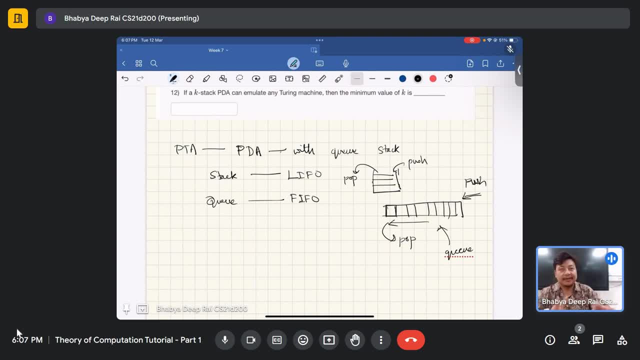 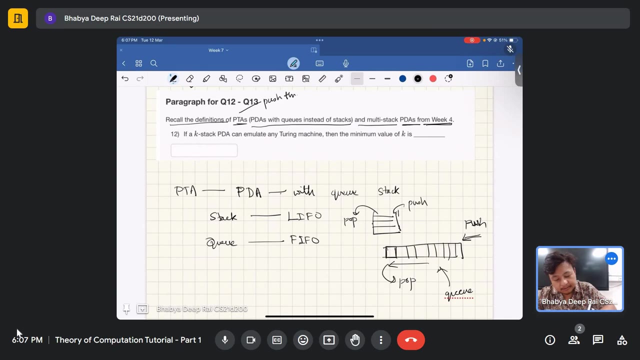 you can push it on the stack, You can push it on the queue, and so on. Everything remains the same, Only that it is a stack instead of a queue, And we proved some results in the previous assignments regarding PTA. This was what is called the push-through automata. 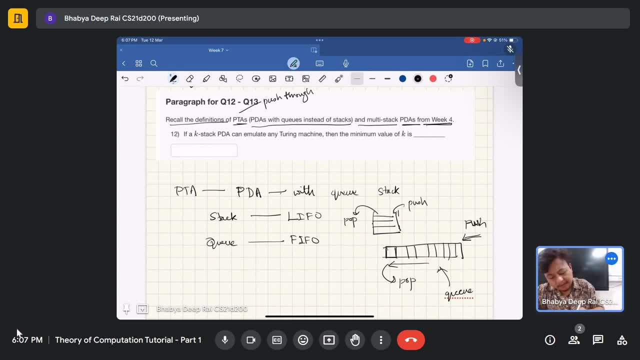 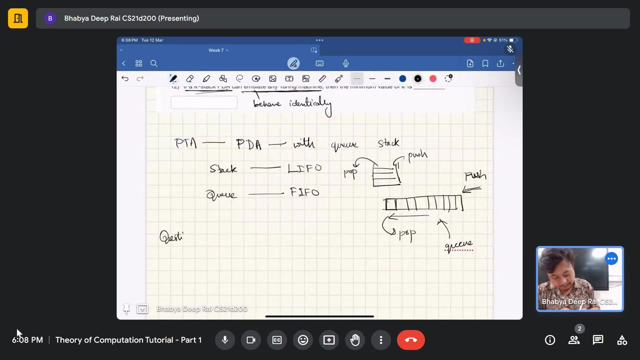 Anyway, what does the question say? If a k-stack PDA can emulate any Turing machine, what does emulate mean? It can behave identically, It can behave like a Turing machine. Then the minimum value of k is something. In other words. question says: 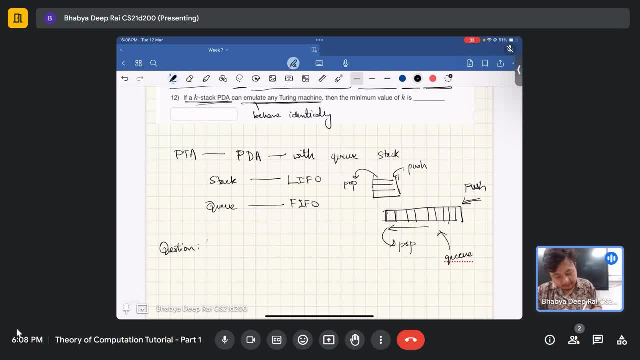 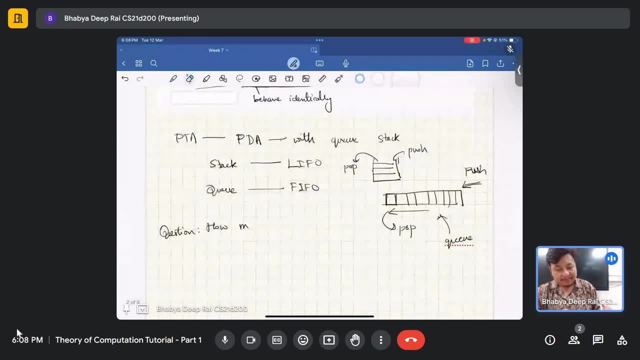 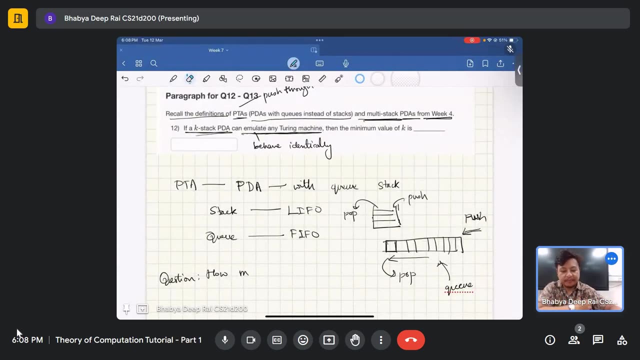 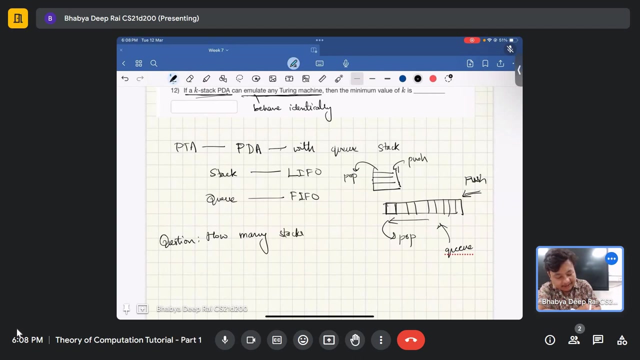 if I rephrase the question, it says how many? also a multi-stack PDA. multi-stack PDA is just a PDA with several stacks, two stacks or three stacks or something like that. Okay, So the question says how many stacks are needed to simulate a Turing machine. 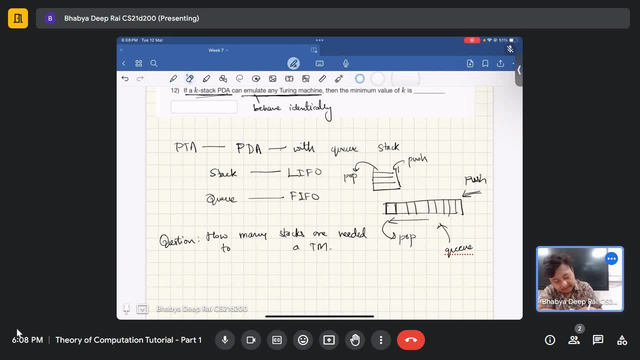 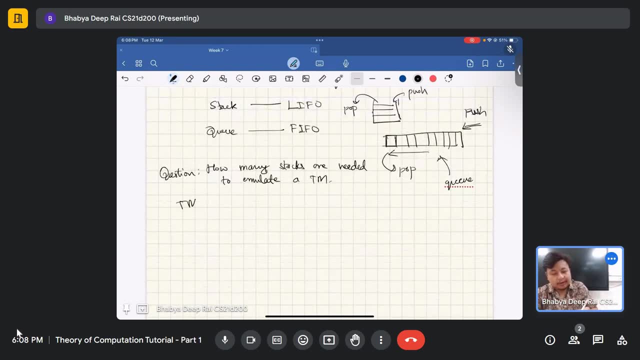 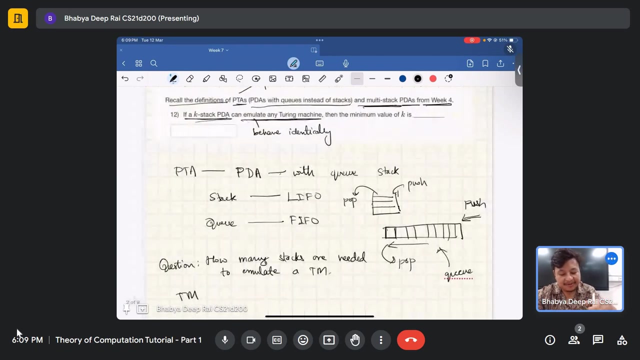 emulate a Turing machine. This is a correct word actually. Now, what does a Turing machine is A Turing machine, again has state, It has several symbols and so on, But the main thing that distinguishes it from you know, a PDA or something like a PTA? 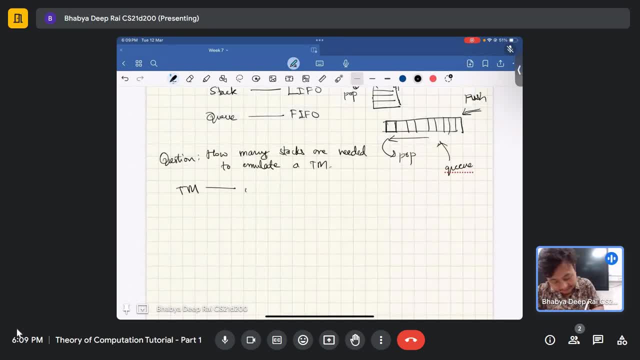 or a finite state machine is the fact that it has an infinite really long tape. So it has a tape And you can write wherever you want- A, 0,, B and so on- And you have a head Right And this head can move right. 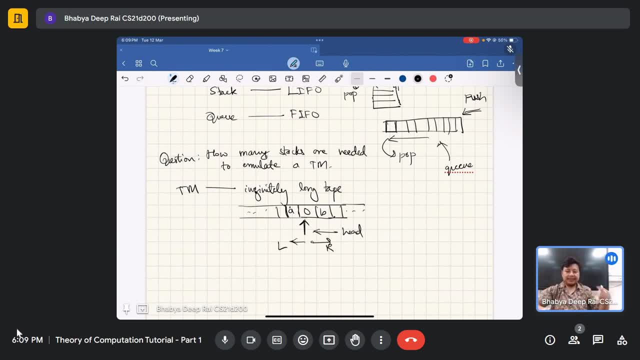 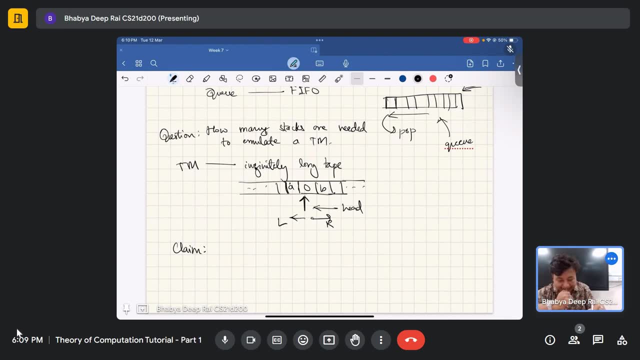 Or left, And then it can make changes as you go along. My claim is okay. So the question says: if I am allowed to have several stacks, if the PDA is allowed to have several stacks, how many stacks are needed to sort of simulate this motion? 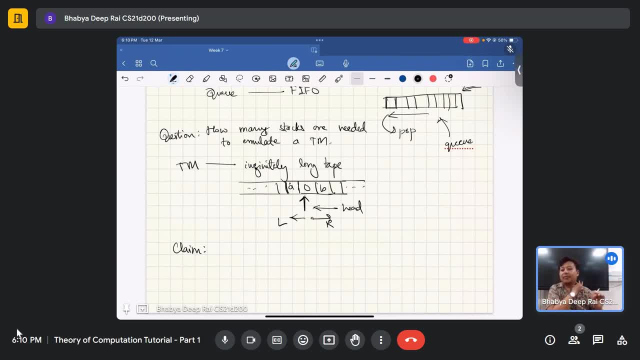 sort of behave like a Turing machine. do everything that a Turing machine can do. My claim is that two stacks are enough. My claim is that two stacks are enough. Why Let the two stacks be A and B? Okay, So let's see. 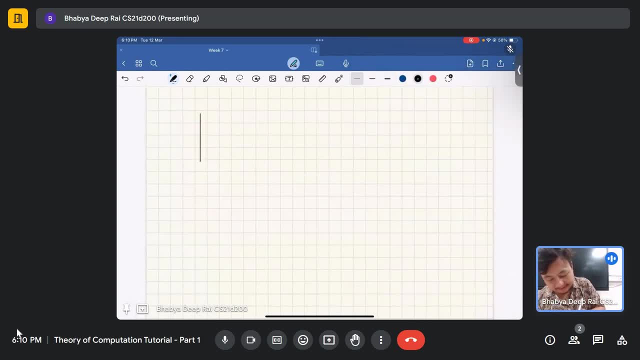 Let the two stacks be A and B. So this is what the stack looks like. There's another stack, Okay, And let's say there's a bottom symbol dollar. Okay, Now this dollar tells that the stack is empty. Okay. 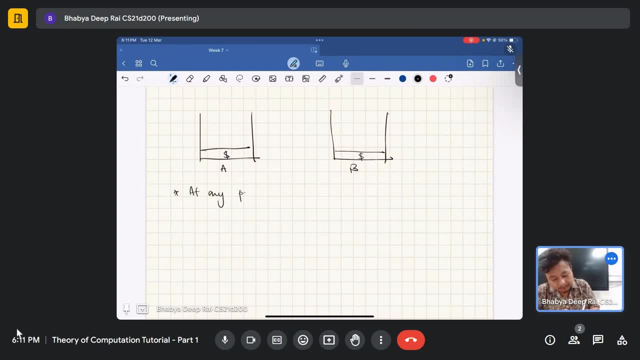 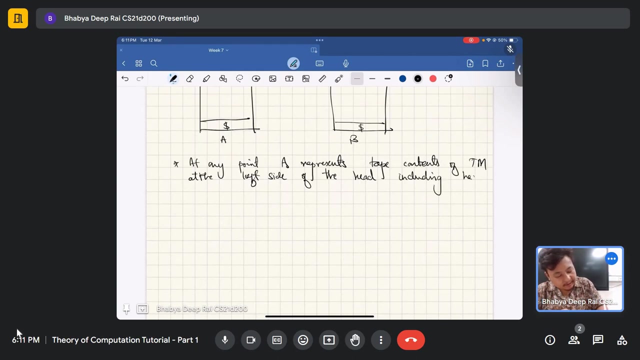 Now, at any point: Okay, represents tape contents of the Turing machine. Okay, At the left side of the head position: Okay, And including head Current symbol: Okay, And same thing at any point. Stack B: what does stack B do? 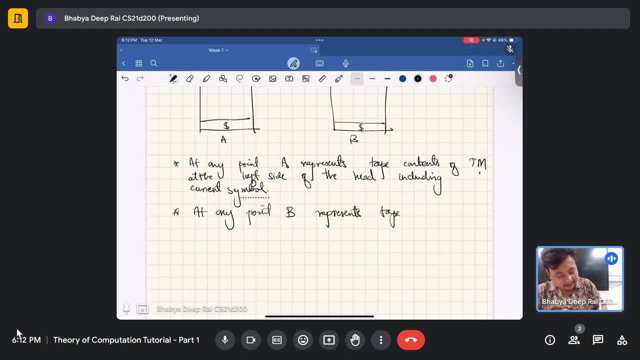 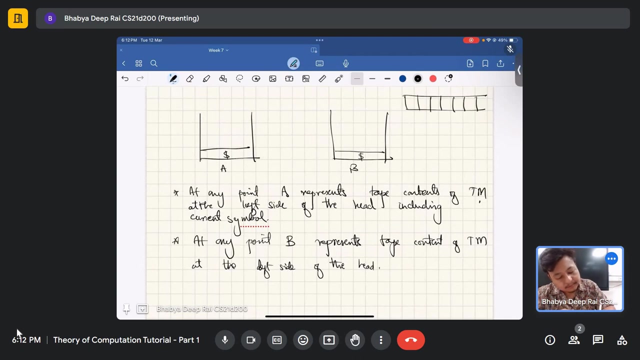 Stack B represents the tape content of the Turing machine at the left side of the head. What does it mean? Example: let's say this is the tape content. This is the tape. Okay, Now let's say the head is pointing here. 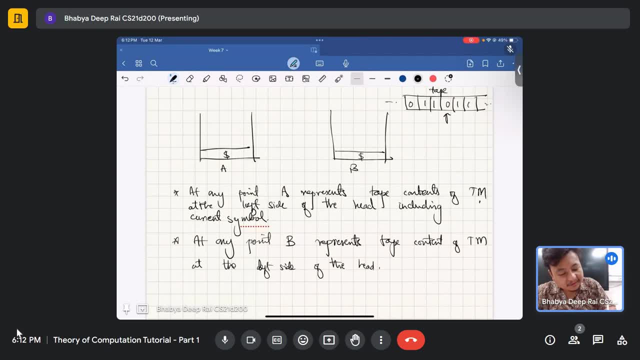 And the symbol is 0, 1, 1, 0, 1, 0, 1.. Okay, And let's say, since we know that an infinitely long Turing machine on both sides can be written as a Turing machine with: 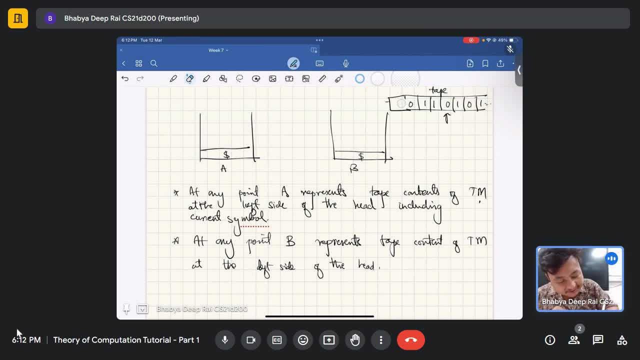 infinitely long tape only on one side. Let's say this part is the end left end marker, Or let's just keep it like this. Okay Then what does the corresponding stacks on the PVA look like? The two stacks It will have this: 0,. 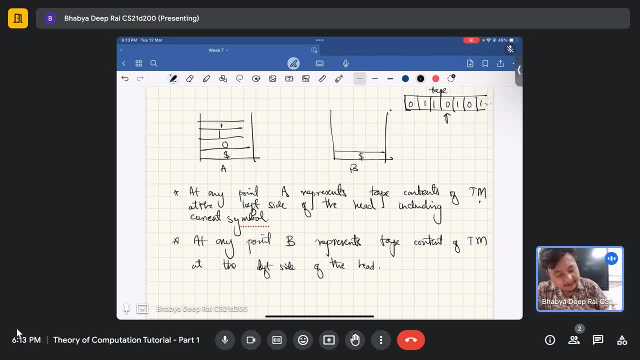 1, 1.. Okay, And along with the head, along with the current position, the current position is 0.. Next, it has 1, 0, 1, 1, 1, 1, 0,. 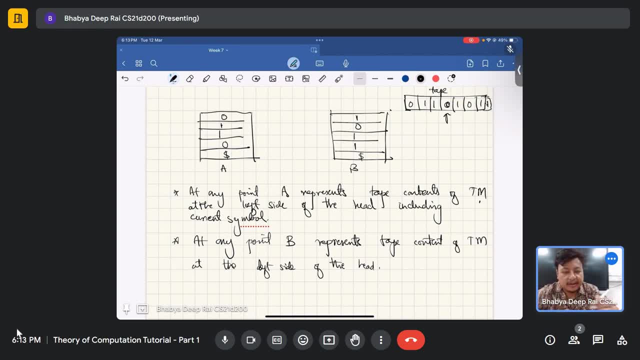 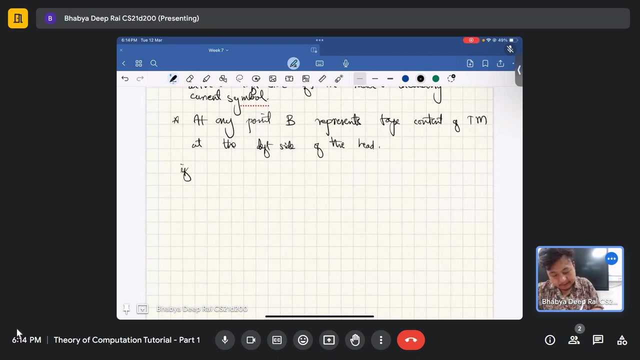 1. Okay, And this is the current position. Okay, This part is this part, And let me choose a color: green. This part is this part. Okay. So I hope you can already see where this is going Now. if 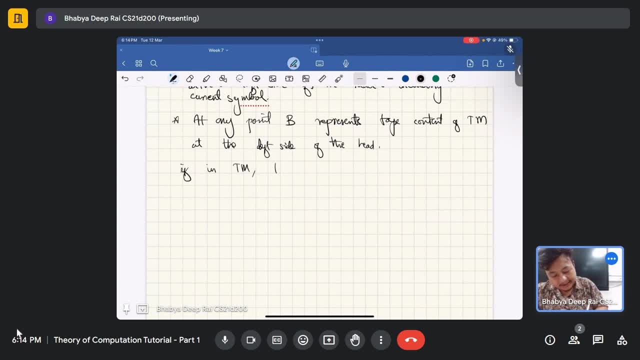 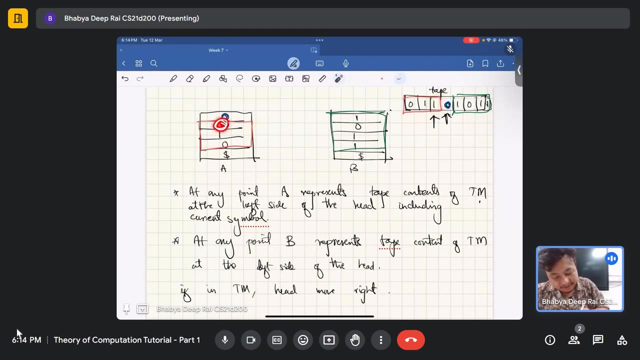 in the Turing machine, head moves right, then instead of pointing here, I should point here: No, which means this symbol should be on top of the stack. Right, I should be pointing here. So this symbol should be on top of the stack. 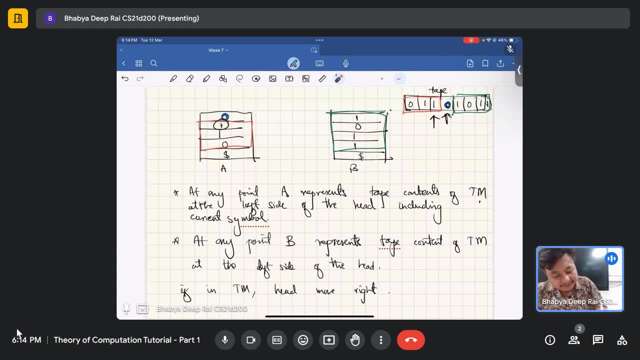 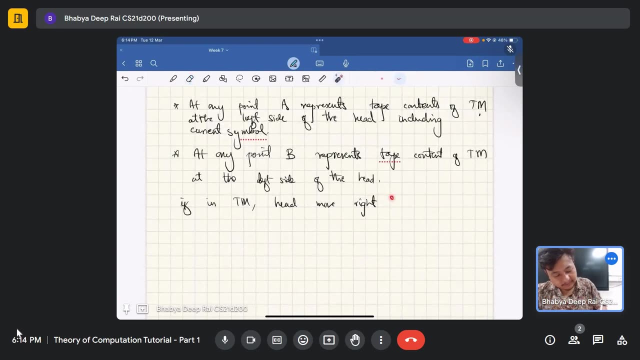 And now 0.. Okay, This will no longer be there And therefore 0 will be to the right. So 0 will. should be here, Shifted there, Right? Well, so if head moves right, okay, then pop. 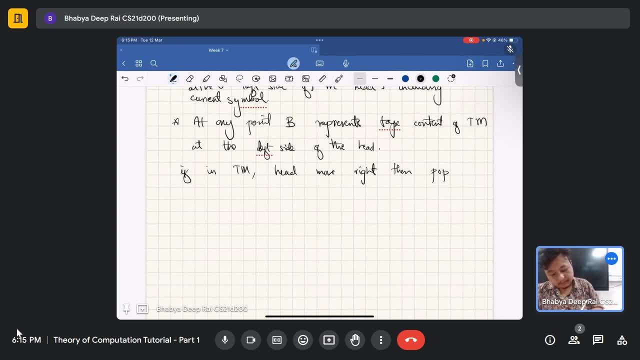 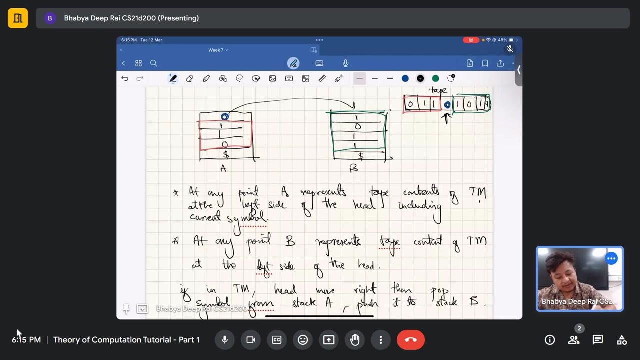 pop symbol from stack A. push it to stack B. Pop symbol from stack A. push it to stack B. So this 0 will be pushed here. So now the top of the stack A represents the correct symbol. Okay, Top of stack A is the current symbol. 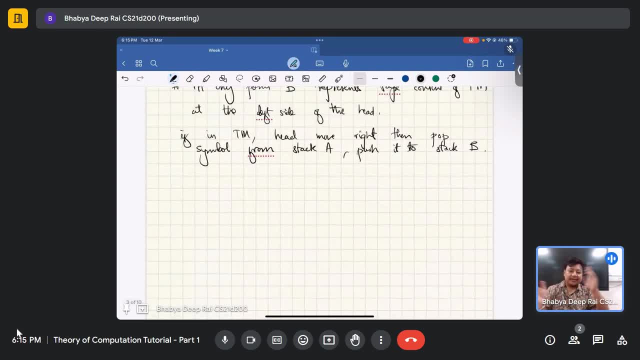 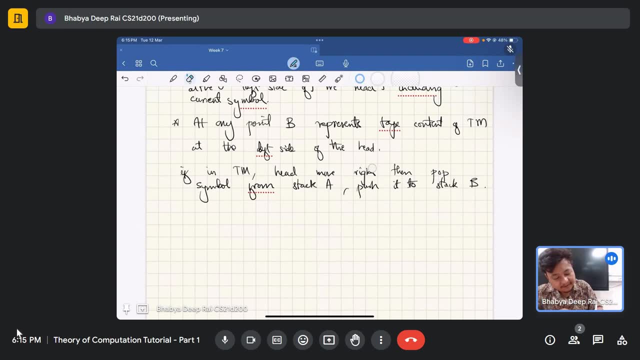 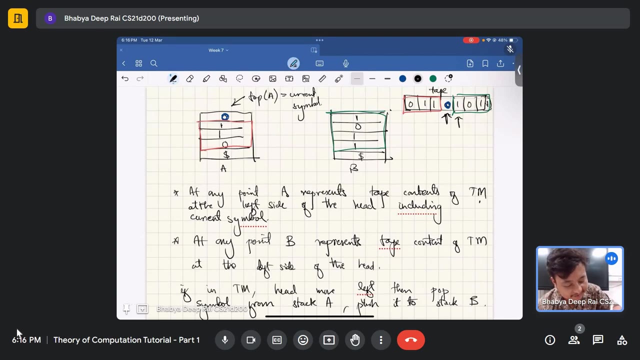 So we can now already tell what happens if the head is supposed to move left, Right. So if if I move- sorry, this is for left, So sorry- Head moves left, then, so if head moves right, then this guy is supposed to be. 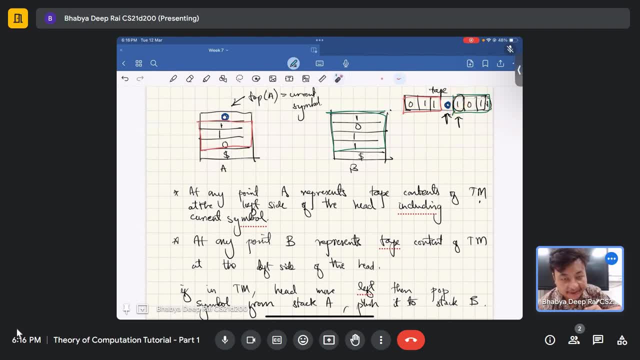 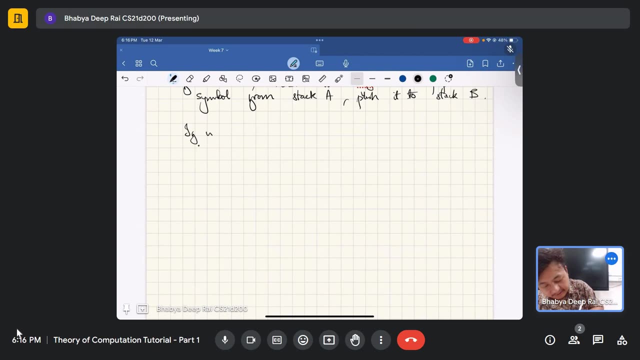 the right. this guy is supposed to be the top of the stack of A, So from B I will pop and push it onto A. If in the Turing machine, right head moves left, if the head moves left, then what are you supposed to do? 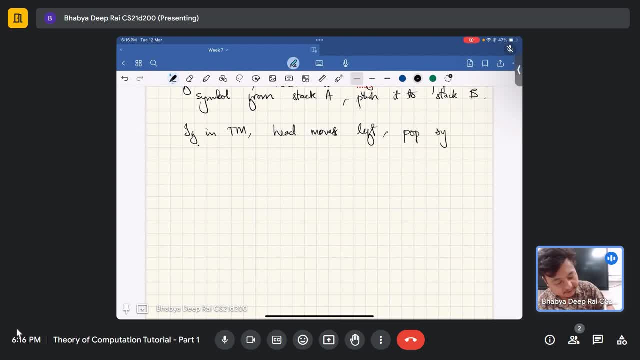 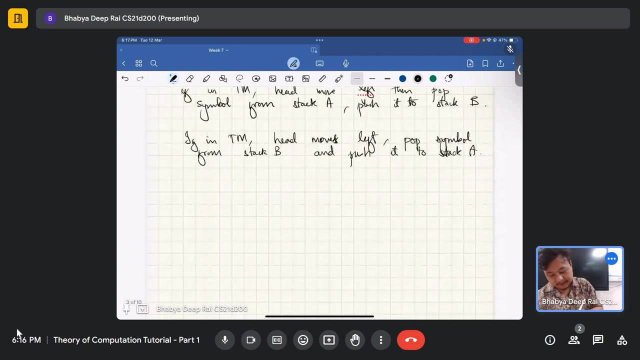 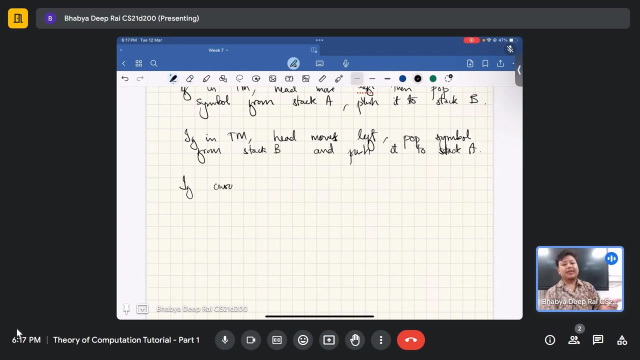 Pop symbol from stack B and push it to stack A, Because that is the new head position Right. And if current and what is Turing machine also capable of doing Wherever it is pointing, it is able to change that particular element also. 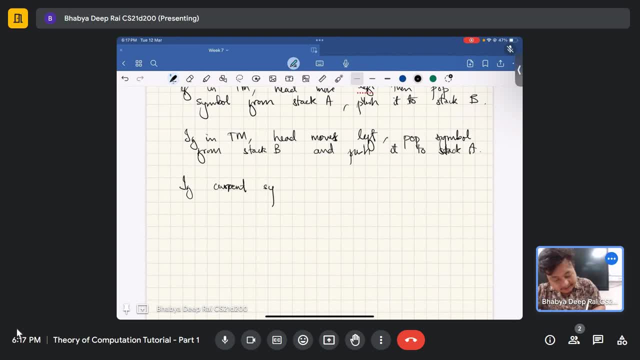 Right If current symbol is changed from say A to B, Right Where A, B, okay it is changed from say: some symbol A and 2, some symbol in B, A, B are in tape aspect. 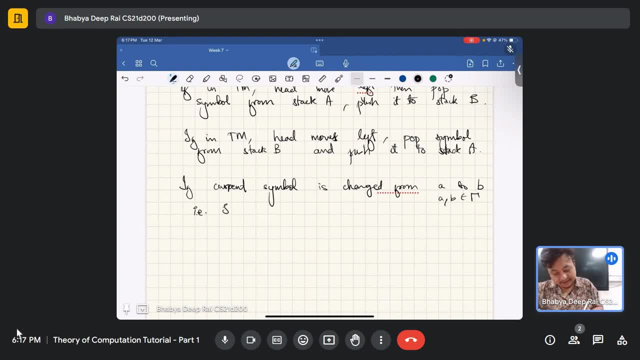 Or, in other words, in terms of Turing machines, in terms of transition function, it will be like delta of the current symbol, no current state QI A is equal to some QJ A will be changed to B. 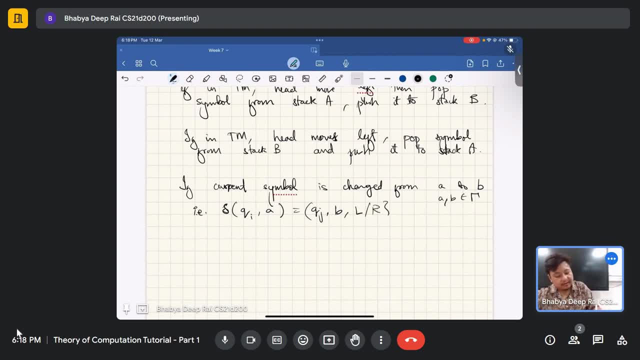 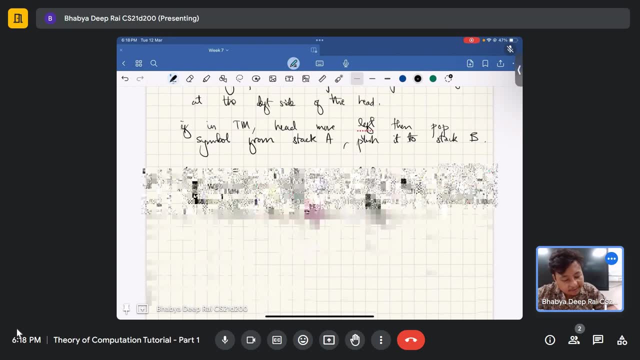 and then either move left or right, Right, Either left or right. If such a thing is happening, then then what if that is, this zero here that we are pointing at, is changed to 1, what are we supposed to do? 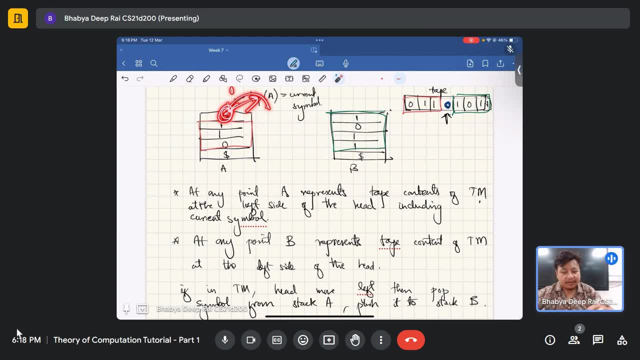 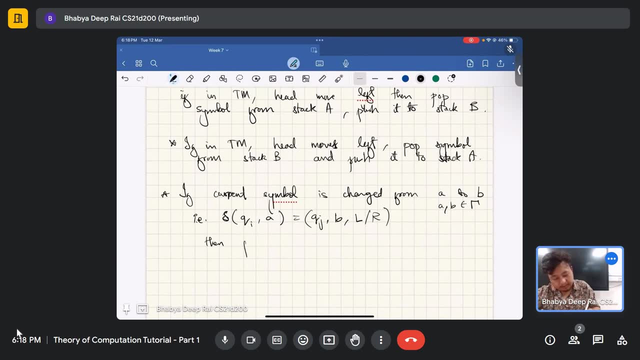 We are supposed to pop from A and push that new symbol onto A, Then pop top symbol from A Right. That is this. this current symbol is: A is popped out and pushed B to stack B. That is all. 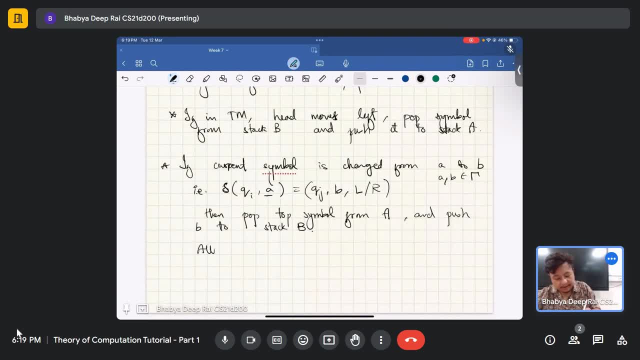 So all of the- so all of Turing machines' behaviour is captured by PDAs with two stacks. so anything that a Turing machine can be done, can do, can be done by a PDA with two stacks. so answer is 2. so just, we see that just by. 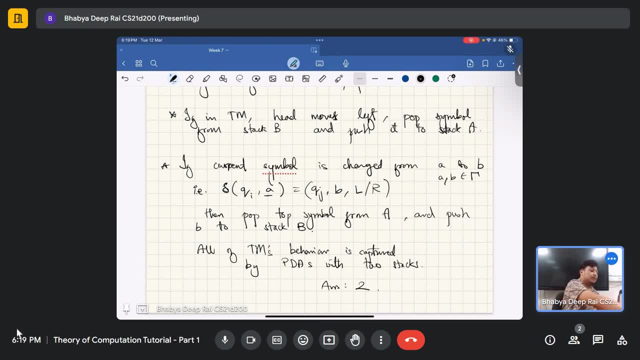 increasing the stack by one. it makes the machine so much more powerful. additionally, by the Church Turing thesis, it is said that Turing machine is the most powerful machine that you can have. anything an algorithm can do, a Turing machine can do so. just by adding two stacks you are able to do so. 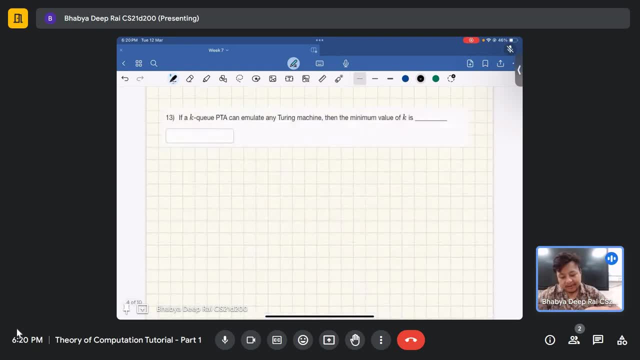 much more okay. so let's go to the next one. if a k-Q PTA can emulate any Turing machine, then a minimum value of k is. so now we have asking: what is the? this question, in other words, says: what is the number of Qs? what is the number of Qs 2? 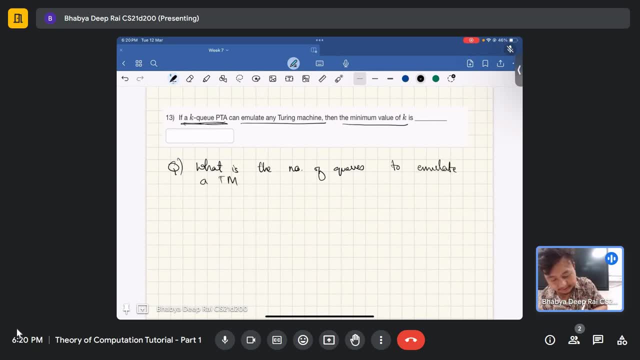 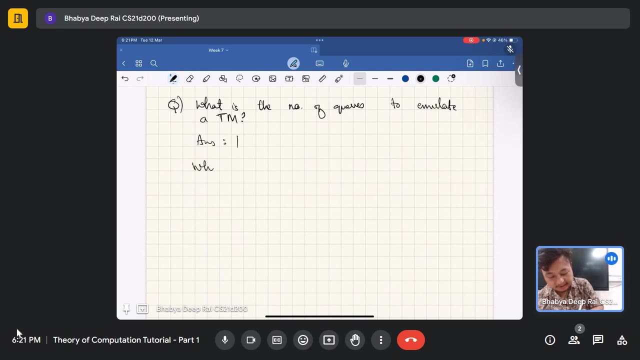 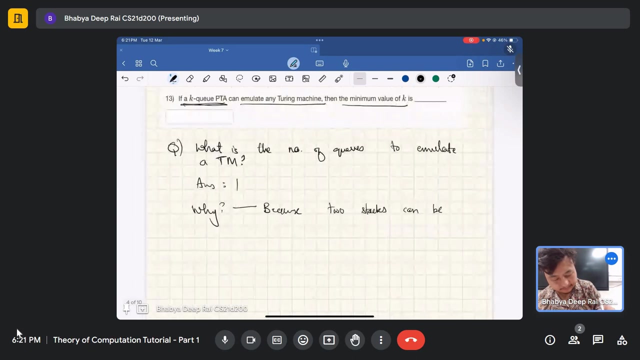 emulate a Turing machine. this is the question. the answer is just one: why can we answer it so easily? because two stacks can be simulated by a single cube. okay, you can use a single cube to simulate two stacks. well, using a single cube, how would you simulate just one stack? okay, I think we've done it before. 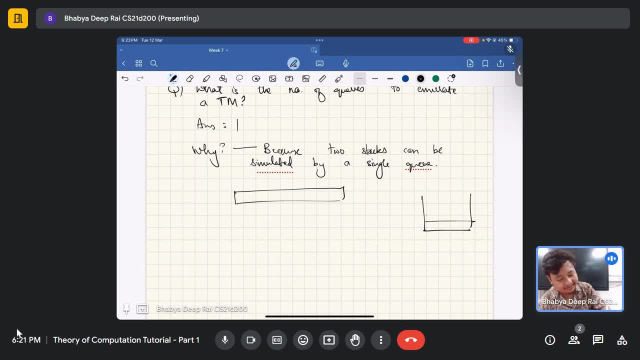 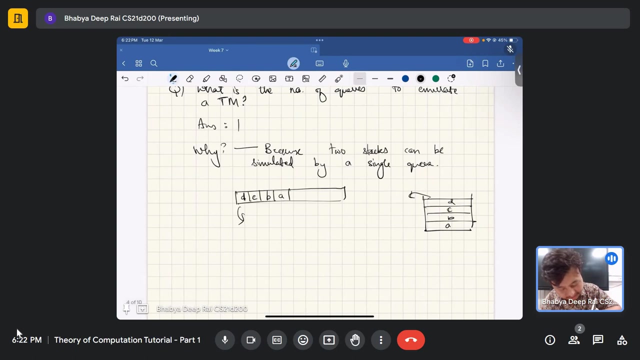 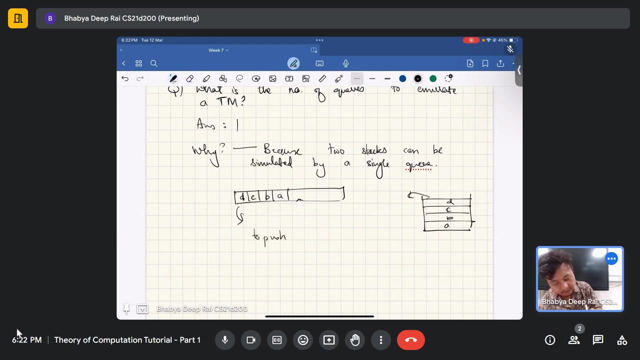 once. so we were imagining the stack to look like this: ABCD, okay, and the cube would store something like this: sorry, DCBA, okay, so DCBA, and if you pop here, you can pop here, and if you want to push something first, you need to. if you need to push, you need to push. 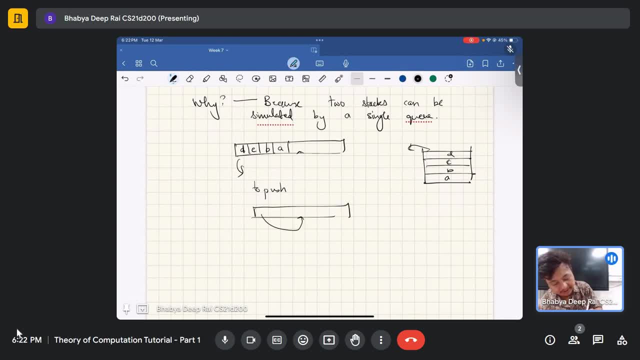 something, then you need to keep popping things at the back and push it in at the back. so first you need to take CBA and say D is popped off, okay once. so if you want to push, you can take DCBA. okay, oh, and you have CBA there, no C. 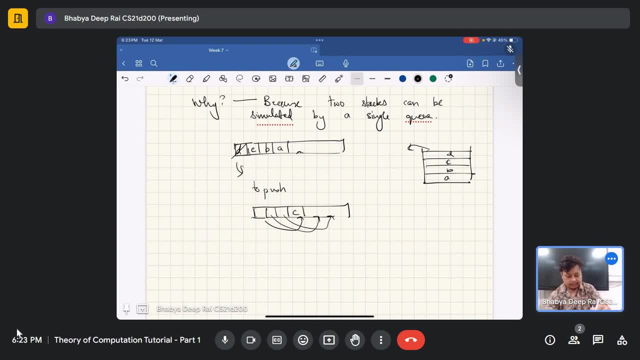 you put a C, you put a, you to push. you first put a D to push first. push, not not D, that's a. I need to push her E, push E, pop D. okay, I pop D first, I push E. okay. now what will my Q look? like I can. 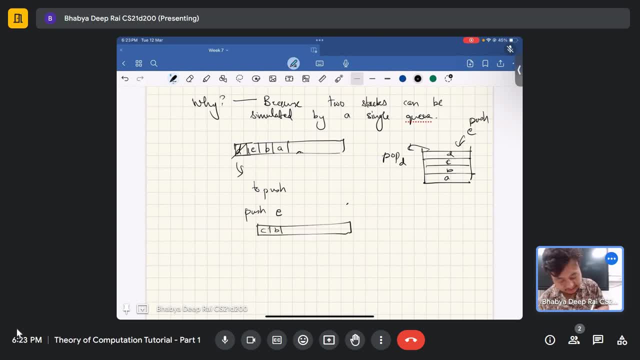 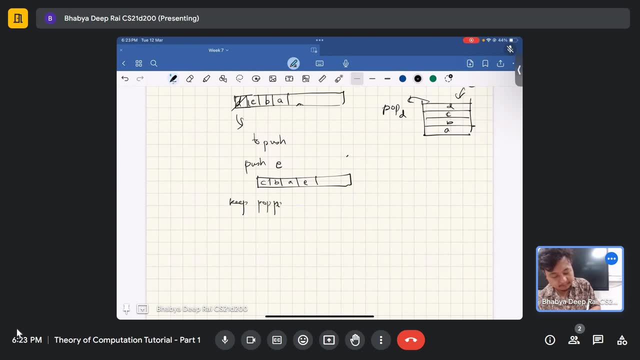 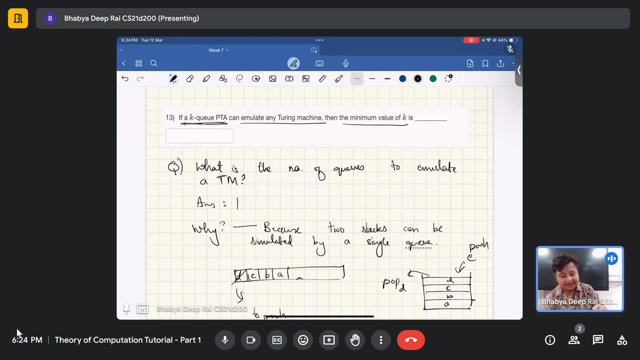 only push it at the back. so C, B, A, then E, next keep popping. what do I do until E is reached? so if I keep popping until he is reached, so I'll get e, C. okay. so this is how I can simulate this. if I simply use need to simulate two stacks, then I can use a. 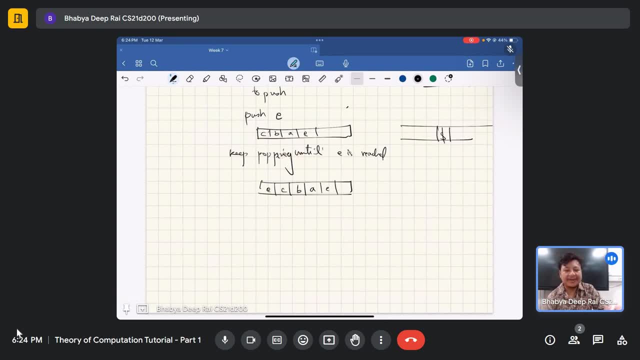 single queue by using our demarcation symbol, let's say our dollar sign, and this part represents the first tag and this represent the second tag. so now, if I the second stack. So this is one way to do it. Another way to do it is, of course, like you can. 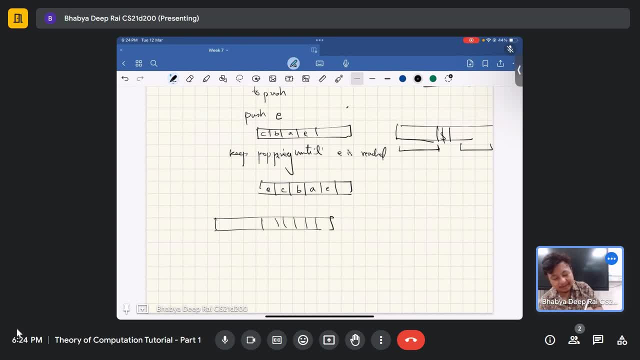 imagine the queue, Imagine the tape of the Turing machine, and then you have the queue here. What you can always do is you can consider the front of the queue, since we only know what is front of the queue and the back of the queue. You can consider the front of the queue. 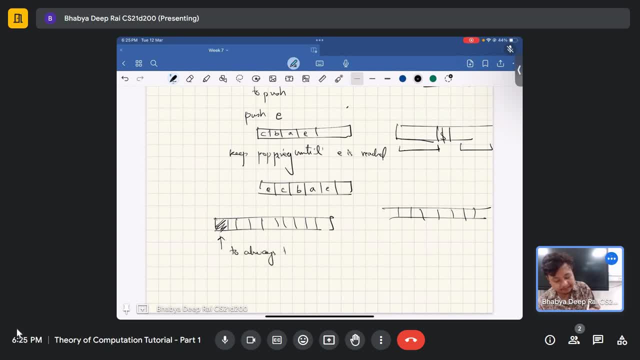 to always represent current symbol. You can always use the front symbol, the front of the queue, to always represent the current symbol. So if this is the current symbol, here have it, And then everything to the left of it, everything to the right of it can be. 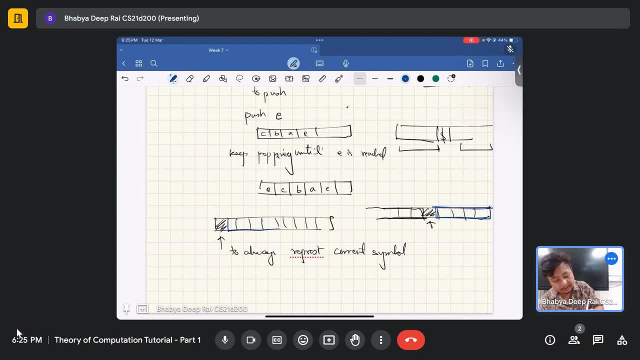 let's say: this is everything to the right I do, and then what you can do is you can add a demarcation symbol. let's call it dollars, and after dollar, whatever will come will represent the left of the cube. so now I'm not going to do it in detail, because it's similar to what I've done. 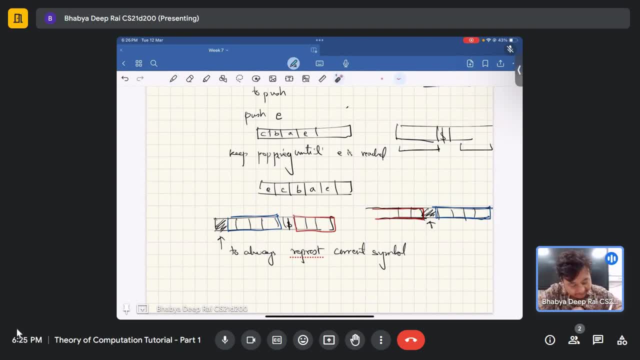 previously. but the idea is that if the head needs to move left, okay, or simpler, let's say: first I'll do. if the head needs to move right, then what will I do? I'll simply pop this from the front and push it at the back, because that is how. 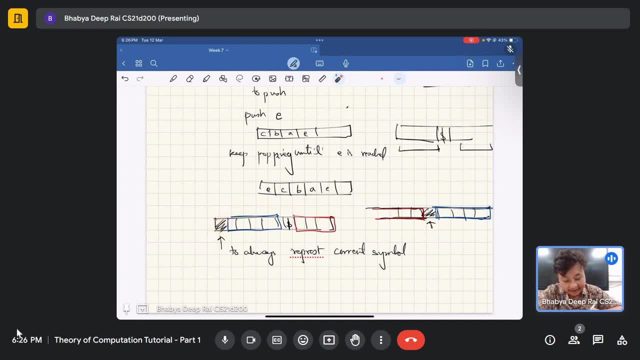 q works right. pop from the front. you are only allowed to push at the back. I'll push it at the back then. what is the new head? this is a new. now, what if the Q moves left? sorry, what? what if this head moves left? then I need to. 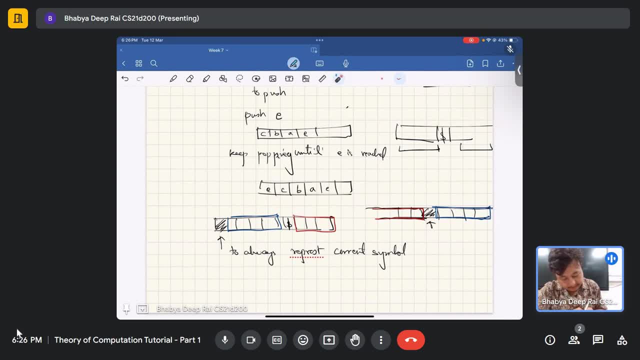 change the axis, keep, I need to keep popping, okay, and I need to get here, right. so, yeah, I need to keep popping and pushing, popping and pushing until I reach here. so first I pop this, I put it here, I pop this, I put it here, I pop this, I put it here, and I keep doing this until my front of the 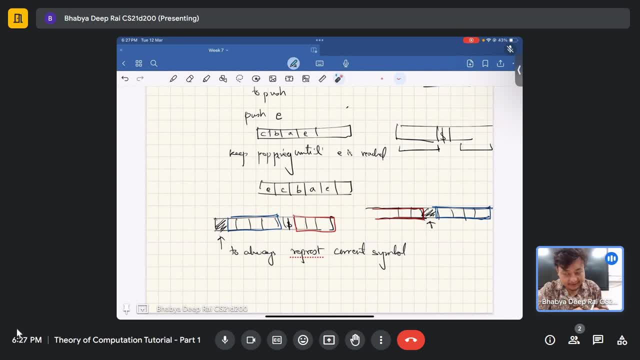 queue is this, and you can work it out yourself. you'll see that this, this dollar, still maintains the fact that, to the left of the dollar, I'll have all the elements to the to the right of the marker and this: to the right of the dollars, I have all the elements which are left. okay, so? 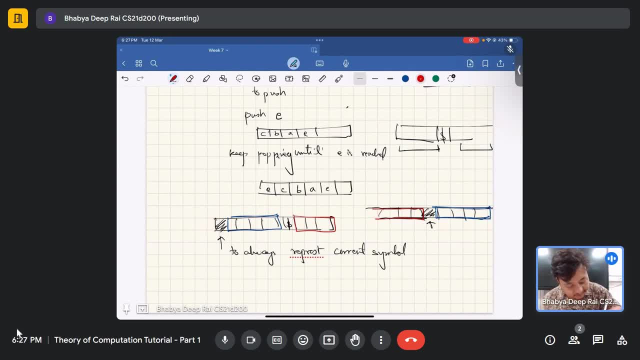 you can verify that yourself. but I'm not going that in too much there in too much. okay, so this. this is another way to show. so the answer is one, just one Q is enough to represent, or in other words, one Q is enough to represent the infinite table of a division. okay, so this. 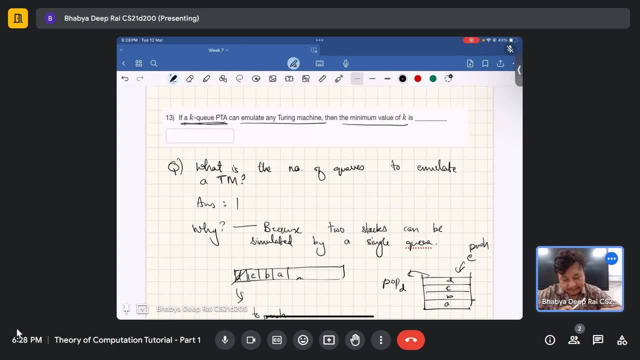 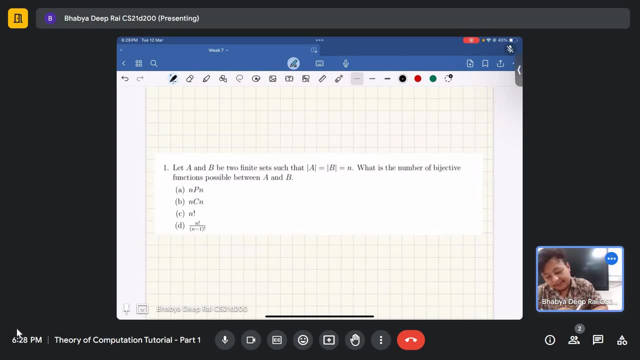 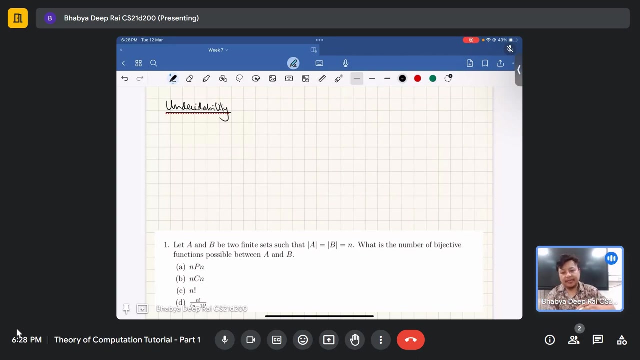 is. we will have two more questions till that time, but then tour discussion is done. yeah, those were some interesting questions based on the assignments. yeah, now we'll move on to the topic of this week. So here we'll talk about a few things. first I'll just give a small recap. okay, now there's other few. Okay, so the next week I have two problems that you might be surprised and everyone can come up with. Those are some interesting questions based on the assignments. yeah, now we'll move on to the topic of this week. elegant Messer do ell문ования. Reflective evidence to review. 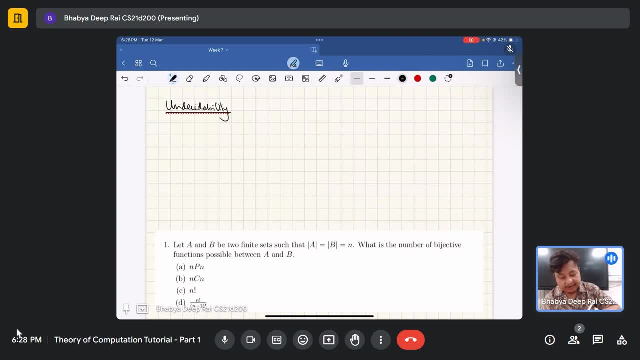 tagging students filled with tele idea. okay, undecided, no anxiety, Dolly Mudd will talk about aside More and talk about schöne Packer. So what is a decidable language? A decidable language is a language that has a Turing machine, which always halts. 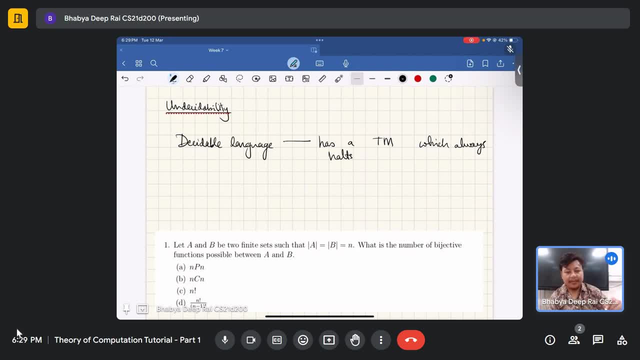 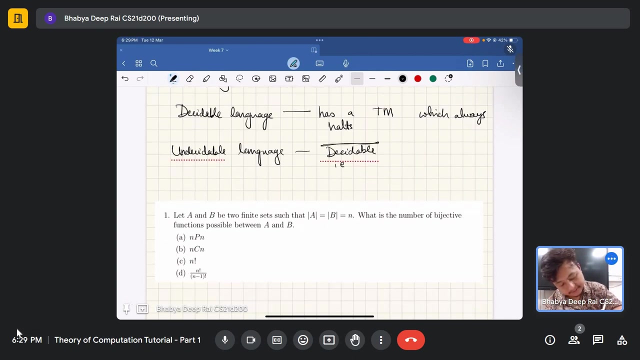 A Turing machine that solves the language will always halt and give the correct answer. Now, what is an undecidable language? Undecidable language is the complement of decidable. Undecidable language is a decidable complement. So that is Turing machine does not always halt. 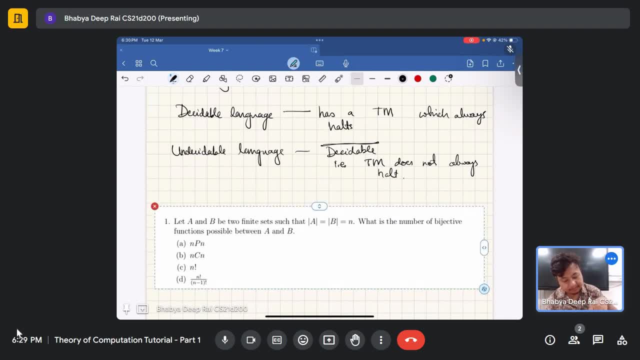 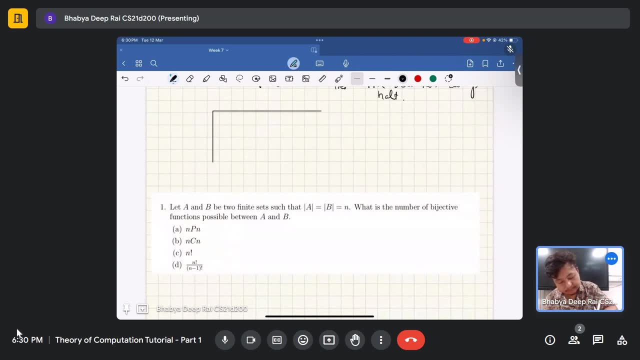 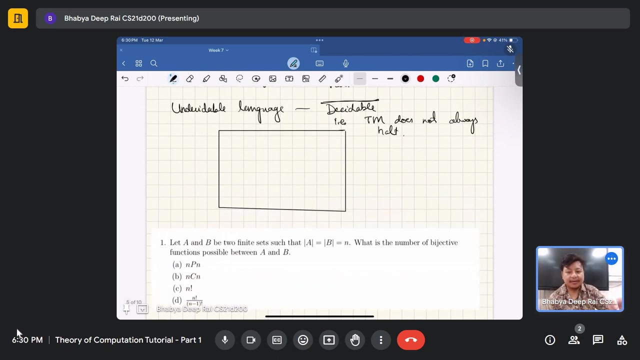 So let's make a Venn Diagram for it. So let's make a Venn Diagram for it. This is a simple cookbook, So you have the following. So you have the following: The set of all languages, also shown by par set of sigma star. 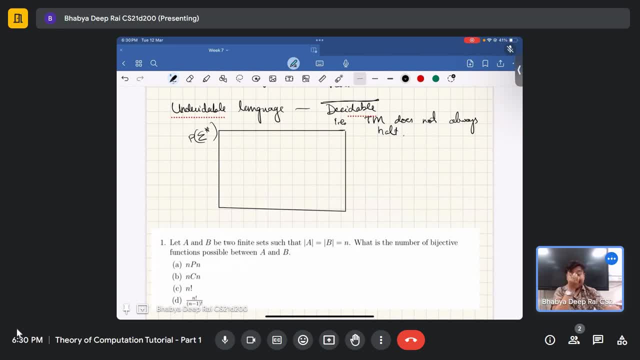 Why? Because any language is a subset of sigma star. So the set of all languages is the set of all subsets of sigma star. So what is the set of all subsets of sigma star? It is par set of sigma star. So you have decidables here, which is shown by D. 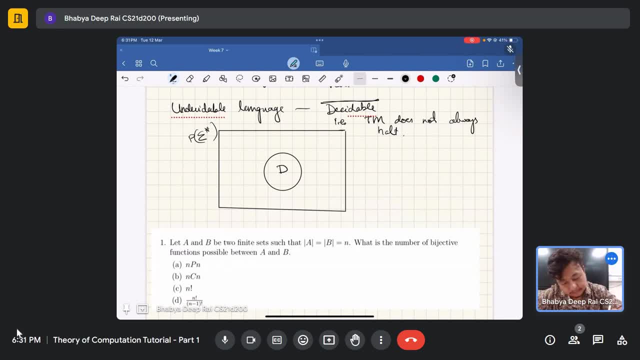 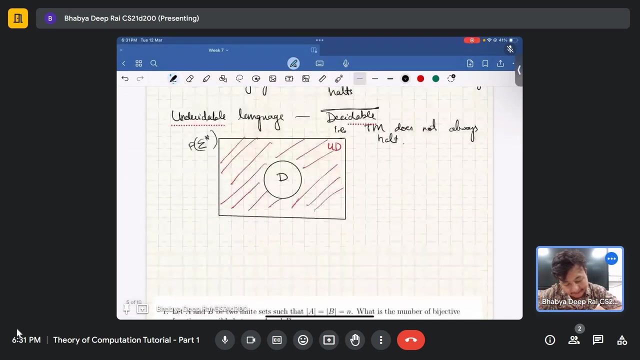 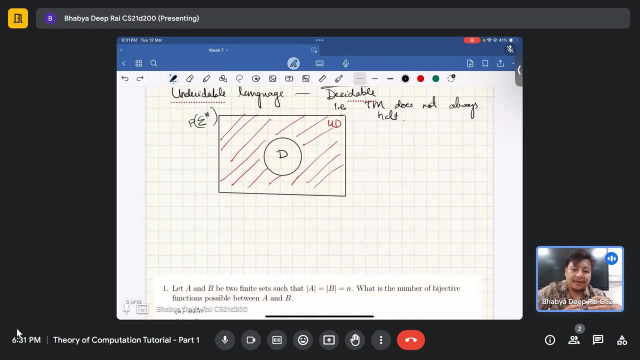 Okay, And everything outside D is undecidable. Okay, Now the question. what we want to explore is, at least in the first few lectures: is this area outside decidable? What does it look like? Well, it turns out that there are, you know, levels of difficulty even for undecidable. 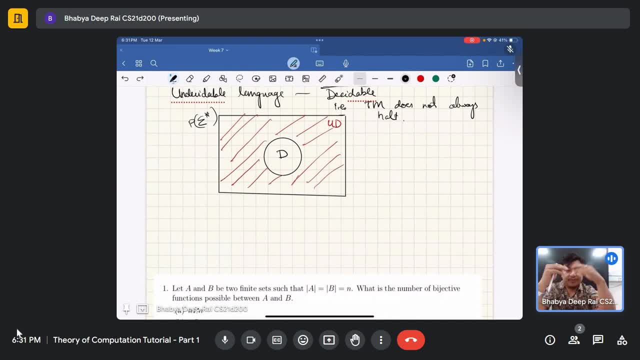 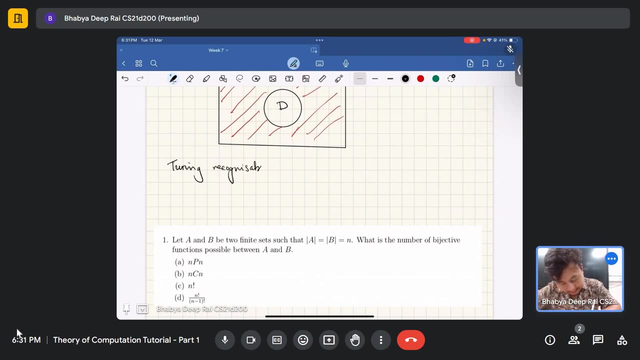 So undecidable languages means very difficult problems because you don't have Turing machine for it. But even they have different levels of difficulty. The first one is Turing recognizable. So that means in other words, the Turing machine recognizes the language. 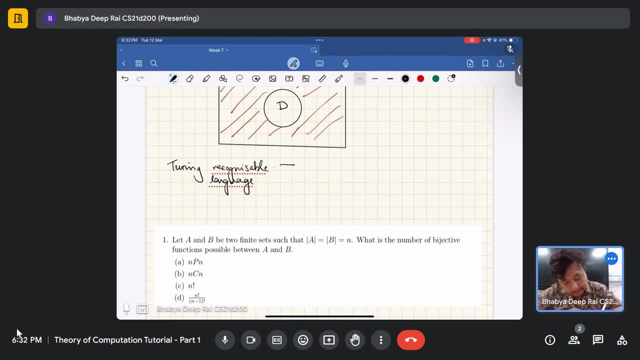 Okay. So what is meant by Turing recognizable language Turing machine? there is a Turing machine for the language that always holds in the yes case, So a Turing machine in a decision problem that says yes or no. Okay, Testing for this language at least, it is always whether something is in there in the language or not. 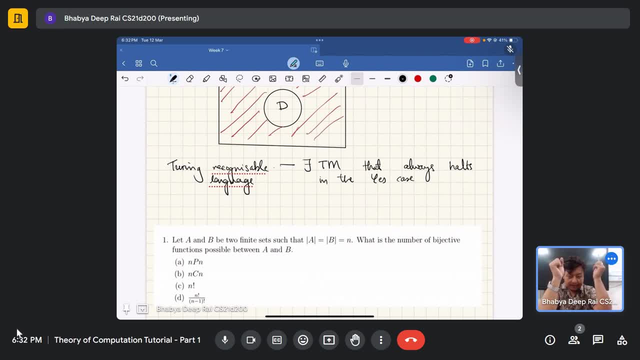 So if the string to be tested is there in the language, it will always say yes. The machine will always hold and say yes. But if it so happens that the string is not in the language, then it may not always hold. 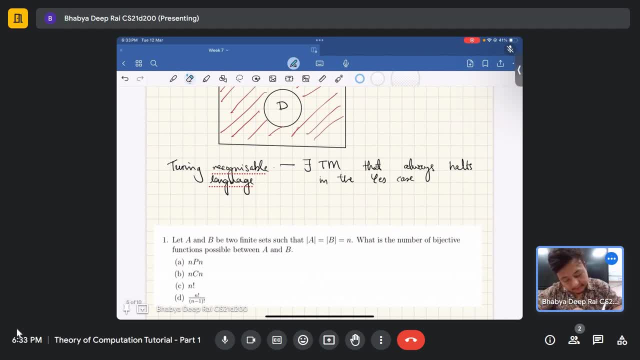 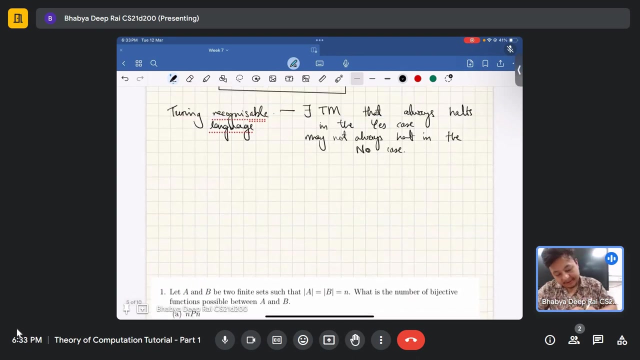 It may loop, also May not always hold in the no case Right. For example, I think there was a problem that said about polynomial, talked about polynomials, So question is: does a polynomial have integer roots, always or not? Okay, 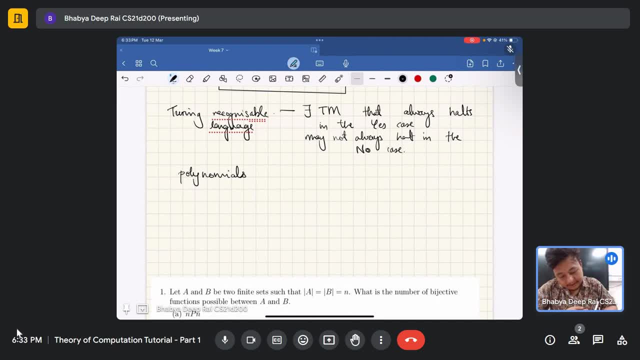 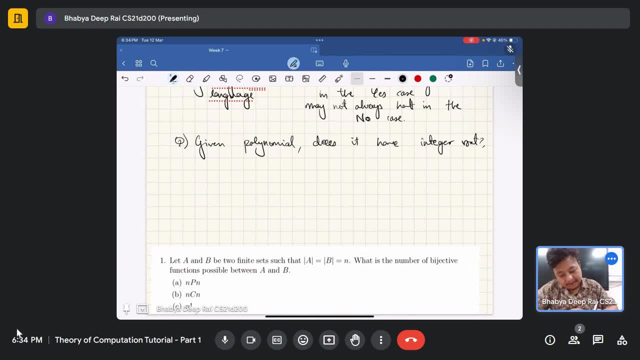 Well, I can well, if it does have integer roots, what I will do, okay. So, for example, x square plus 2x minus 1 equals zero. this is a polynomial l, So is this in the language. 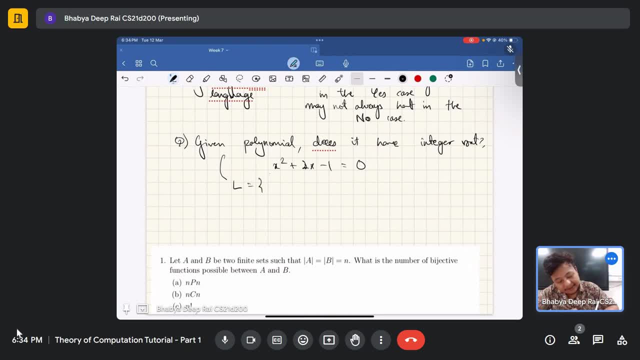 The language is what is the language? L is p such that p is a polynomial. So this is什麼? So with integer roots? This is an equivalent way to formulate it. Now the question we ask is: given a polynomial, does it have integer roots? So can we build a Turing machine to? 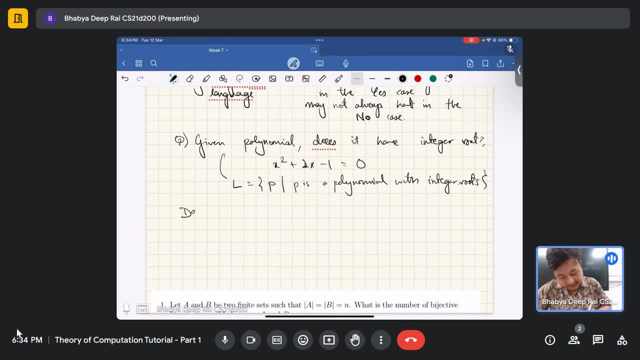 decide it. Well, if I have a following Turing machine, okay, and input is called P, let's say okay. So I go over. you know, 0, 1, minus 1, 2, minus 2, 3, minus 3, 4, minus 4, and so on. 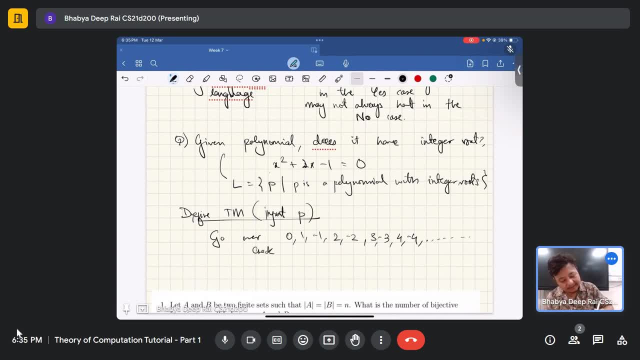 Go over each of them And check. go over, let's say, x equals, and check if P of y- sorry, P of x- is equal to 0 or not. If yes, then that particular value is a root. So say yes and hold. This is what my 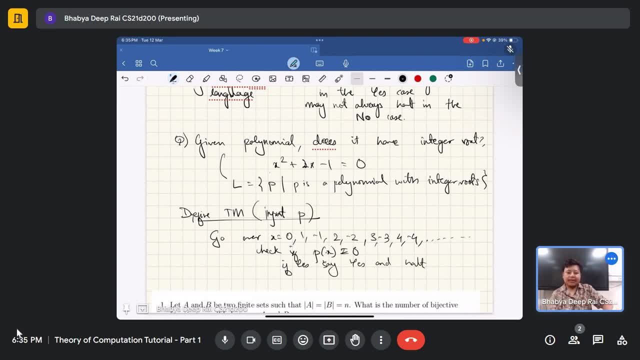 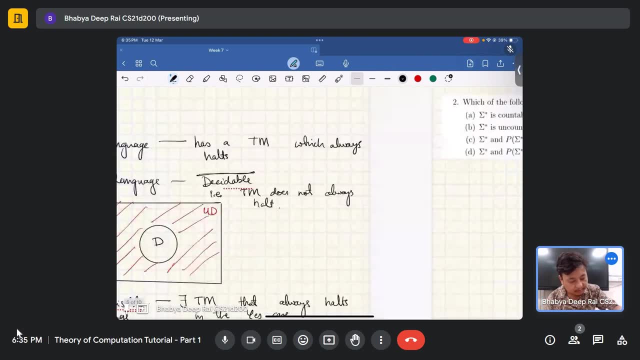 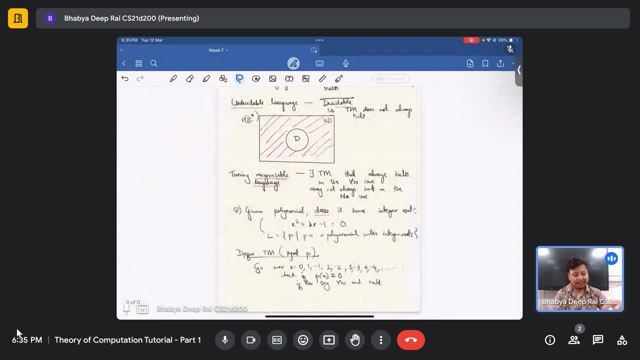 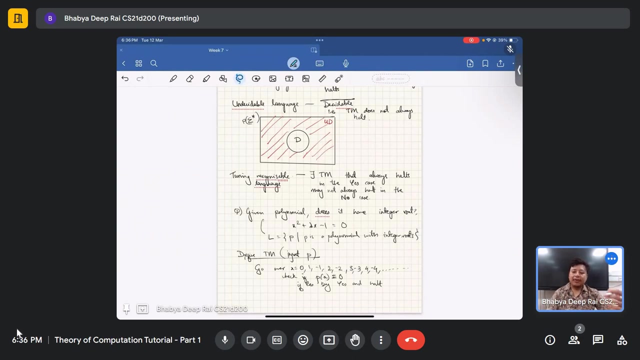 Turing machine can do, Otherwise what it will do? it will just keep looking for it. no, So so it will just keep looking for it and it will never end. If, let's say, the polynomial did not have integer roots, we are just looking over all. 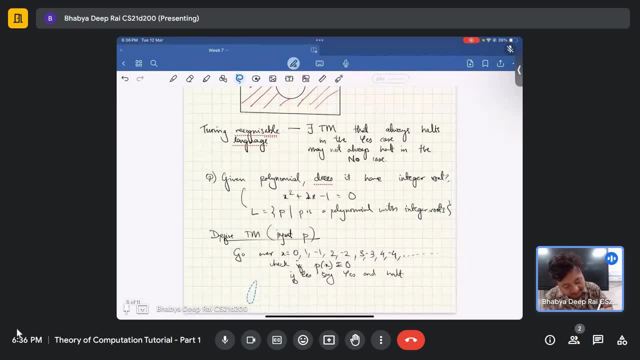 possible integers? no, So this is an example. but what if? so, it will never find it. But but take into account the fact that if the integer existed, we will always sooner or later encounter it and then make the polynomial evaluate to 0, and then say yes and hold. So that means that if 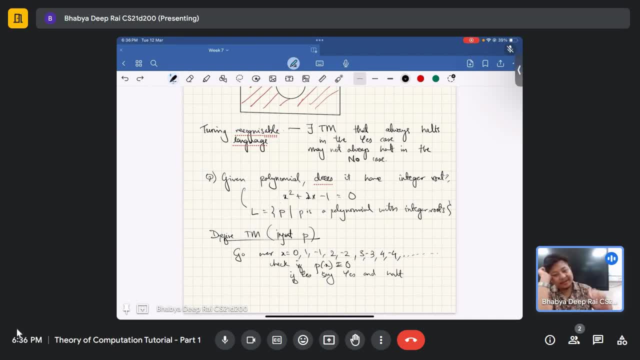 the given polynomial definitely has integer roots. the Turing machine will always say yes and hold, But in the no case it is not halting. So it is a Turing recognisable. So it is a Turing recognisable. So this means L is Turing recognisable. Now another fact is: any decidable language is Turing recognisable. 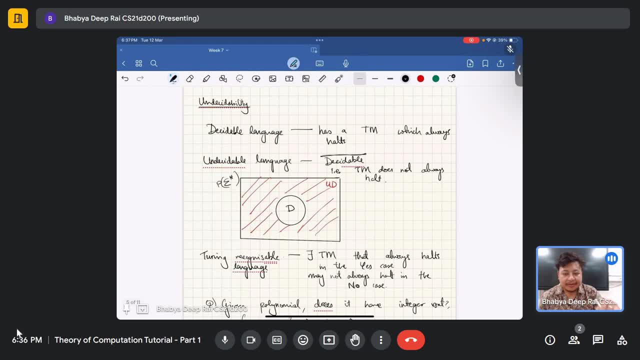 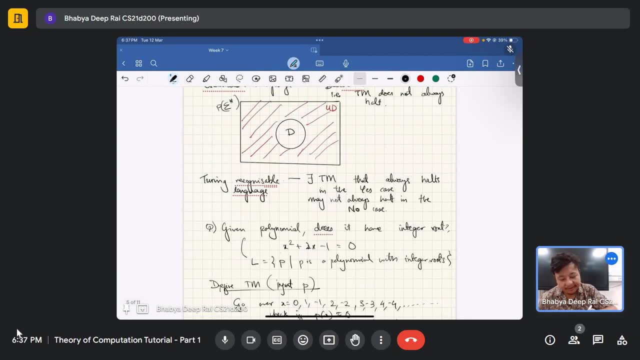 Right. Any decidable language is Turing recognisable, because a Turing recognisable means it also it calls in both the cases yes and no. But Turing recognisable means that it may not. it may not halt in the no case. but even if it halts in the no case, it's not a problem. 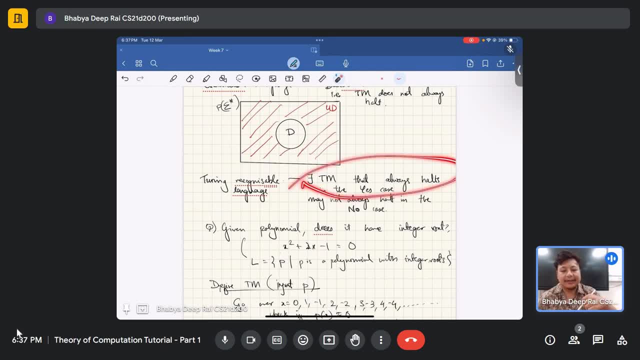 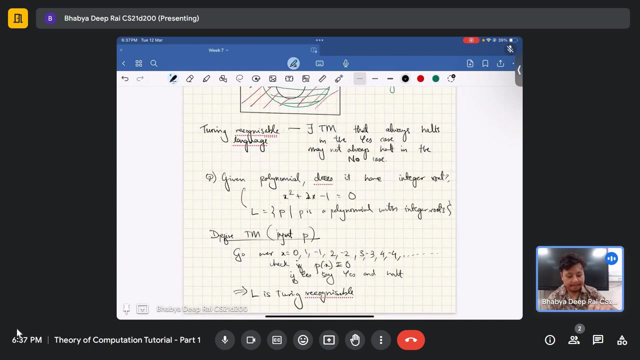 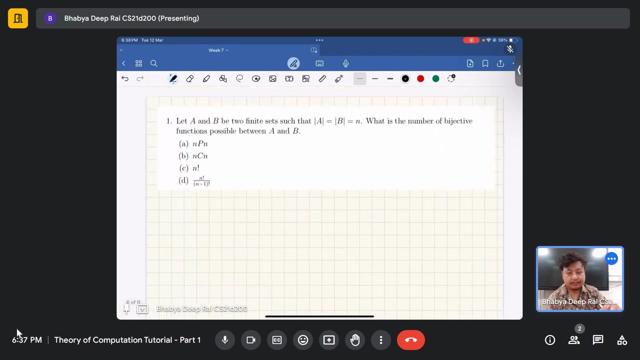 it's still Turing recognizable as long as it halts in the yes case. So therefore, all decidable languages are Turing recognizable. Okay, so this part is focused on the study of such languages. Let's begin. Question says the following: Let A and B be two finite sets such that size of A is equal to size of B is equal to A. 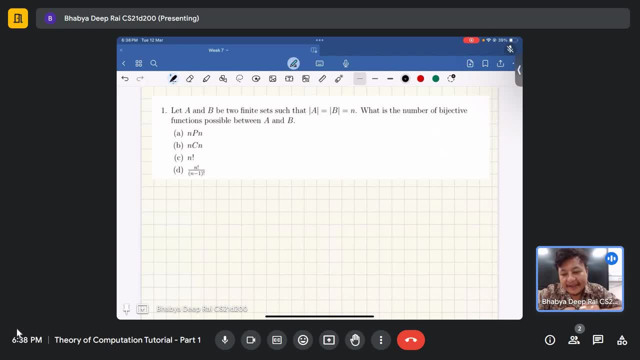 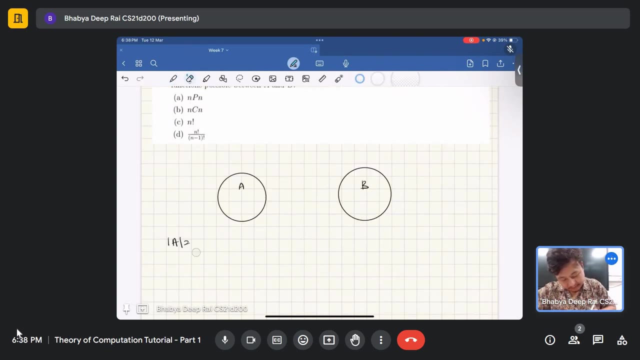 What is the number of bijective functions possible between A and B? So here they are saying there are two sets, A- both are finite- and B, so that size of A is equal to N, both the sizes are equal. Question is, what is the number of bijective functions possible between A and B? 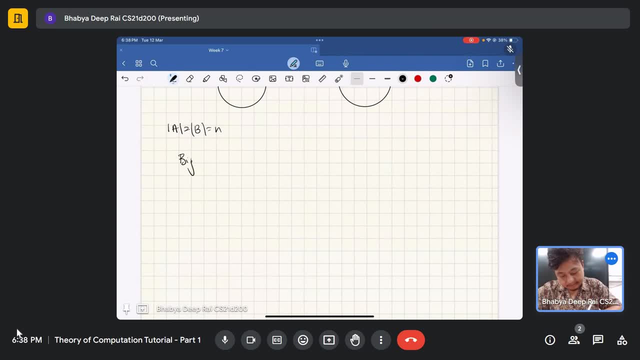 What is the bijective function? first of all, What is the number of A and B? The bijective function is both 1: 1 and 1: 2. right, Both 1: 1 and 1, 2.. So what is meant by 1: 1?? 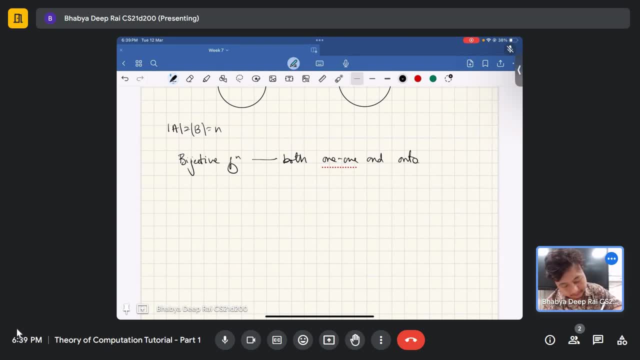 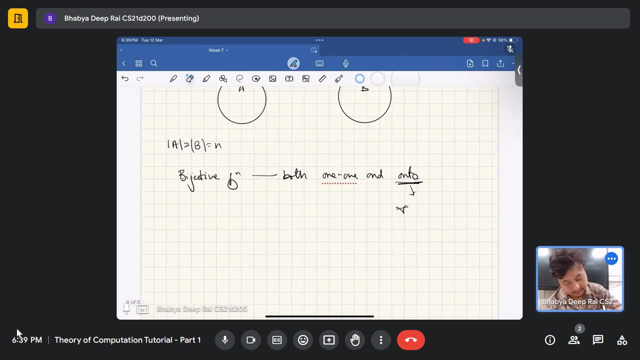 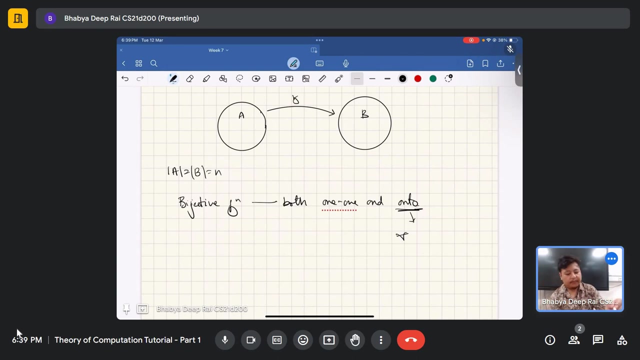 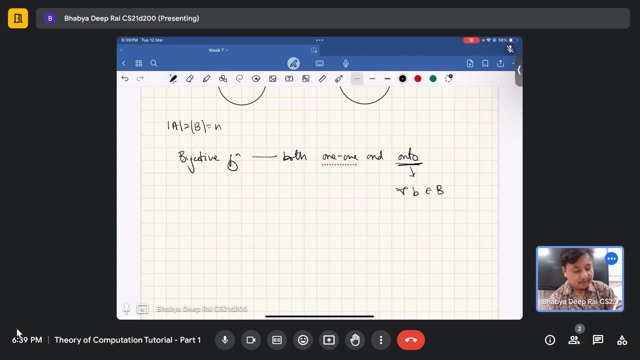 For? okay, let's do 1, 2.. WHAT IS B, WHAT IS S? WHAT IS B, WHAT IS S? first, okay, so let's face the function for all B, P and B and F- inverse of B is there in a. so for any element I take in 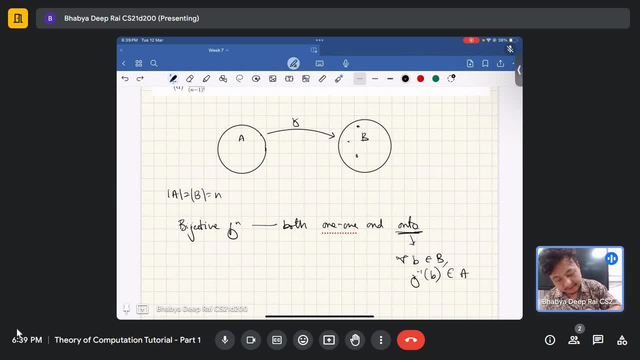 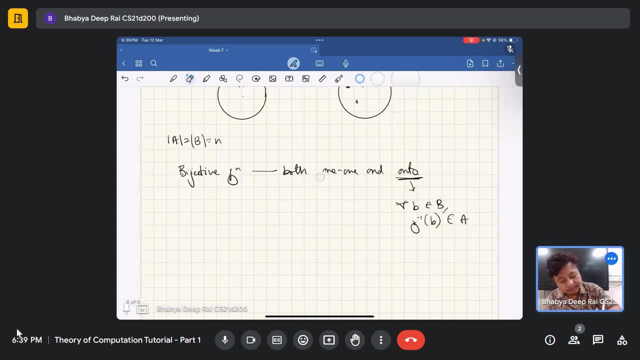 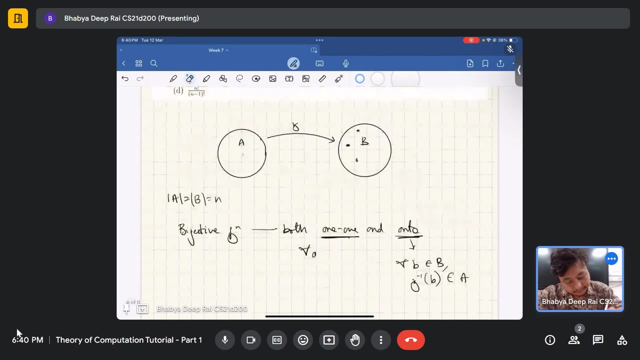 B, I will always find a corresponding some, some F, some value of a always maps to that. okay, and what is onto for all elements a in, or it's rather defined as follows: the if there are two elements, okay, they must be. if there are two elements, then 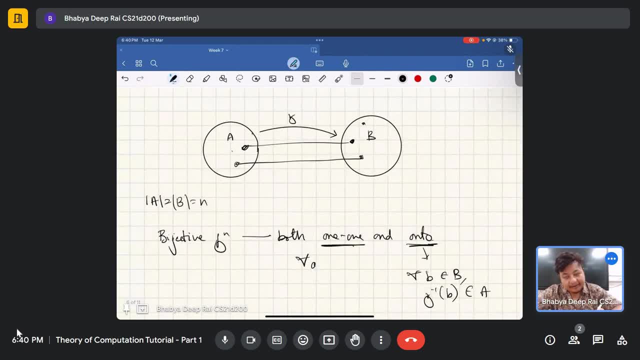 in B that are mapped from F. they must be mapped to from distinct elements. it cannot be something like this is not possible. something like this is not possible, sorry, sorry. yeah, this is not possible. this should always be possible, but take care that these kind of elements may exist. 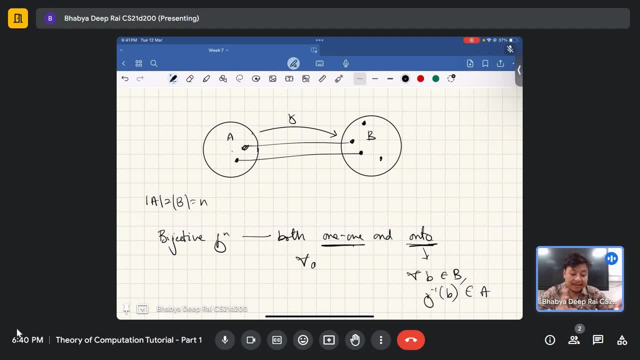 that don't get mapped do at all, but don't want to. these kind of elements cannot exist. they should be. there should be some kind of element that is getting mapped together, okay. so, like I said, something like this is not, though, so for all: a 1, a 2 and so on. 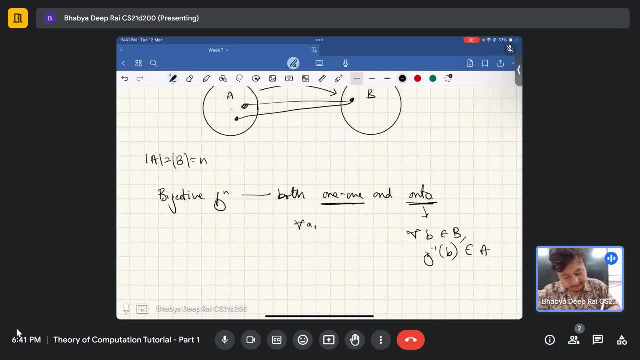 so if for all, so if so for all. a one A, 2 innumerable elements is few things not available in the Noel field. so if there is such a thing that that is getting mapped to, that all elements dense, there is. no, it is not any map. 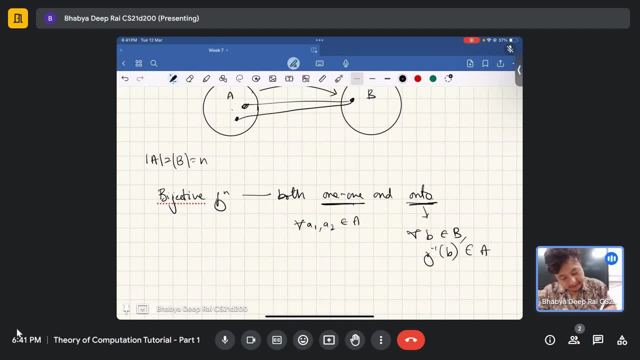 But Doling Onto giving k material절 a2 in a, if f of a is equal to f of a1, is equal to f of a2, then it must be that a1 was equal to a2.. It cannot be that they are separate. yeah, it cannot be that there are two separate. 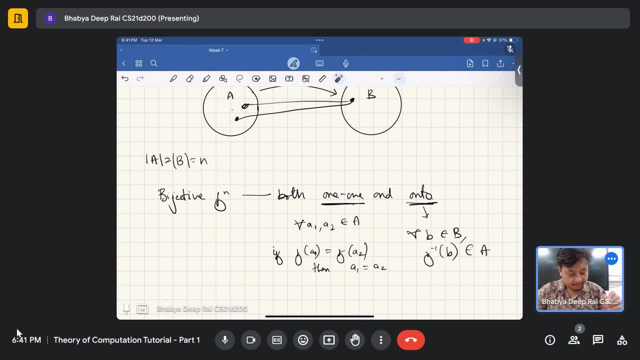 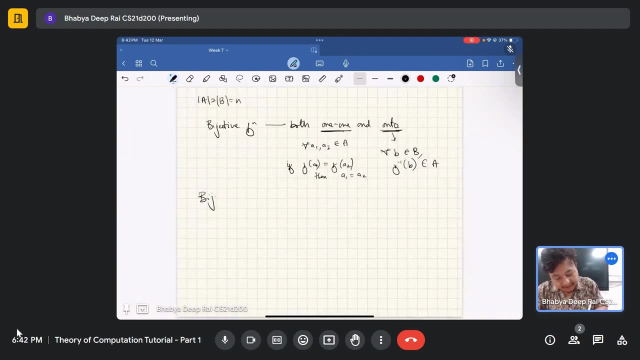 elements in a that are mapping to the same element in a. Now, what does a bijection look like? Now, what does a bijection look like? Bijection is both 1: 1 and 1: 2.. Now, because it is 1: 1,. 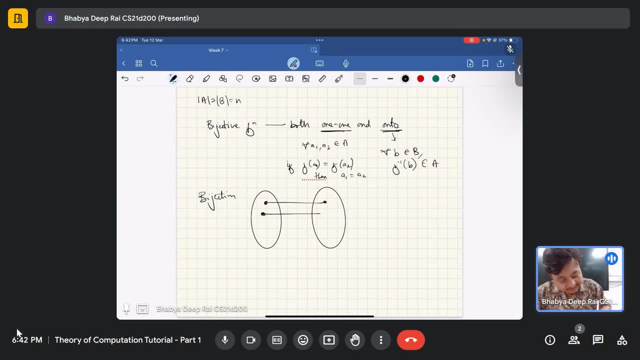 because it is 1: 1, one element gets mapped to one element, one element gets mapped to one element, and so on. something like this cannot occur, Because it is onto. it should be mapped by some element and it cannot be mapped by this guy. 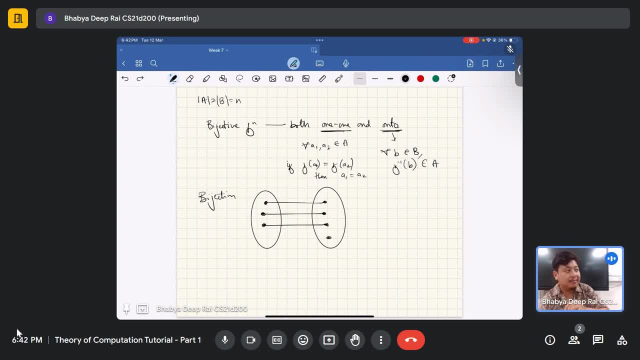 because it is a function. it is contradicting the meaning of the function, So it can only be that there is an element here. So this is what a bijection will look like: Every element on b side is covered by the function, and every element in b side is covered by distinct. 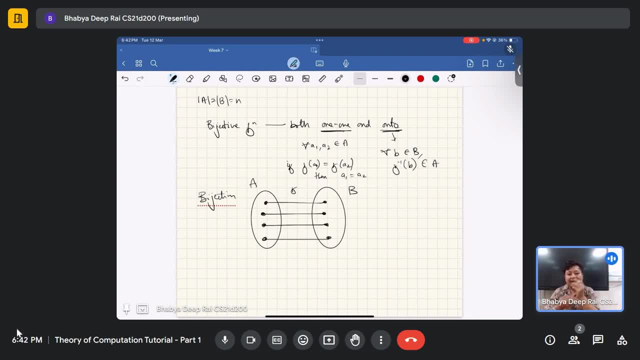 element. This is what a bijection looks like. Why is a bijection important? Bijection showing bijection between two sets shows that their sizes or their cardinalities are same. Getting it If there is a set A, there is a set B and there is some kind of bijection. 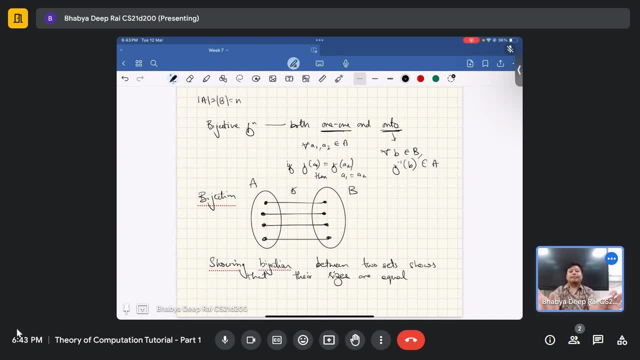 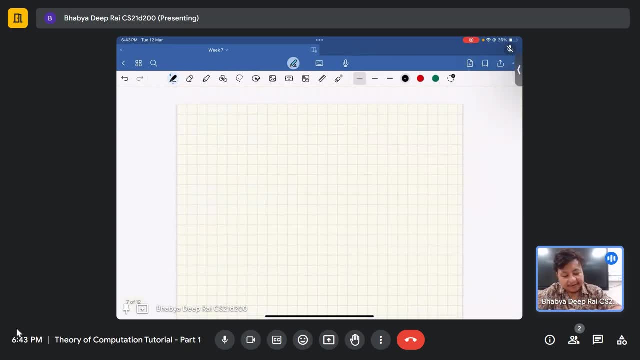 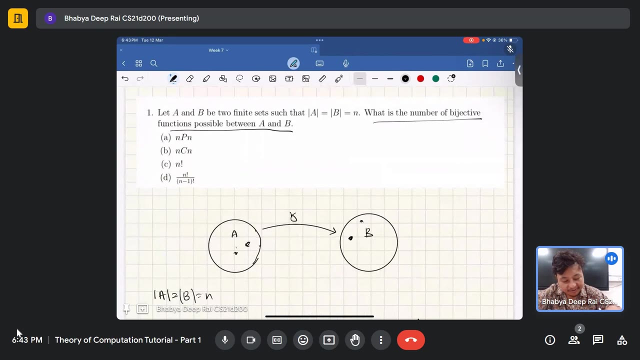 if I can show a bijection, then it means that their sizes are same. So this is a very common tool in discrete maths, in mathematics in general. So they say how many number of bijection possible between A and B. So this is a simple. 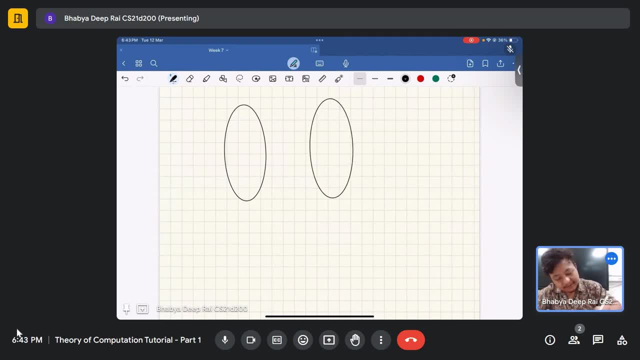 combinatorial question. So if I have A and I have B and I take this and now I want to count, I have element 1,, I have element 2, 3 and so on. I will just number them randomly So one can be mapped to some element. 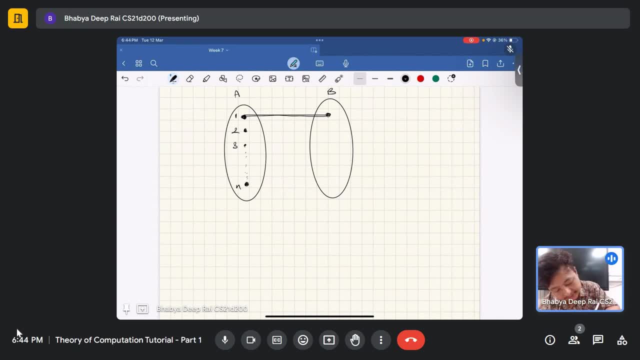 in B Or- and I will call this A1, A2, A3, A. So I will call this B1, B2, B3, B4 and so on till Bn. since both are same size, Then A can map to B1, or A can go to B2, or A can go to B3,. 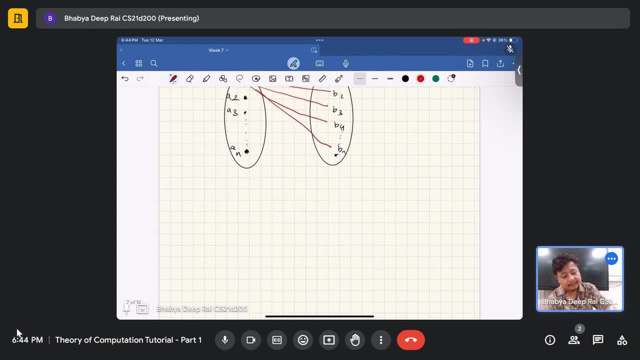 A can go to B4 and so on till Bn. So it is number of bijections. Number of bijective functions is nothing but the number of choices for F of A1 plus number of choices for F of A2 plus, and so on till F of A2.. 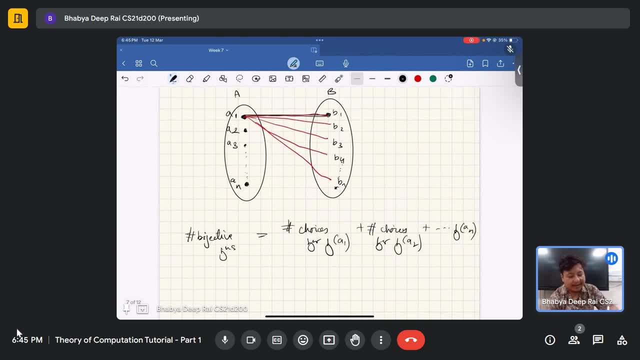 So how many choices for f of a? There are n elements here, So there are n choices. How many choices for a2? Now, let's say a chose something. Let's say a chose this guy. How many remaining are there? There are n minus 1 remaining. So how many choices for? 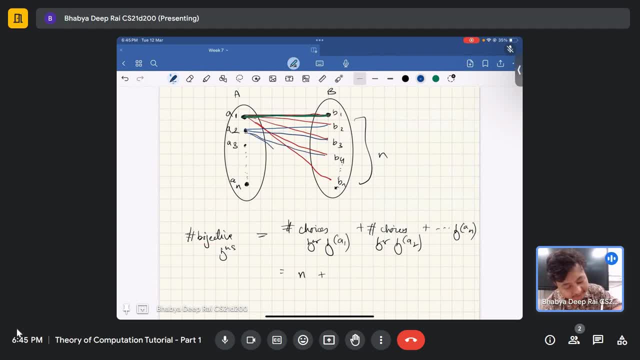 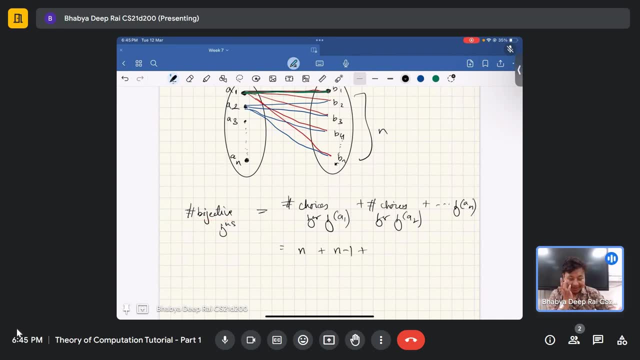 a2?? a must choose from the remaining n n minus 1.. Now, similarly, how many for a3?? it must choose from the remaining n minus 2.. This is not plus, this is multiply, because it is an and case a has n many choices. 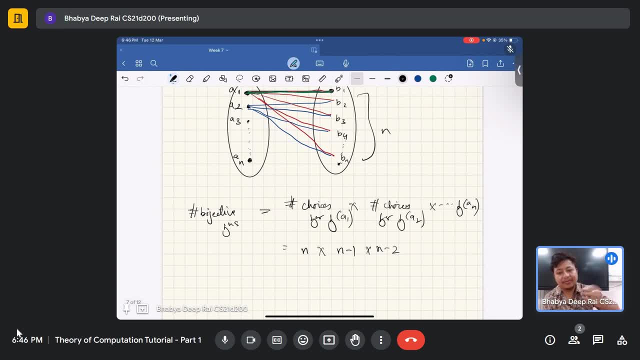 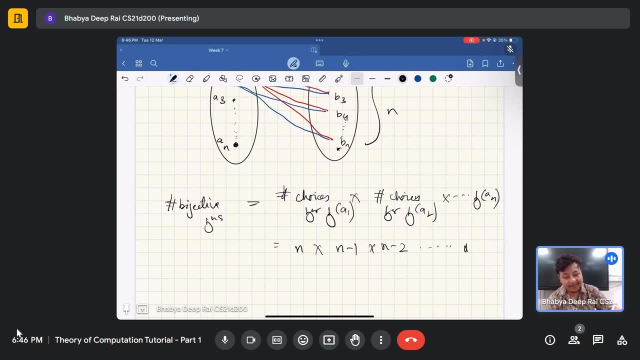 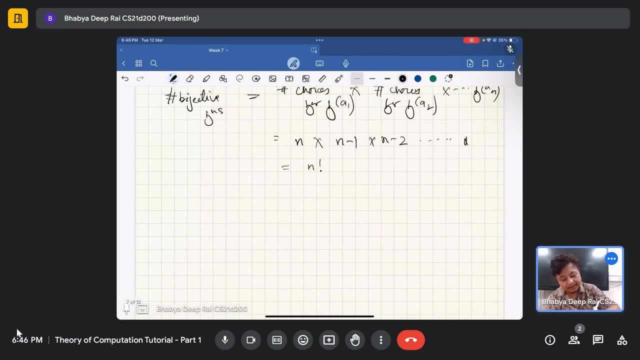 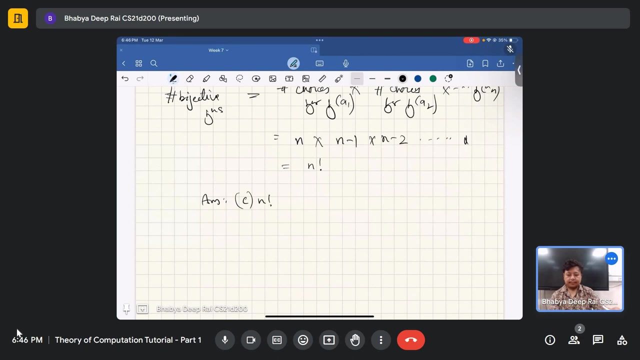 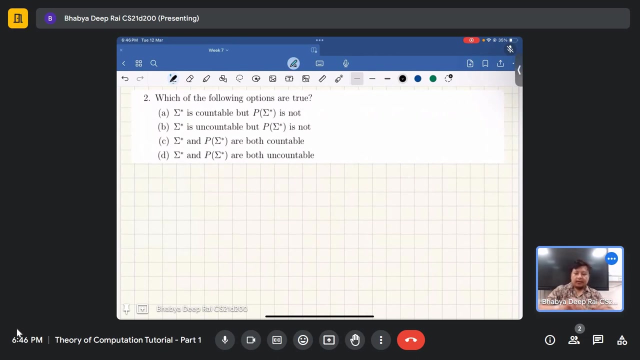 and b makes n-1 many choices, a2 makes n-1 many choices, and so on, and so on, until there is only one choice remaining, and this is nothing but n? factorial. So what is the answer? c- n factorial. Another question based on accountability. now, Which of the following options are true? 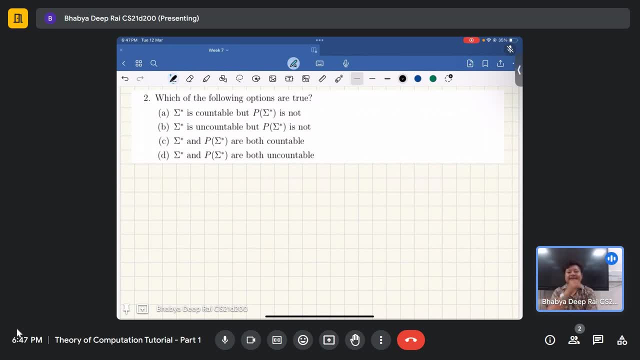 Okay, Sigma star is countable, but power set of sigma star is not. Sigma star is uncountable, but power set of sigma star is not. Sigma star and power set of sigma star- both are countable. Sigma star and power set of sigma star are both uncountable. Firstly, anything that is 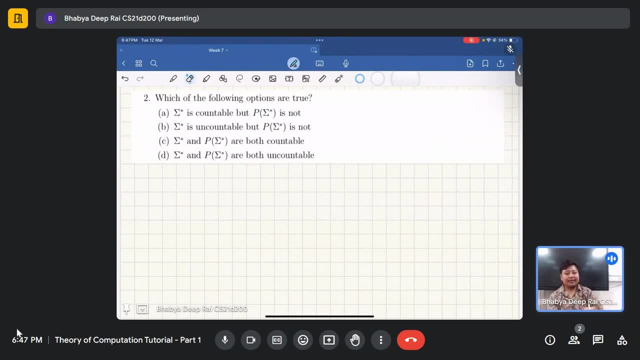 countable can be listed. Okay, All elements can be listed in some particular order, such that every element in the set appears in the list. Okay, Any countable set can be listed so that every element can be listed. Okay, Any countable set can be listed so that every element can be listed. 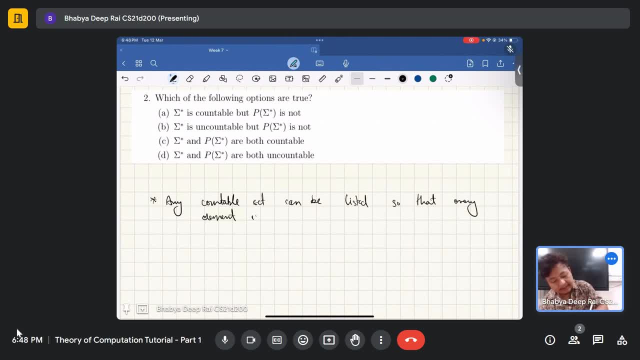 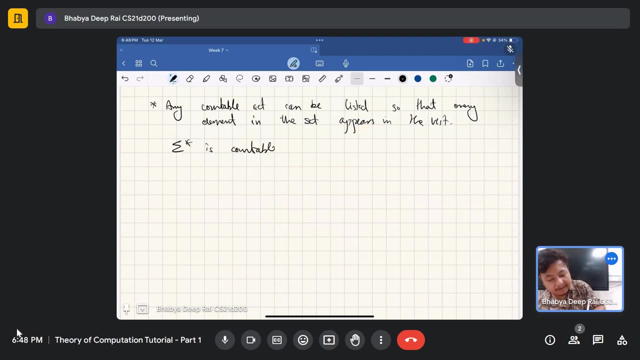 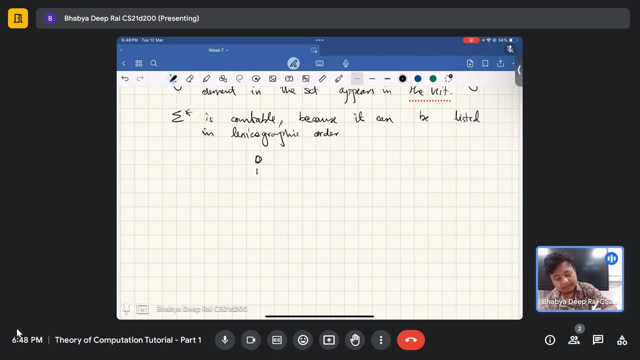 Okay, In the set appears in the list, Sigma star is countable. Why? because I can list it. It can be listed in what order? In lexicographic order: how well, first I do a 0, then I do a 1, then I do a 0, 0, then I. 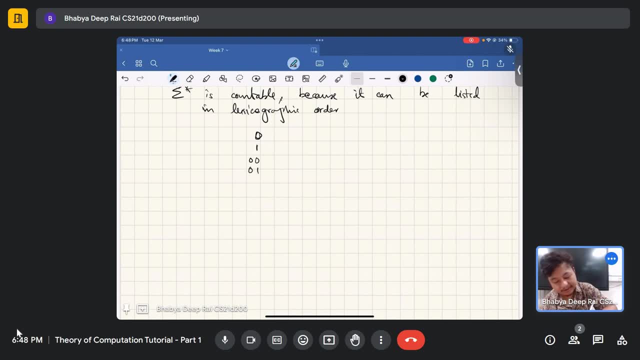 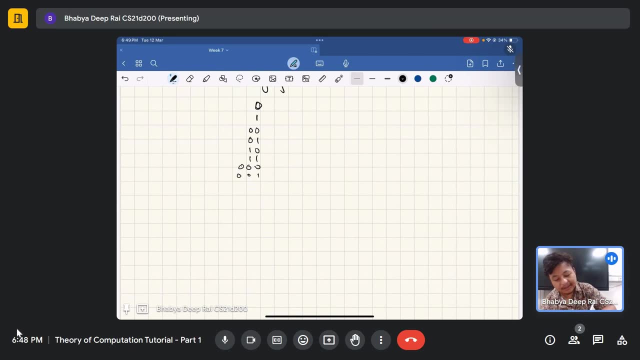 do a 0- 1, then I do a 1- 0, then I do a 1- 1, then I do a 0, 0, 0, 0, 0, 1, and so can be listed out in this, and this is the normal lexicographic order. the rule is just as the next person. 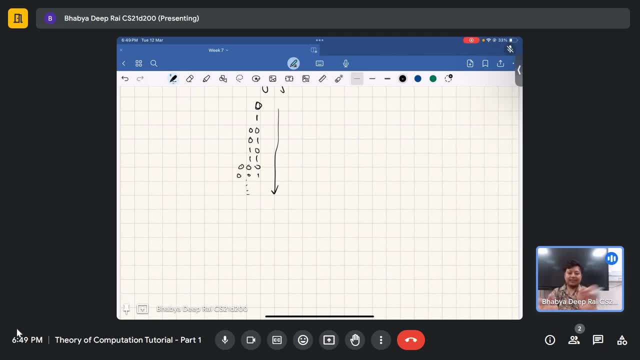 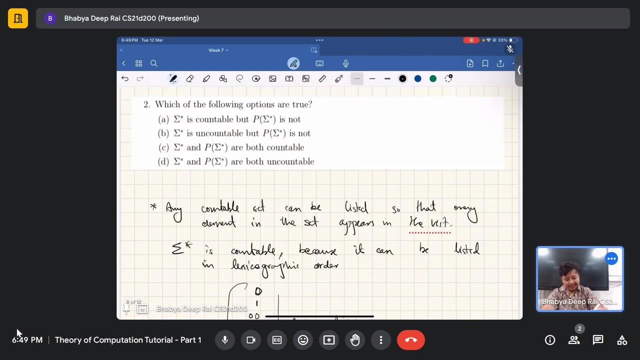 in the element is always lesser in comparison to the previous person. so lexicographic order and every string is guaranteed to appear here, every binary string. so this is nothing but Sigma star, so this is countable. now the question is saying either A is true or B is. 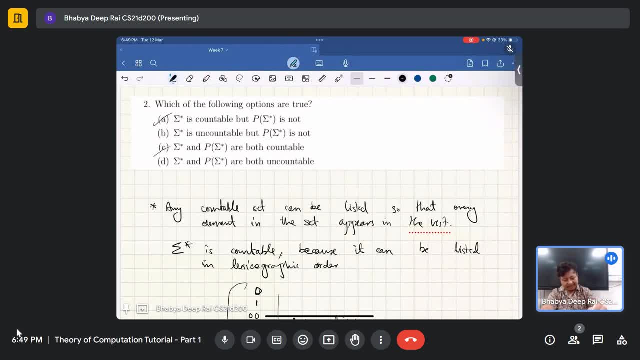 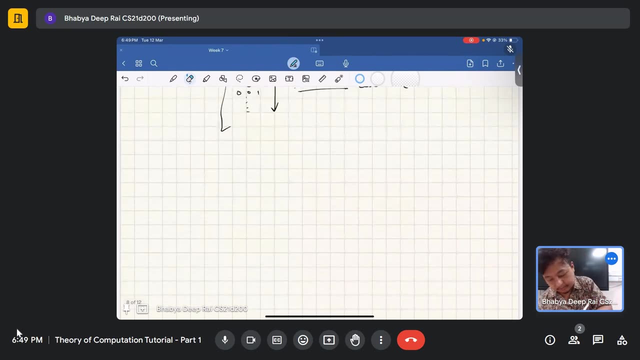 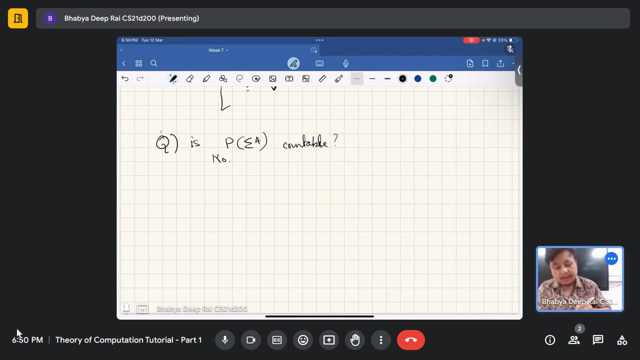 true, right, Sigma star is countable, but power set is not, and Sigma star is and power set. both are countable. so now the question is: is the power set countable? okay, okay again, the answer is no. a power set of an infinite is never countable, even if that particular set used to be countable. Why? Because of Cantor's. 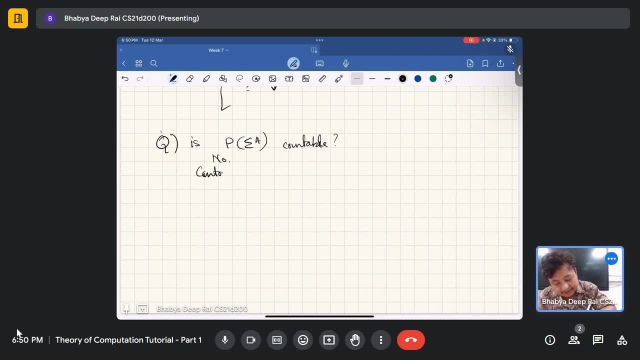 In the lectures we saw Cantor's argument. Cantor's argument, Cantor's theorem, let's call it- shows there does not exist a bisection between set A, an infinite size set A and power set of A. If you want to recall how he did it? 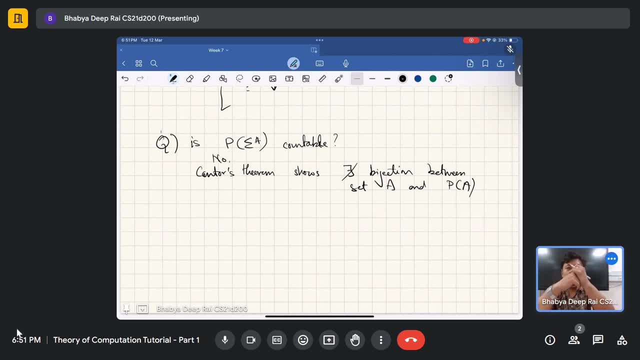 or, if you want to recall the proof for the real numbers and natural numbers, real numbers versus natural numbers. we listed out all the real numbers and then found the diagonal. We took the diagonal and then flipped it each so that it does not exist. 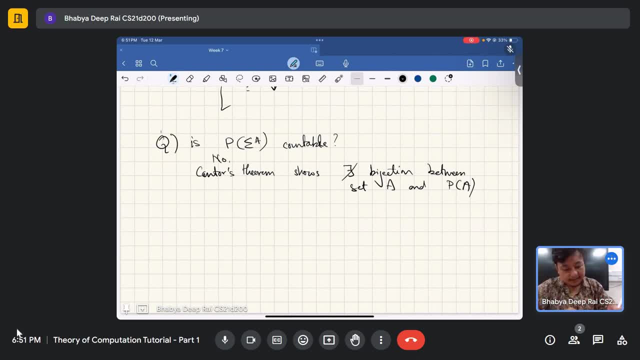 We can do a very similar thing for the power set also Right. so what we do is we take what is called the characteristic string. So, although this is not real, it is not really required, but any, let's say, B is a subset of A. 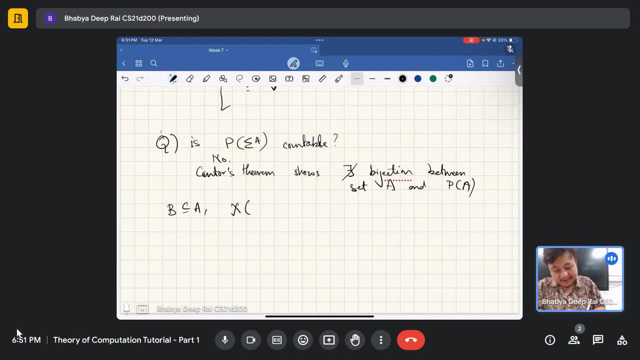 then what I can do is this characteristic, represented by chi: B is a string which consists of string B1,, B2 and so on, Where B I equals one if, and only if, the ith element is in A. Okay, and this I'll leave as let as an exercise to you guys, but show that the diagonalization 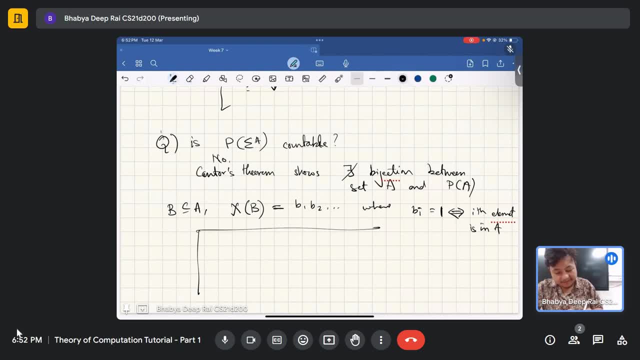 shows that if I take different choices of B, okay and uh, B can be taken as 0..0..0., 1..1.. sting also, and this is another choice, to B0..1..0.. take care that this is infinite, because A is an. 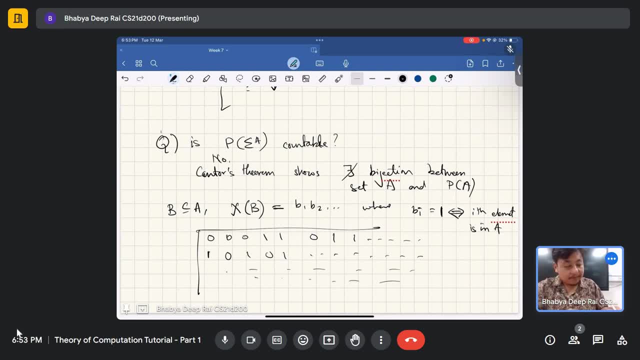 infinite set. the subset, like the string length, is also different and show that the diagonalization would imply that our bijection is not not null, wat diagonalization would imply that our bijection is not possible. But what is this? If I take all of these strings, what is this? This is nothing but the power set of A. I mean they. 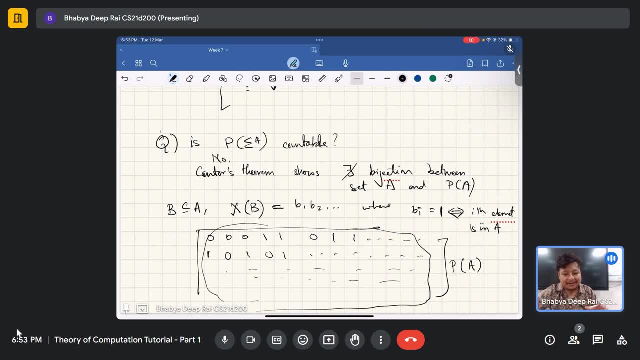 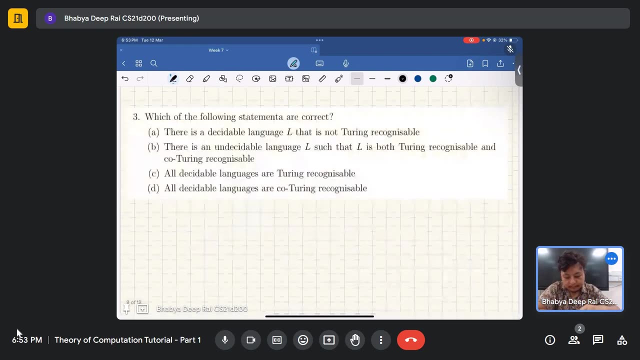 are represented as strings, but as sets they are still the power set of As sets together. if we collect them, all of them, then they are just subsets of A. So together we collect them, they form the power set of A. So here is the question on decidability: Which of 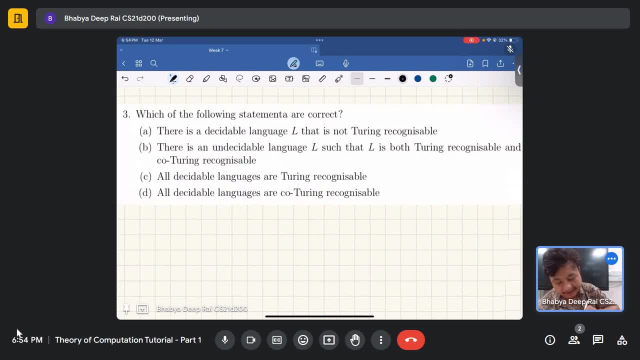 the following statements are correct: There is a decidable language- L- that is not Turing-recognizable. There is an undecidable language, L, such that L is both Turing-recognizable and coturing-recognizable. All decidable languages are Turing-recognizable. All decidable languages. 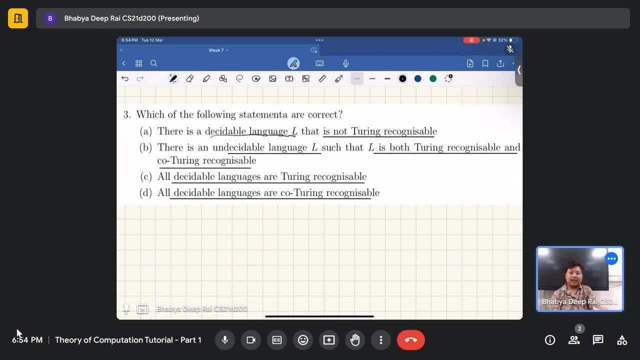 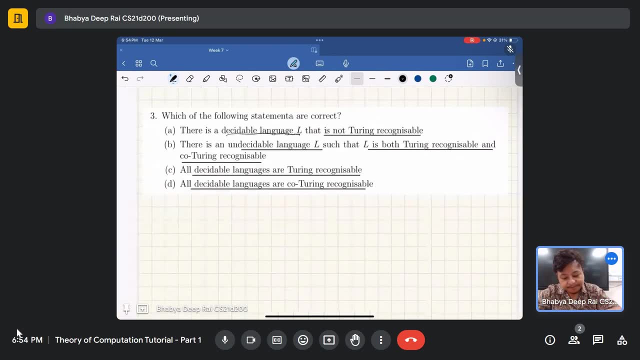 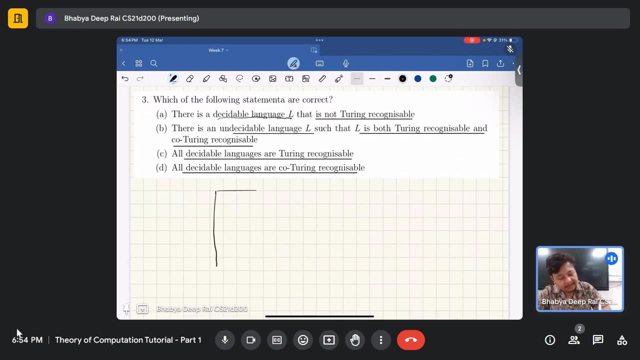 are coturing-recognizable. These are the questions. Ok, Now let's recall this: both Turing-recognizable- oh sorry, Turing-recognizable- and decidable. So the first option we have to, okay, and this is, uh, this, this part. 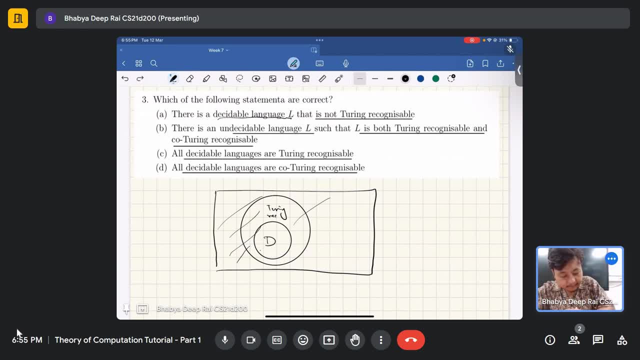 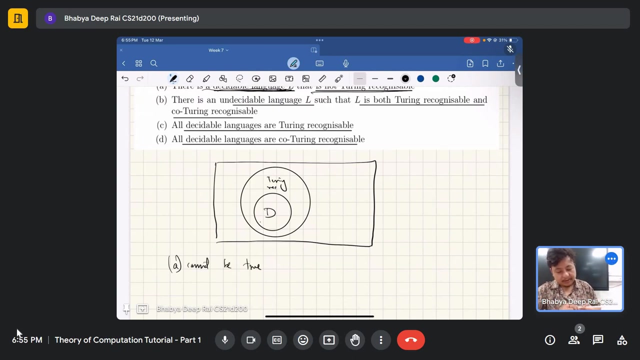 is undecidable. okay, everything outside decidable is undecided. so they are saying there is a decidable language, l, that is not turing recognizable, but turing uh. decidable d is inside turing recognizable, right? so it cannot be the case, so a cannot be true. next, it's saying 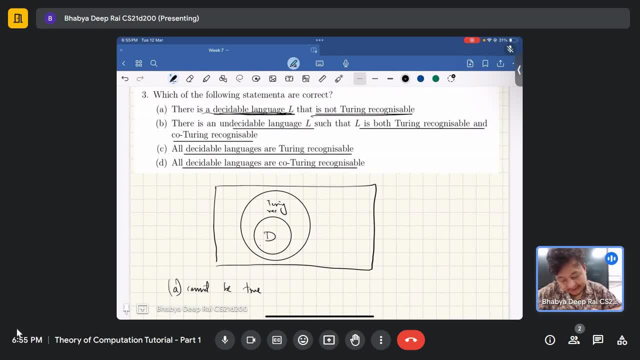 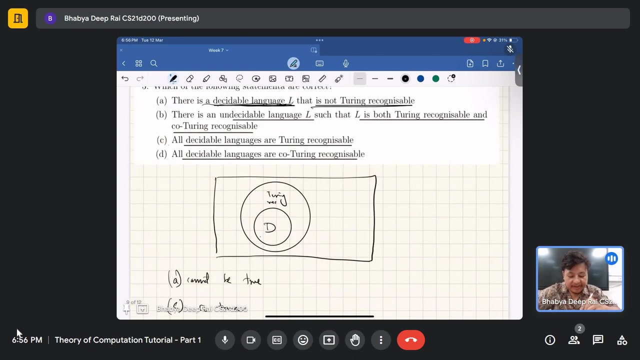 okay, i will come to b. um, let's look at c. all decidable languages are turing recognizable. all decidable languages are turing recognizable, and that is evident from this venn diagram. any decidable language is inside turing, so c is true. now, before we look at b and d, we'll look at what is called code turing. 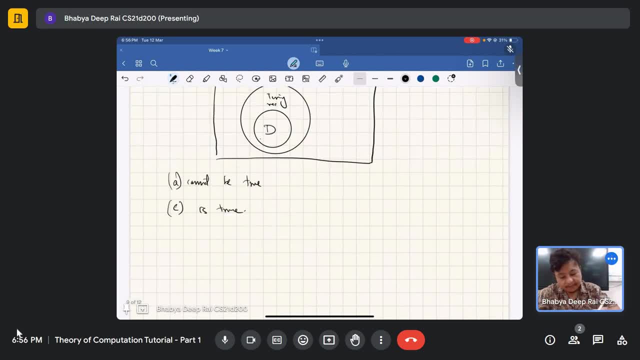 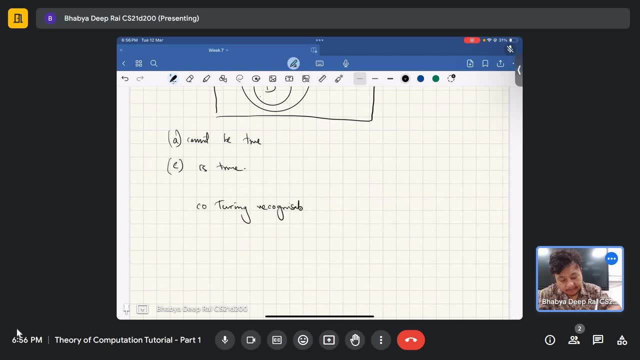 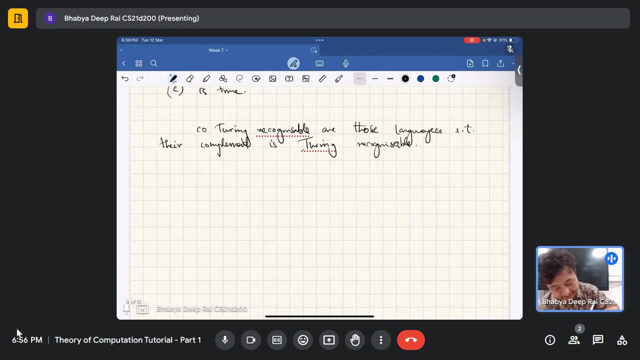 recognizable. okay, code turing. recognizable languages are those languages such that cotorina. those are such that their complement is turing recognizable. that addends the name. you may have seen it in the lectures, also in the lectures. okay, i'm not going to tell why. in the lectures, uh, it said that turing recognizable. 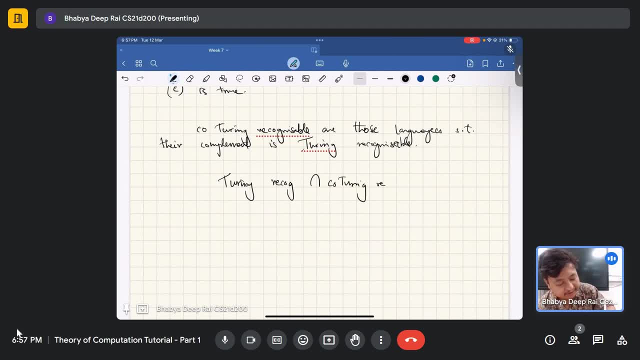 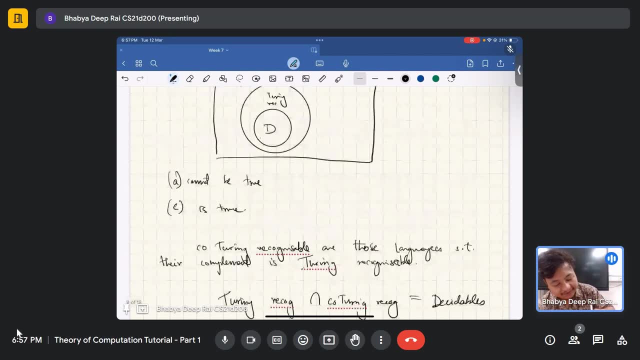 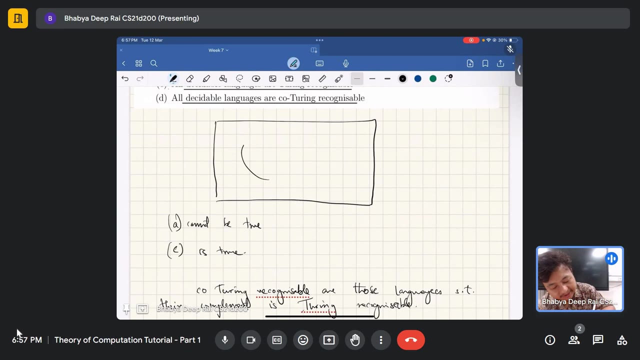 intersection, code turing recognizable is exactly exactly what the decideables so, in fact, the picture looks more red. it's not just that these contain inside turing recognizable, but including the fact that d is an intersection of the touring recognizable and code turing recognisable. okay, now it says there is an undecidable. 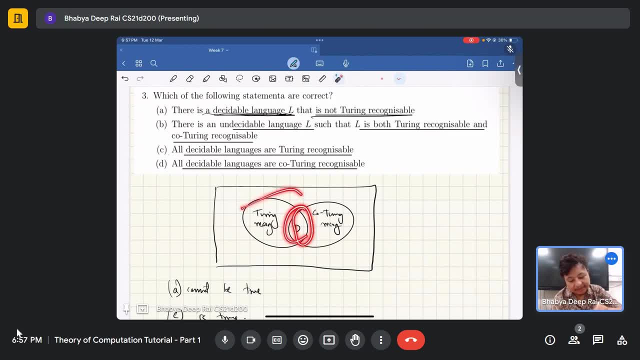 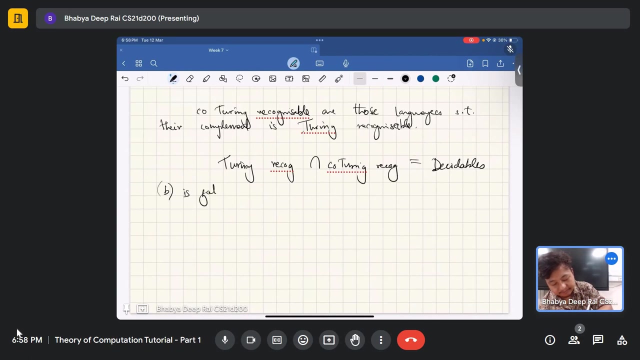 language l. undecidable meaning outside. decidable, which means everything, which means everything here is undecidable. undecidable language l says that l is both turing recognisable and code turing recognisable. that cannot happen. b is false. why, if there is an undecidable, 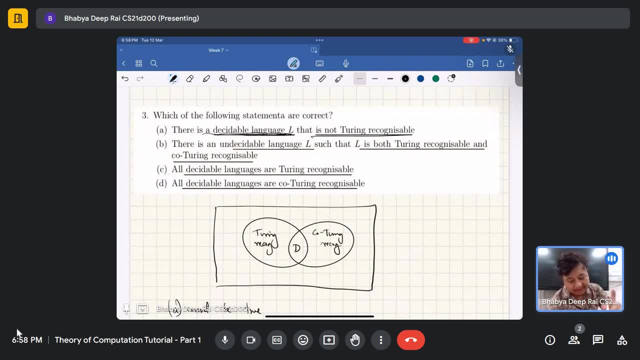 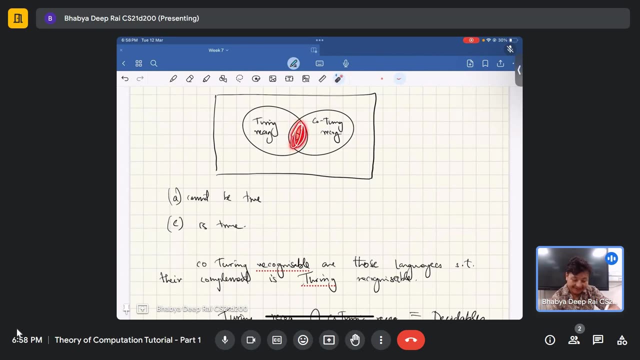 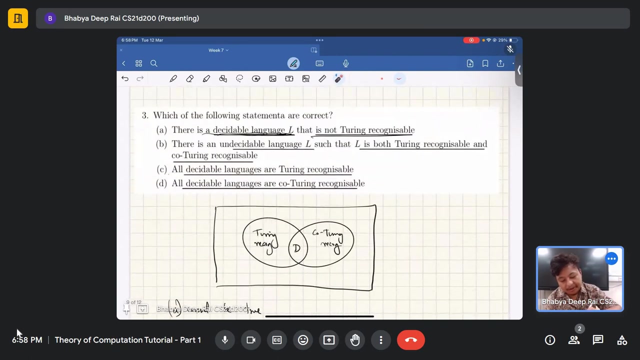 language l that is both turing recognisable and code turing recognisable, then it should lie here: right, it is both turing recognisable and code turing recognisable, but this is exactly the set of decidable, so b is false. finally, all decidable languages are code. 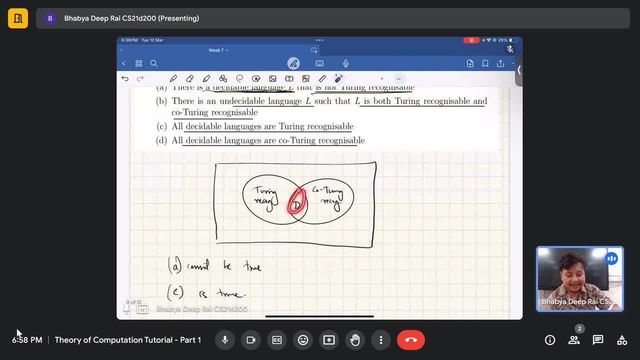 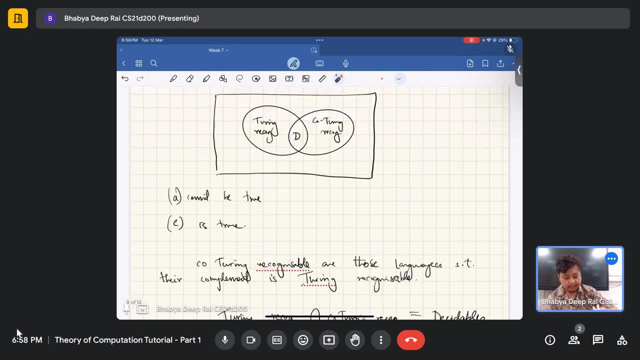 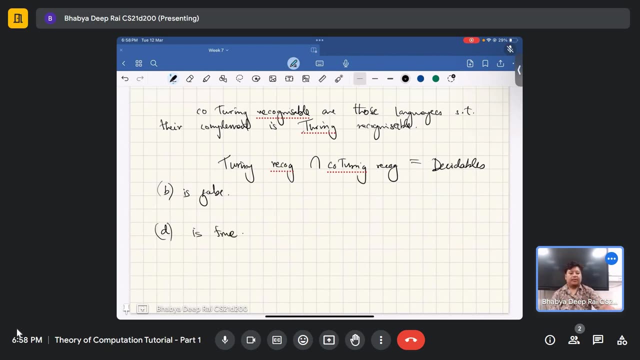 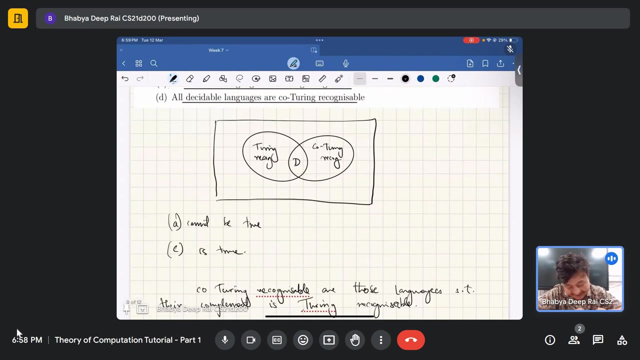 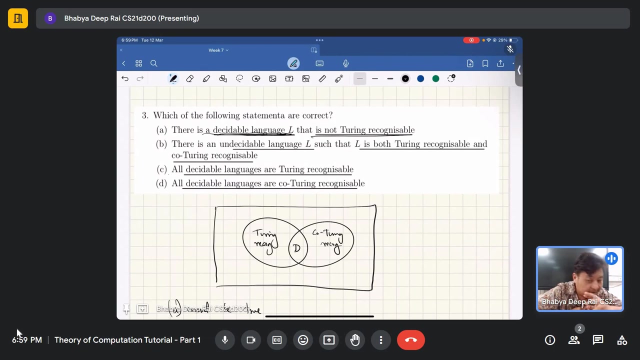 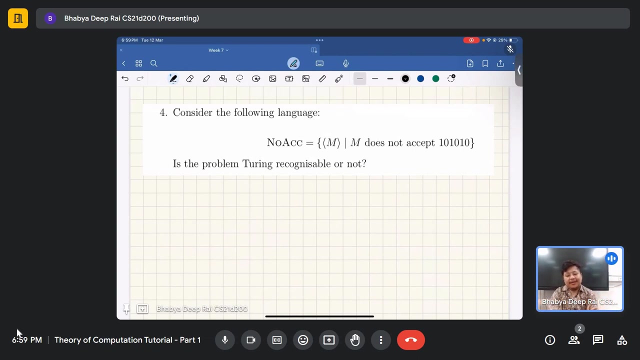 turing recognisable. all decidable languages are code turing recognisable. that is true, true, okay, so the correct options are c and d. all decidable languages are turing recognisable and all decidable languages are code turing recognisable. okay, now consider the following languages: language: 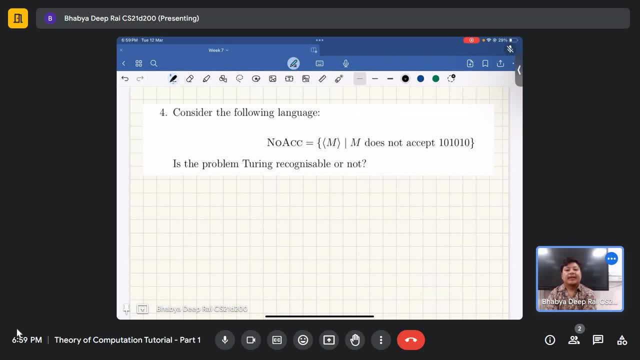 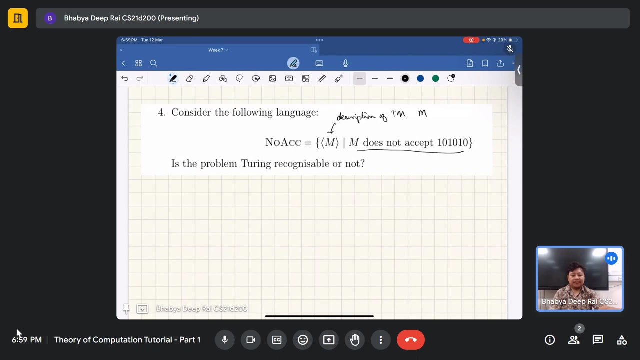 no act is defined as follows. it is the set of: okay, this is the description of turing machine. okay, this means description of a turing machine called m. okay, description of a turing machine, m, such that m does not accept the string one zero, one, zero, one, zero is the problem: turing. 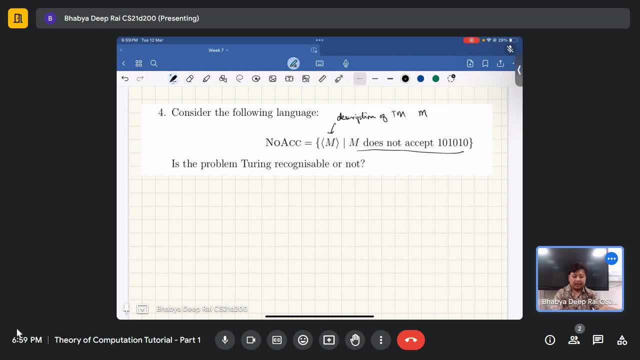 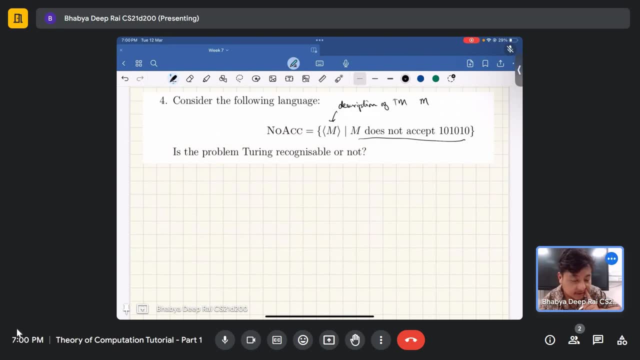 recognisable or not, cripto. so let's see if i need to build a turing machine for this. how do i know whether m does not accept it except 101010? well, the direct question would be: i'll just run them. okay, my universal turing machine will just. 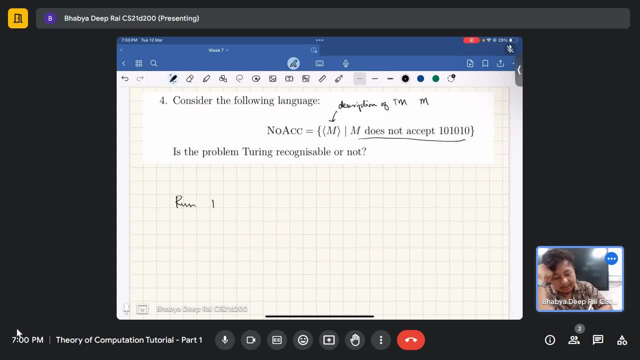 run m on the input 101020. let's do this, run them. run themali: 0, 1, 0, 1, 0.. If it accepts, then what should I say? Say no. If it accepts, then what should? 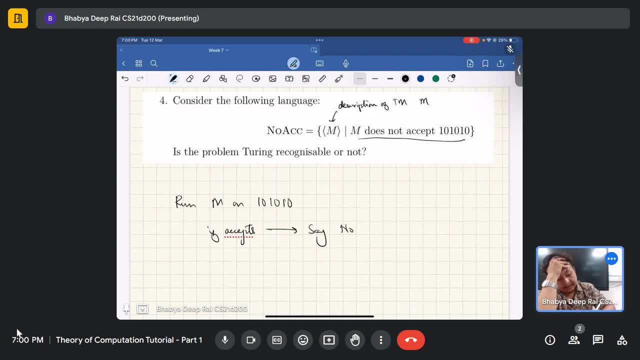 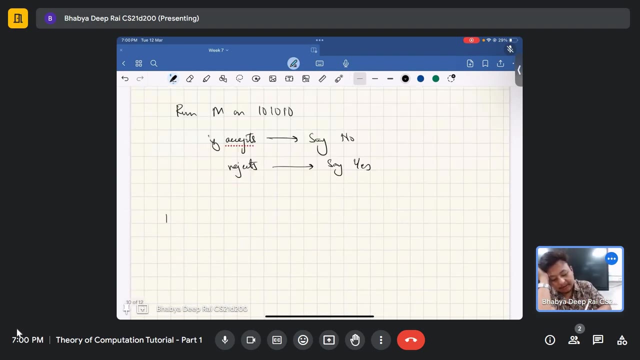 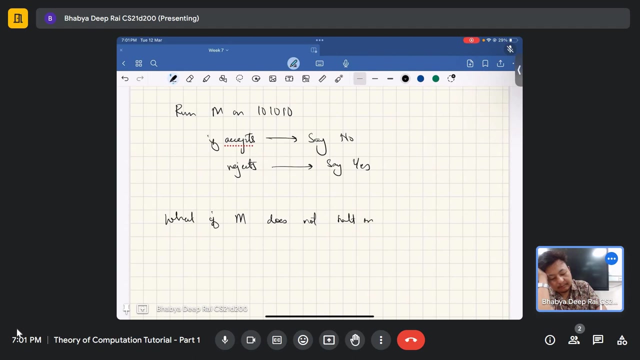 I say It should say no, And if it rejects, say yes. All well and good, But what if it does not halt on 1, 0, 1, 0?? What if it does not halt at all on 1, 0, 1, 0?? This is the. 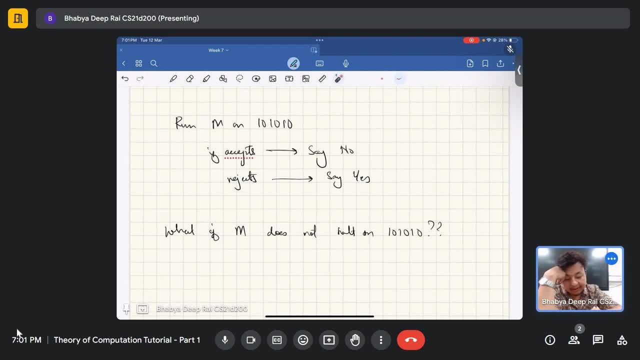 problem, right? Because then, on running M on 1, 0, 1, 0,, 1, 0, I'll just keep waiting for it to halt. If it accepts, I'm guaranteed to say no. If it rejects, it's guaranteed to say yes. 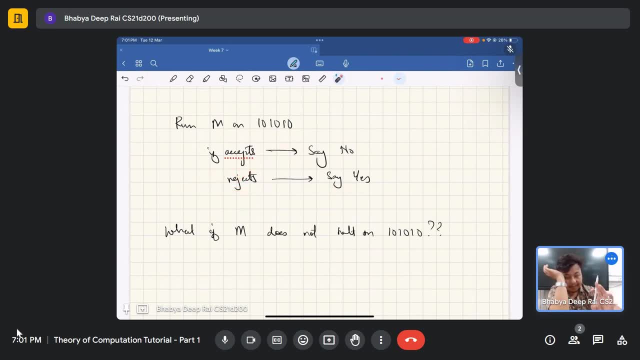 But if it loops, I just keep waiting. But remember, if it loops it means that the language does not belong to M. The string does not belong to the language of M. If it belongs to the language of M, it means it halts and accepts. So if it loops, it is as good as. 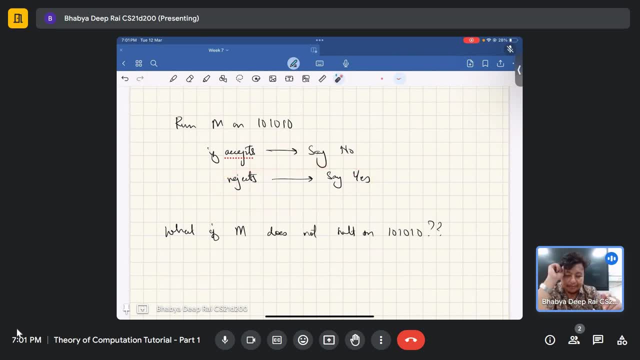 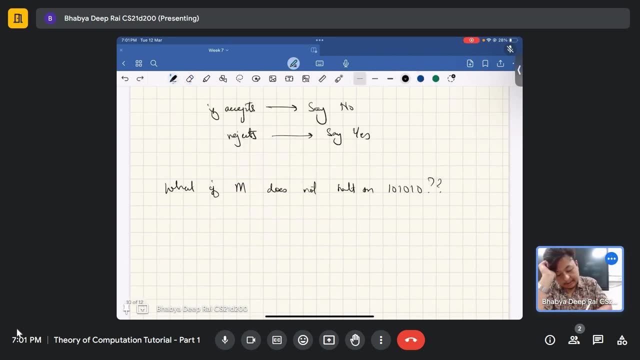 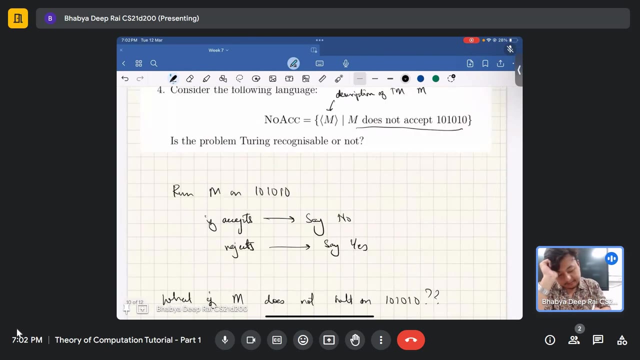 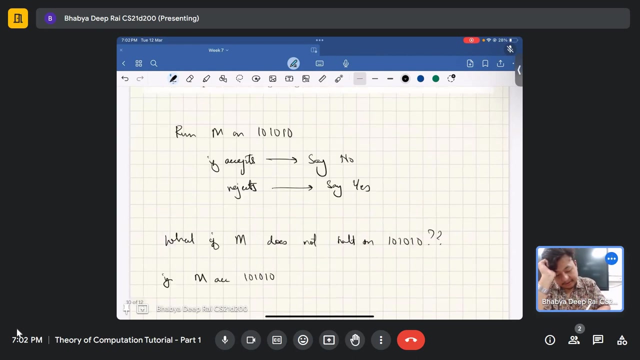 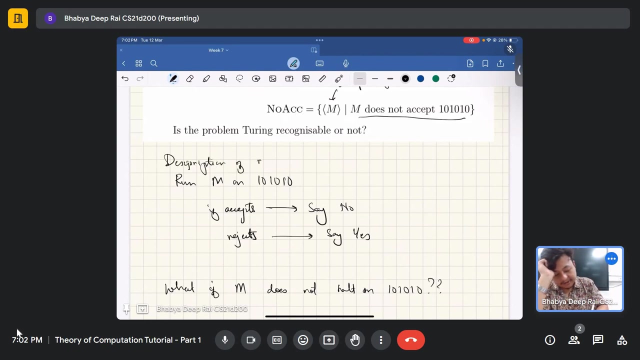 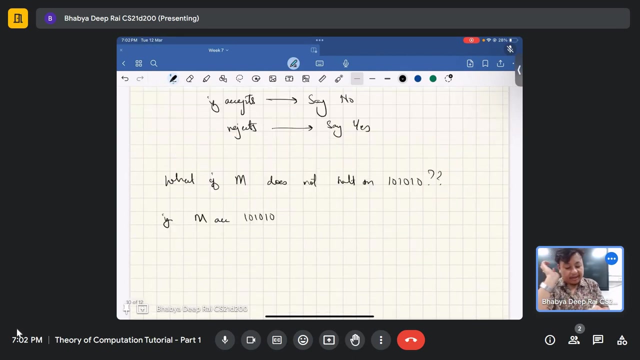 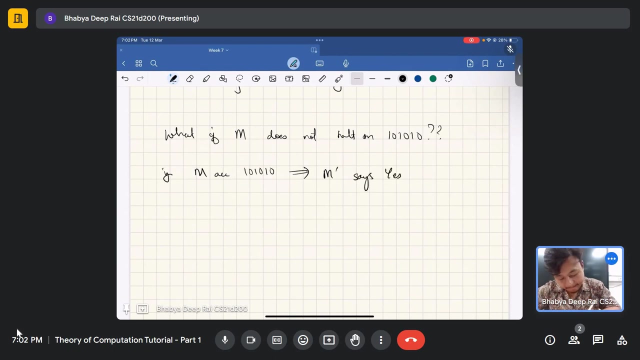 rejecting actually, But we just don't know when to stop it. If M accepts 1, 0, 1, 0, 1, 0, let me call this bigger machine description of machine M prime. If M accepts 1, 0,, 1, 0, then definitely M prime says yes. However, if M does not, 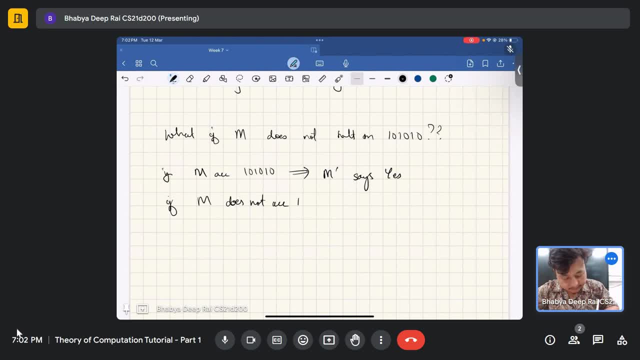 accept, that is, it may reject or loop. Alright, Thank you very much. Thanks you, Bye, bye, loop. If that happens, m' says no or loops, Because we are talking about the case when it does not accept It accepts, then we should be saying no. If it does not accept, then 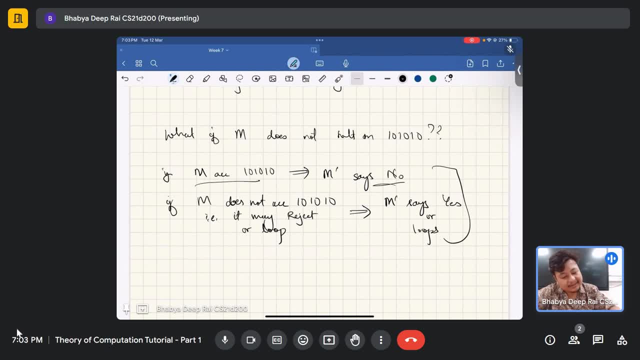 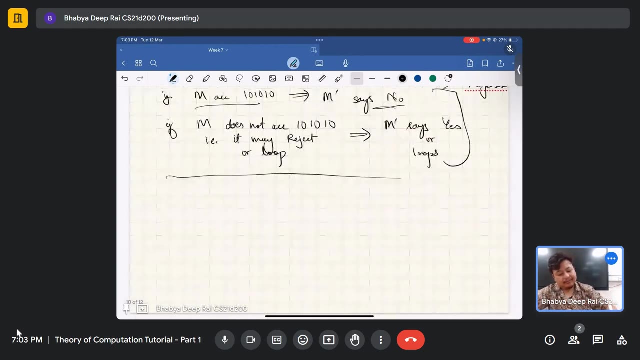 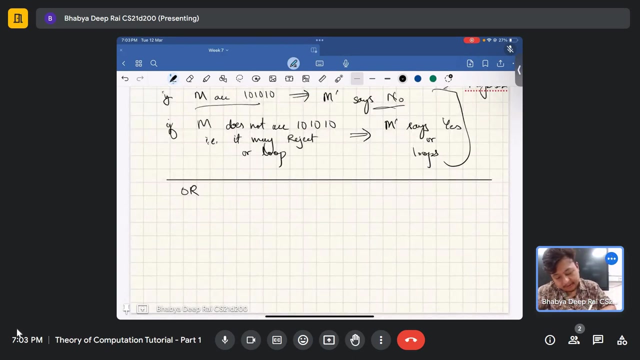 m' says yes or loops. What is this? One way is that it is directly the definition of code Turing recognizable. Next, another way to show this: that it is code Turing recognizable or alternate approach. What is the alternate approach? The alternate approach is look. 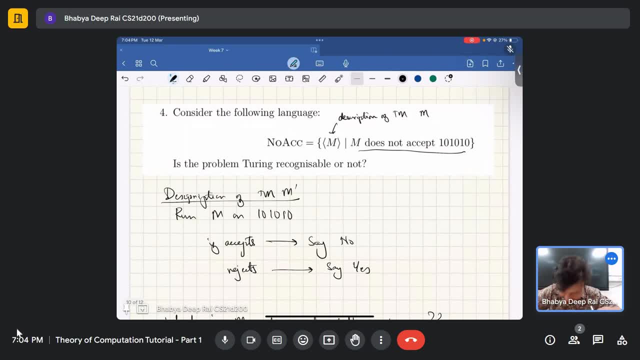 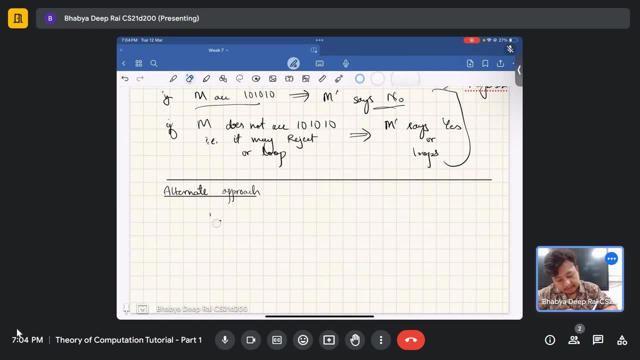 at the complement of the language. Noack is all the descriptions of m such that m does not accept 101010.. So noack complement is a set of expressions of m such that m does not accept 101010.. It is a set of all strings, all the machines, such that m accepts 101010.. 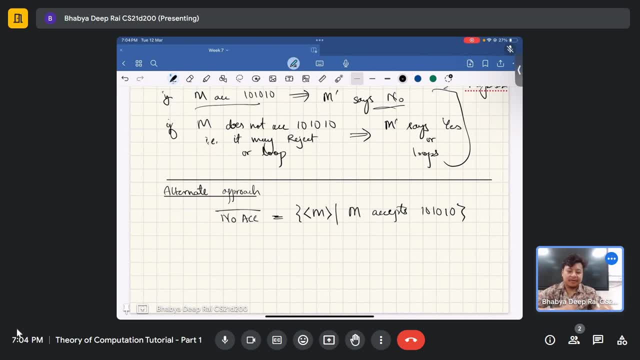 And this is Turing recognizable. Why? Because, again, what is the machine for it? I will just run m on 101010.. If it says yes, if it accepts, then I will say yes, If it does not accept, then it may loop. So in the yes case it will definitely be loop. So in the yes, 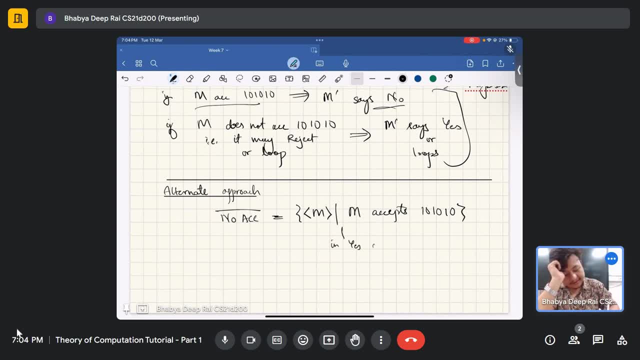 case we know if it accepts 101010,. we would definitely know by just running it. No case may loop. What does this mean? This means noack is a set of expressions of m such that m does not accept 101010.. So in the yes case we know if it accepts 101010, we would definitely. know, by just running it, No case may loop. What does this mean? This means noack is all using m, such that m does not accept 101010.. If it is awesome, then no law exists, then it will accept m. So this means noack is a set of expressions of m which has a set. 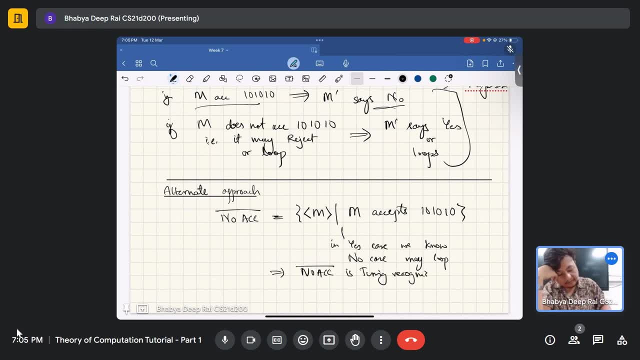 of expressions of m that we are getting from m. So it is something like this, which means noack. there is something called Turing recognizable as if turingRecognizable If noack complement is Turing recognizable, its complement. remember the complement. 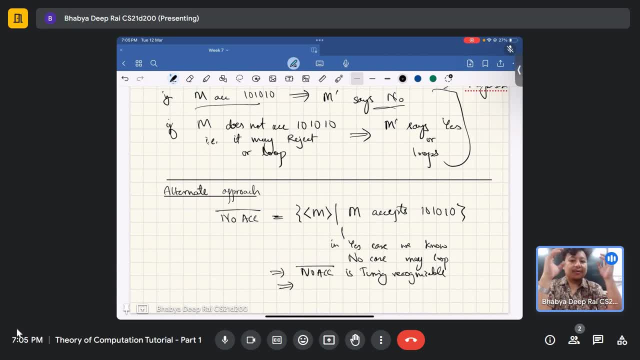 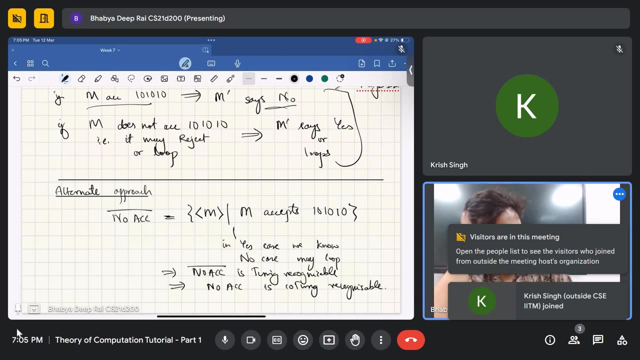 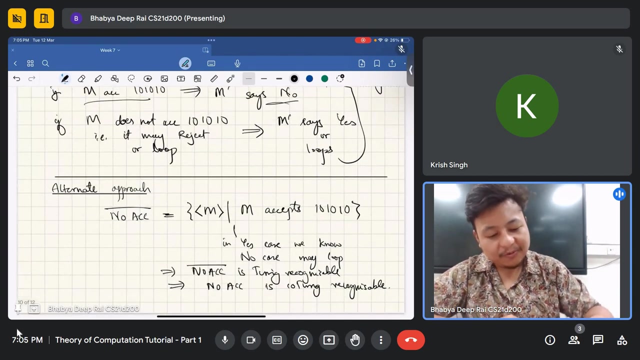 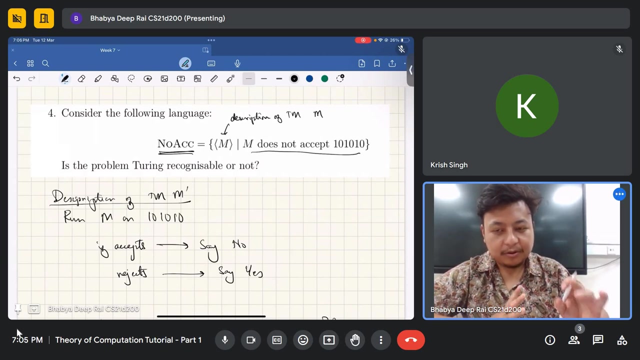 of a turing recognizable language is coturing Recognizable, So it's complement is coturingRecognizable And I will not uh. so so at this moment we only know whether this particular language, no act- is either recognizable or quote to recognize, but uh it, it may like somewhere in between right here, which is exactly. 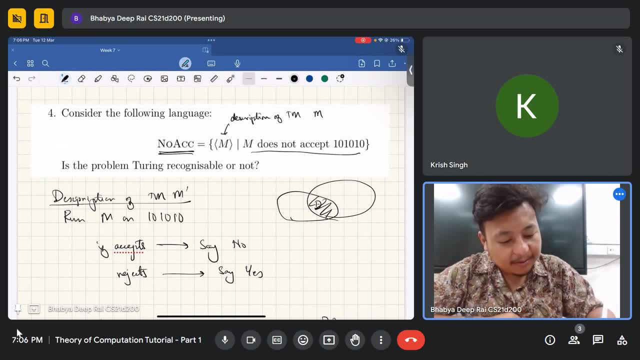 decidable. will i somewhere in between? but uh, currently i'm not doing, but in the next session i'll show that. oh, it cannot be inside disciples, it needs to be here in quote to recognize. so uh, right now the answer is quite vague, but in the next session we'll see why it is here. 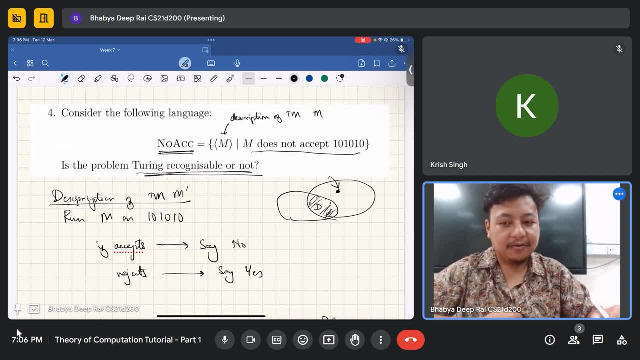 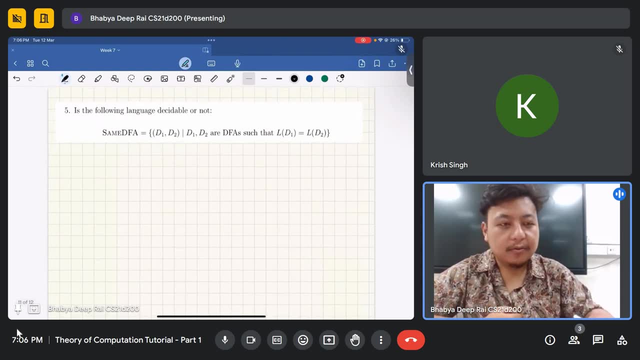 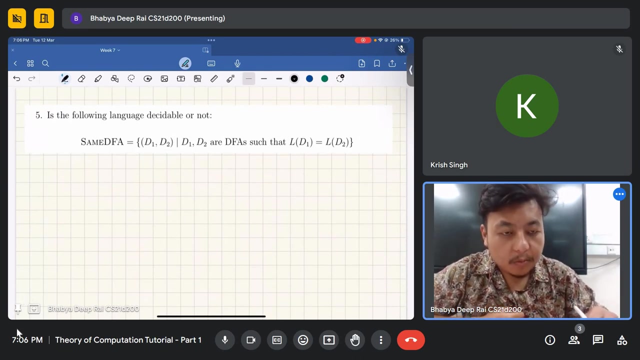 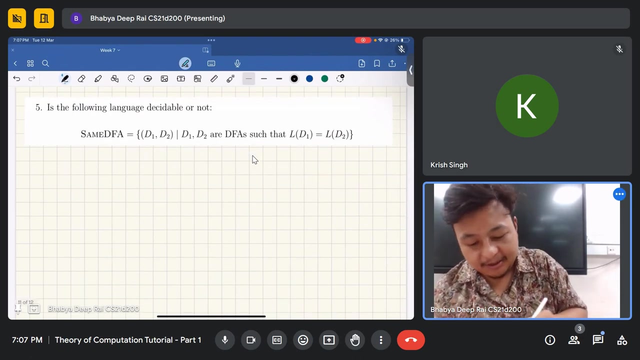 because it needs the idea of reductions and there is an interesting reduction. hello, uh, krish, is it? i am i audible? so i'm audible, right, oh, okay, okay, thanks, uh, okay, so, um, so here's the question. okay, so, uh. the question says: is the following language decidable or not? 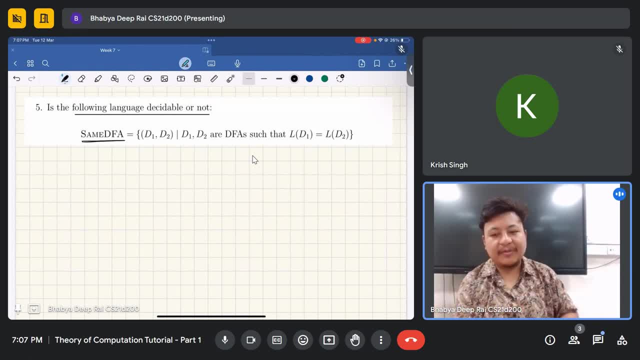 the question is called the language is called same dfa. okay, what is the inputs? it's, if they are two dfas, okay, d1 and d2, and they are in the language, only if language of the first dfa is equal to the language of the second case. okay, so input: there are two inputs. there are two inputs. 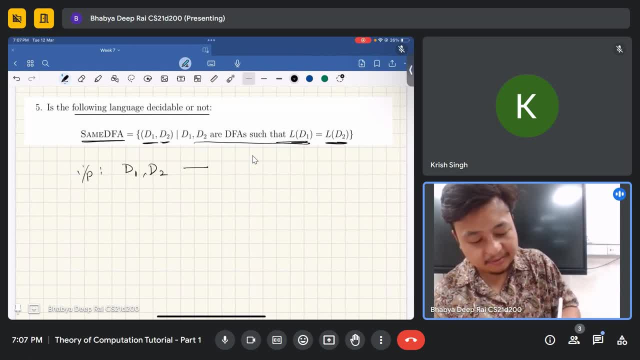 there are two dfas, d1 and d2, and the output is yes if l of d1 is equal to l of d2 and no. otherwise, if they have different languages, then they will say no. uh question is: is this language decidable? is this problem decidable? 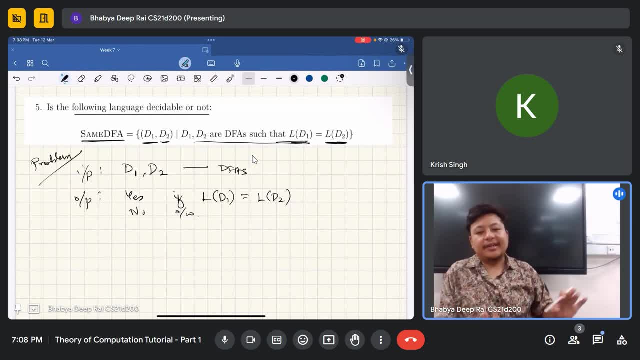 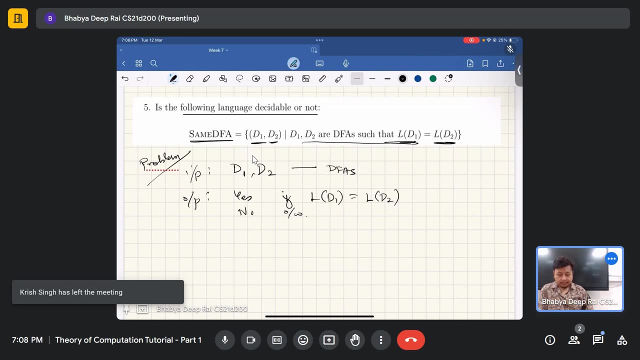 So this is another way to state it- this is probably decidable. in other words, can we find a total Turing machine for it? in other words, can we find a Turing machine that will always halt, that will correctly say yes or no and that will correctly say yes or no? 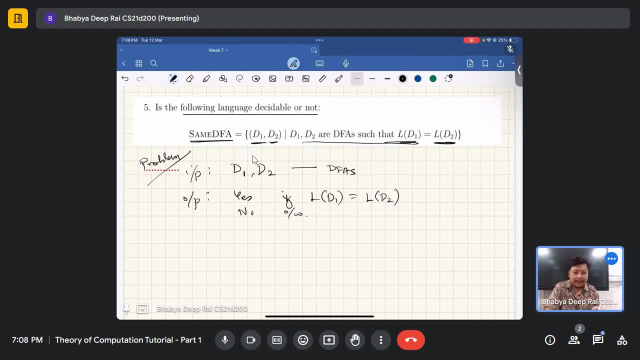 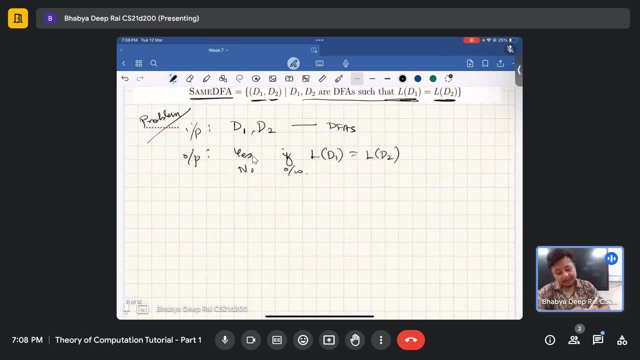 and it will say yes only if the languages are identical. So how do we solve this problem? So here we will use the closure property of regular languages, the closure properties of DFS. Recall that. So here we will use the closure property of regular languages, the closure properties. 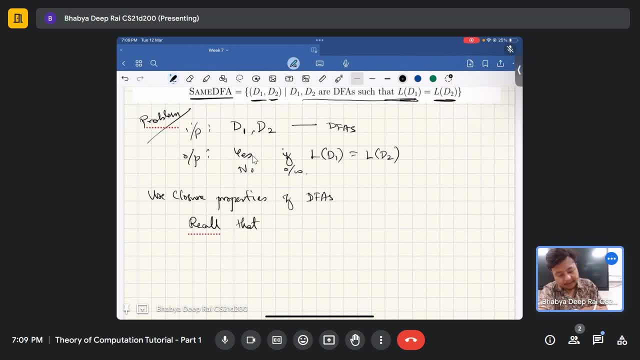 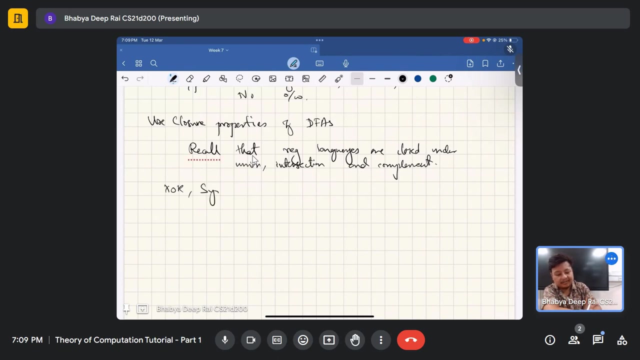 of DFS Recall that Regular languages are closed under Union Interception and Conflict. they are closed under Union Intersection and Conflict. Now we will do an interesting thing. We will look at what is called the XOR or Symmetric Difference. What is the Symmetric Difference? 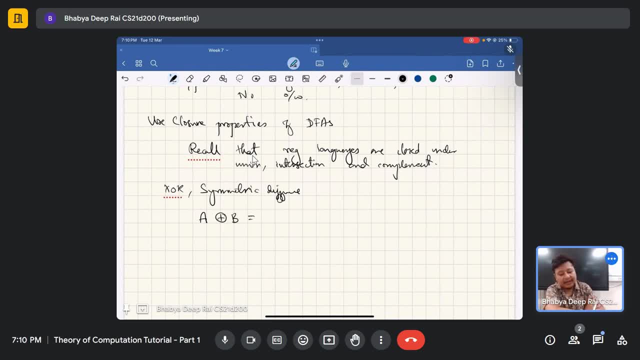 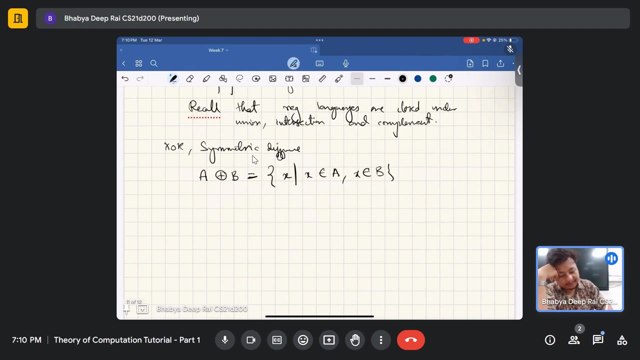 Asymmetric Difference, also called Parity Symmetric Difference. B is the set of all the elements X, such that X is in A as well as X is in B. So in other words, here is a Venn diagram: A, B, X. 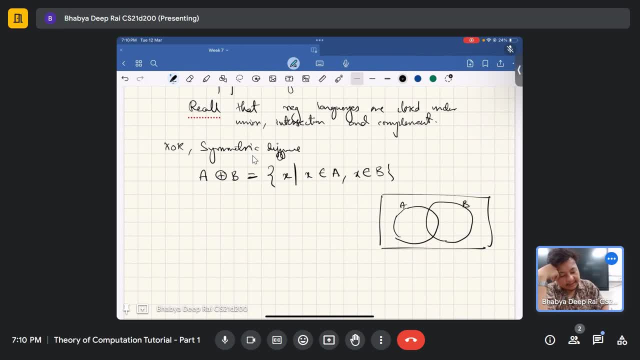 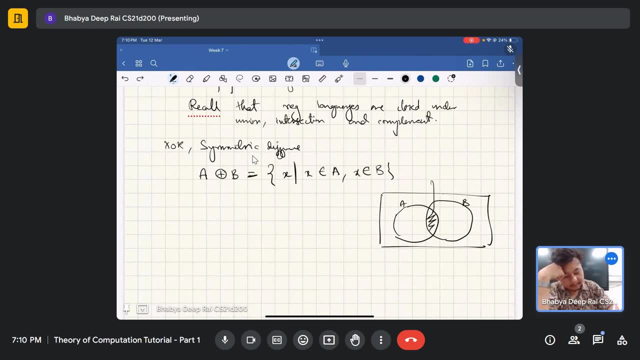 Okay, And this part, this part is A, sorry, oh, what am I saying? It is the opposite of that. A is not in B And X is in A, X is not in B, or X is in B, X is not in B. 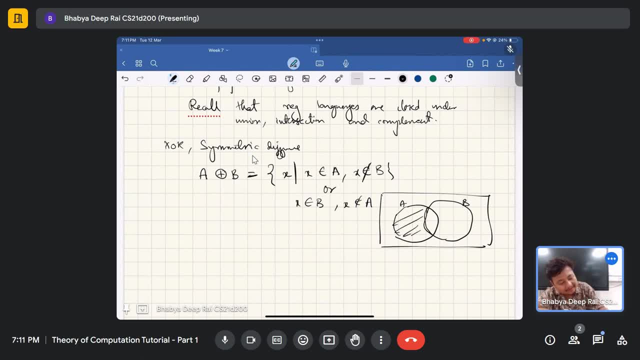 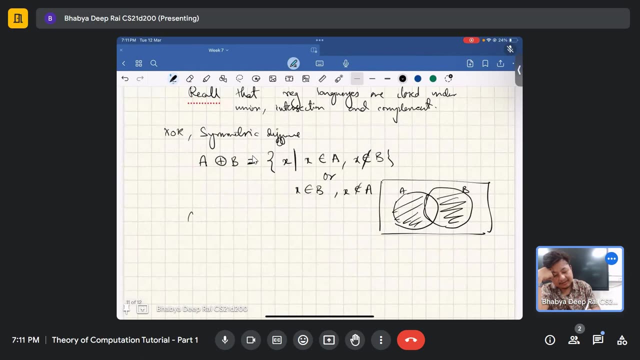 So what is the Symmetric Difference? They are, these parts, exactly the opposite of intersection. Since it is exactly the opposite of intersection, I hope you can already see that can also be written as follows: Okay, Okay, Okay. And, by the way, A, A, A, XOR, B can be written as follows: okay, 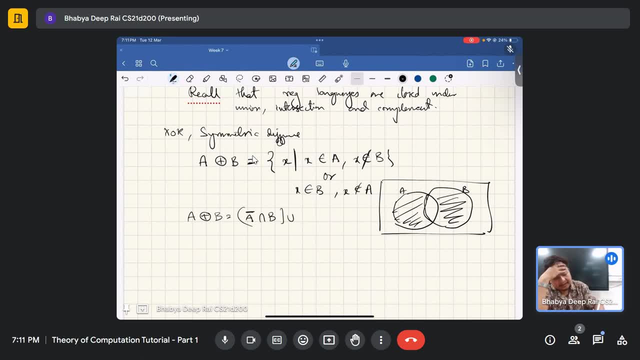 A complement, intersection B- union A intersection B- complement. You can verify this later. you can try this as an exercise. okay, This is exactly B complement, union, intersection A. this is exactly A complement, intersection B. okay, And then this is the union. 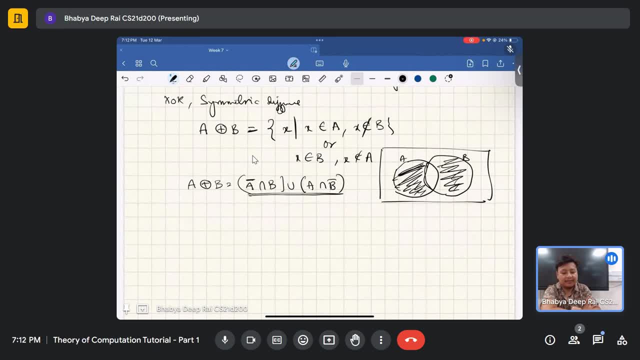 So this we can easily compute, We can always. So we can always build a DFA computing A XOR B asymmetric difference. okay, Because? why? Because it consists of intersections, unions and complements. Nothing is violated here. By violated I mean, see, if I do a complement, I can find a DFA for this, and this is also. 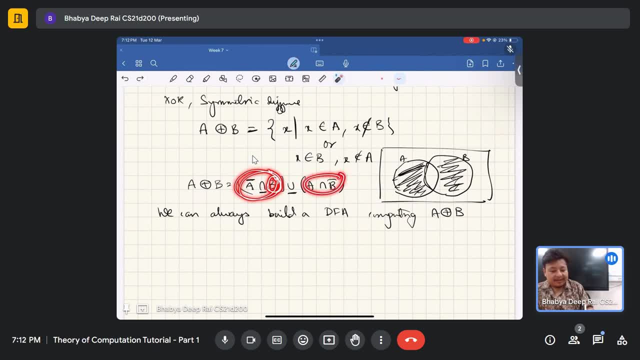 regular, So I can find a DFA for this. this is also regular and the union is also regular, So the entire thing is regular. you can always make a DFA for this and it's constructive. You can use some kind of subset constructions to achieve this. 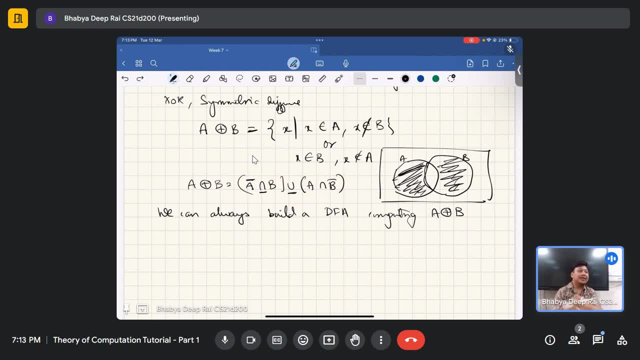 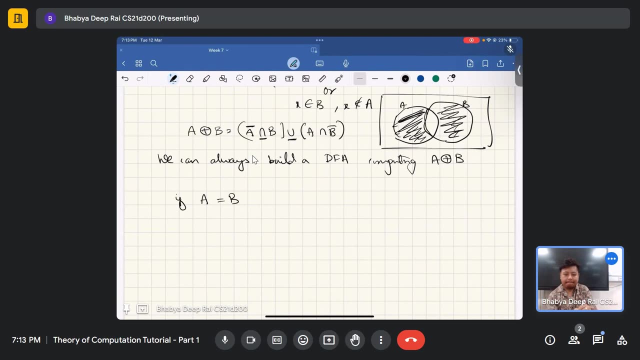 Okay, So we can always build a DFA which computes a symmetric difference B. Now what do we observe? If A is equal to B, then imagine these two circles. you know, fusing in A is equal to B. There is no element that is in A and not in B. 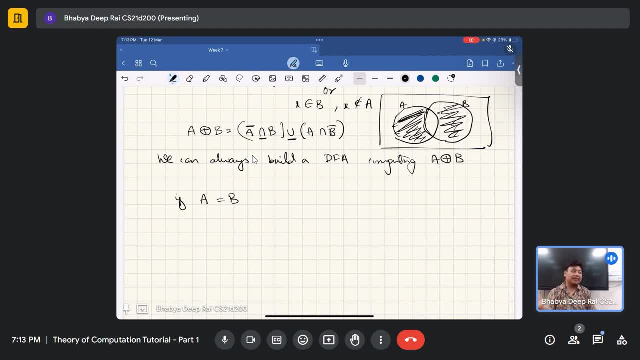 Okay, And there is no element that is in B which is not in A. Okay, So if A is equal to B, this is A and the same thing is B also. So there is no element which is outside inside A, but outside B and inside B, but outside. 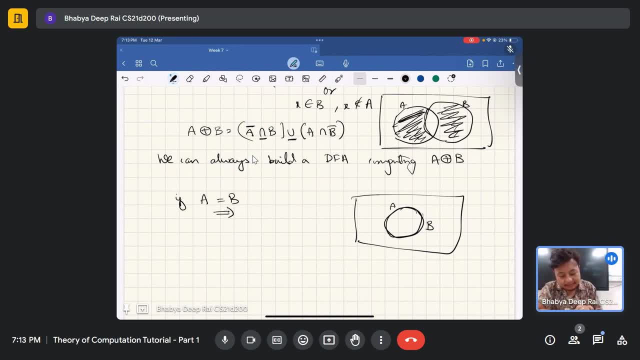 as you can see, Then, or you can also think of this as follows: A complement B union. A intersection B complement, right, So yeah, so A complement intersection B is nothing but B complement intersection B union, B complement intersection B union. 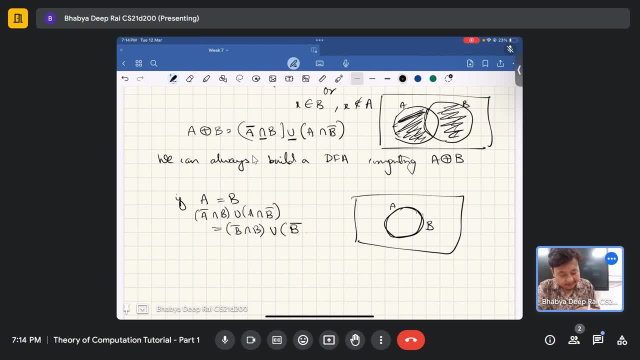 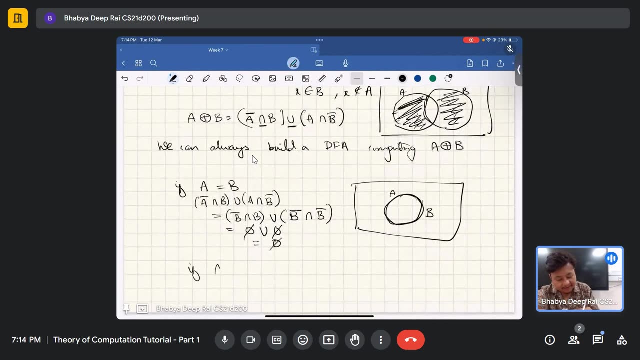 Okay, Okay, Okay. So A complement, intersection, B complement, which is empty set, union empty set, which is empty. So if A is equal to B, there is, it is empty. If A is not equal to B, similarly you can see that this is A XOR, B is not empty. 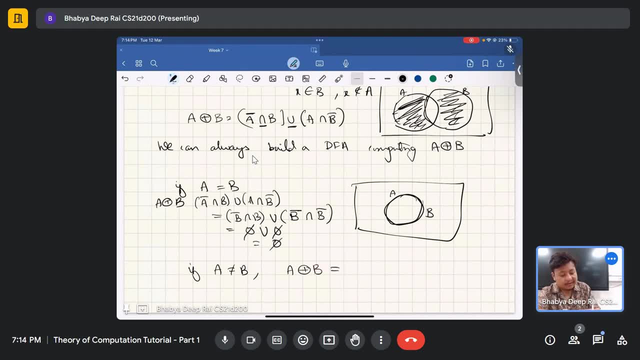 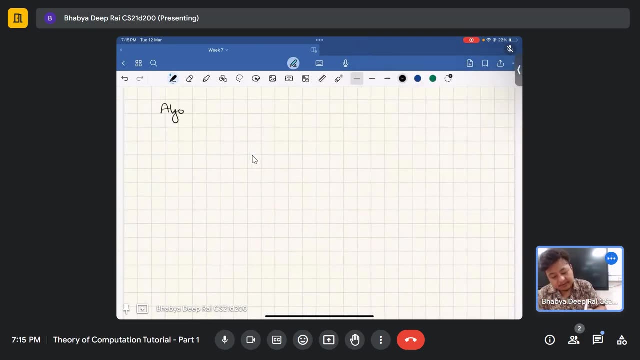 Okay, Okay. So now let's introduce A A, XOR B. Okay. Now the question is now here: is the algorithm here. is the algorithm okay? or the Turing machine description: okay. the input is d1 and d2, what do you do? construct dfa, d1x. 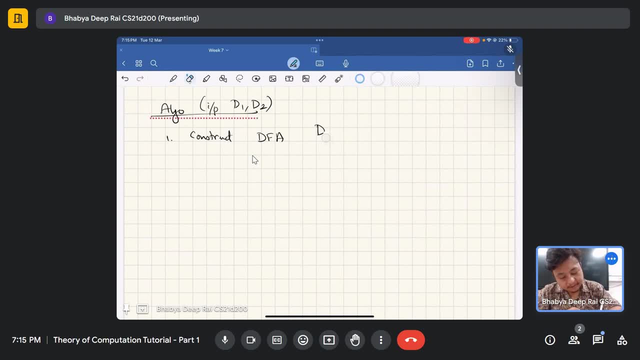 or 2, let me call it dxor, computing L of d1, xor L of d2, okay, now all I need to check whether it is empty. check if the language computed by d of xor is empty. If it is empty, then what would it imply? they are the same set output: yes, if no. 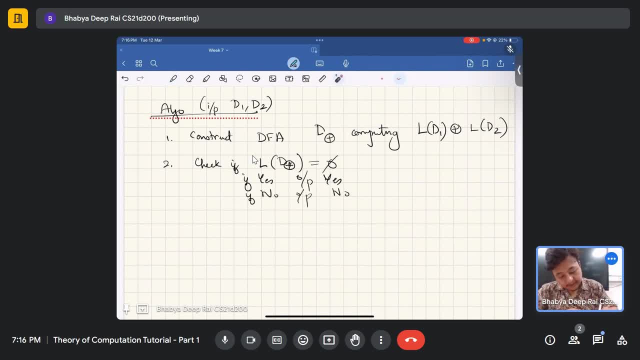 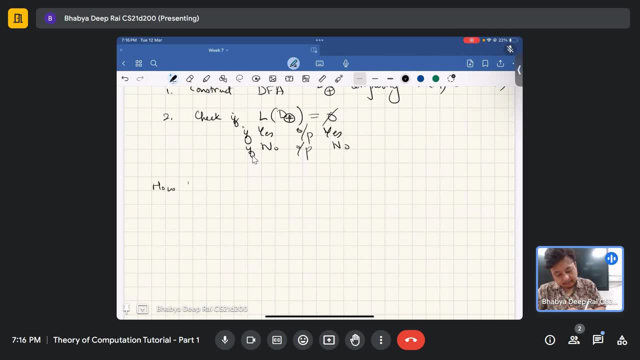 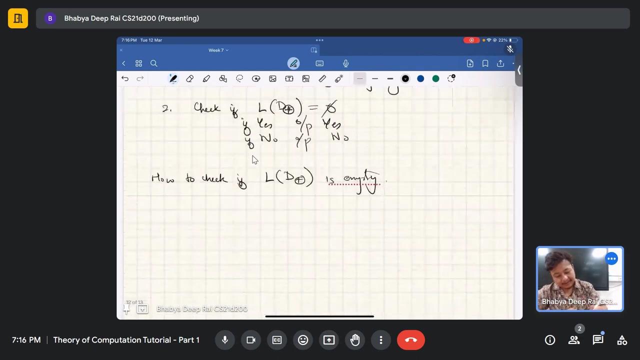 output. no, now it is not over yet. why is step 2 possible? how to check if language of this is empty? Simply check if there is a string that lands to the final state, or simply check that. is it even possible to ever land in the final state? 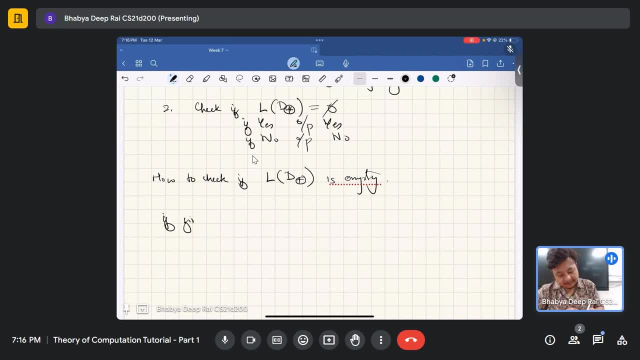 If final state is not reachable, are not? if final states are not reachable, then no string will be accepted. right? If no string will be accepted, then the language is empty. language of that particular df is empty. If the final states are not reachable at all, then 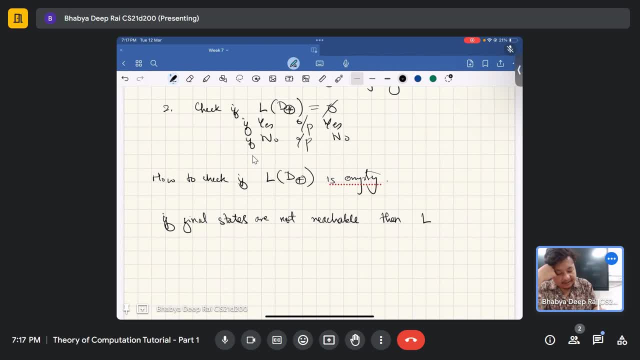 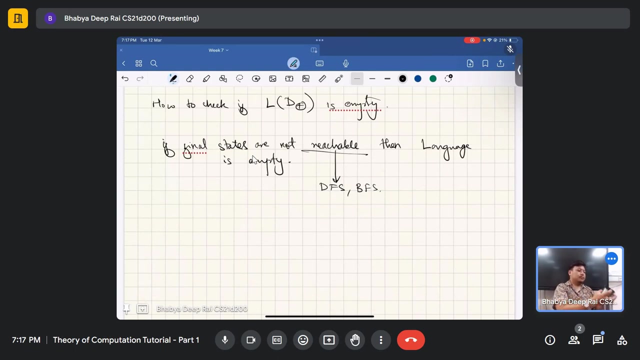 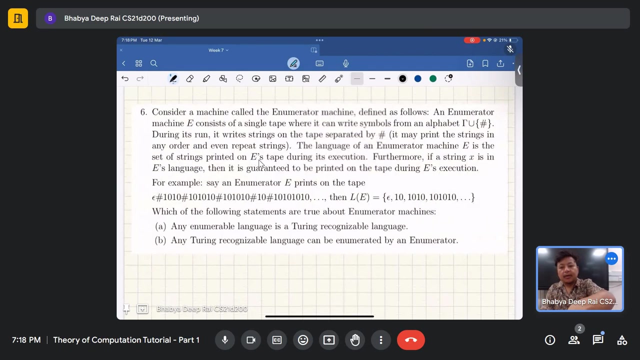 language is empty, Okay, Okay. And how do you do this? You can simply use some dfs or bfs, Okay, Okay. Next we'll look at another question called enumerator machine. Okay, Based on enumerator machine, So so. 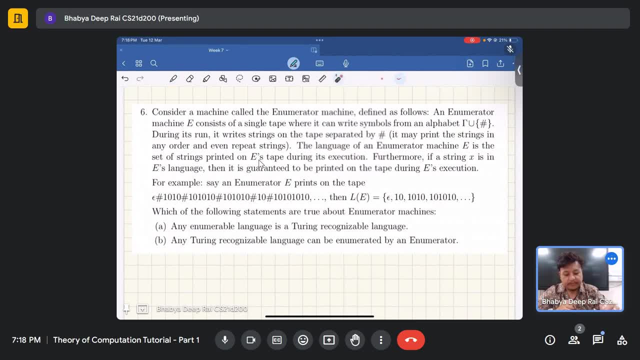 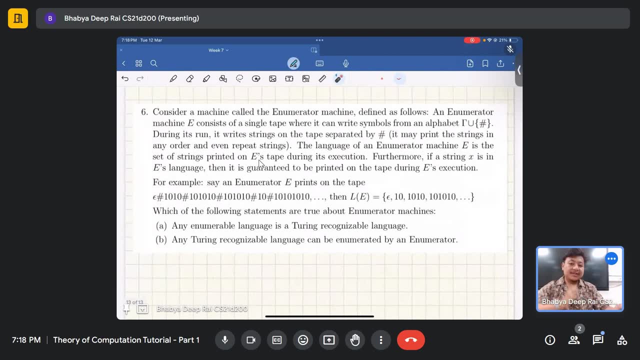 enumerator machine. Okay, What is an enumerator machine? So consider a machine called the enumerator machine, defined as follows: An enumerator machine consists of a single tape where it can write symbols from an alphabet: Okay, Gamma, union, some hash Okay. During its run, it writes: 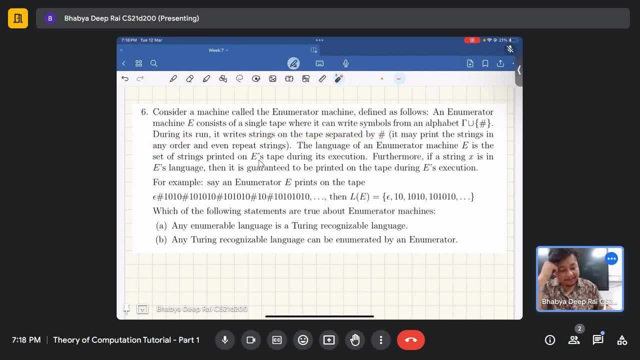 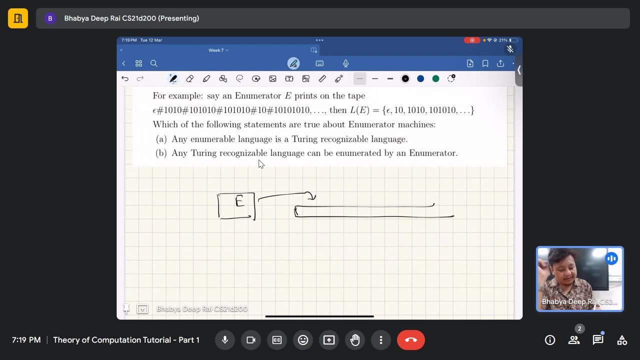 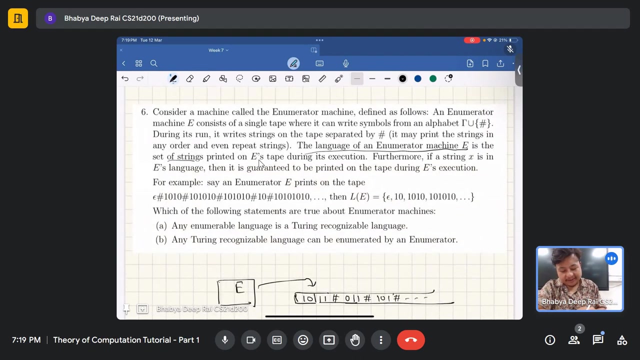 strings on the tape separated by this hash. It may print the strings in any order, even repeat strings. Okay, So here is a machine E and E can write strings And so on. The language of the enumerator machine E is a set of strings printed on E's tape during its execution. 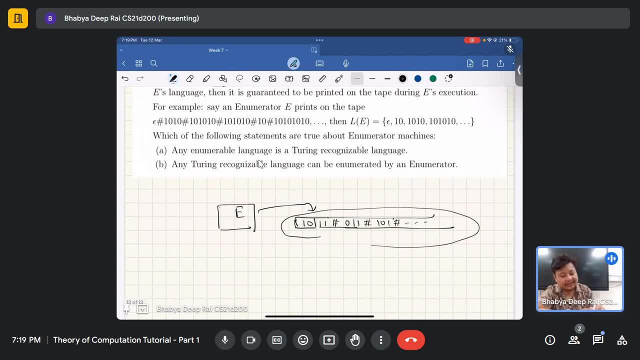 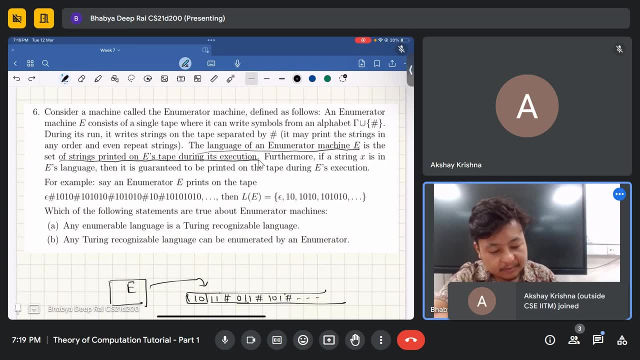 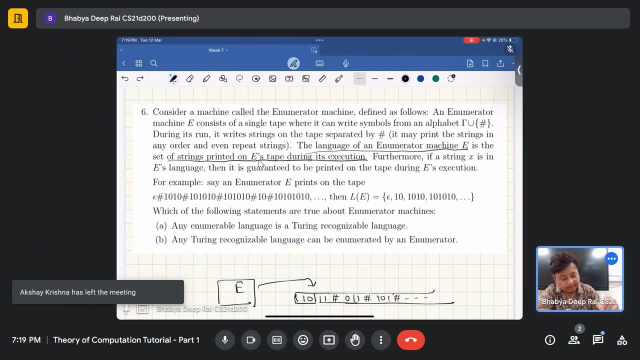 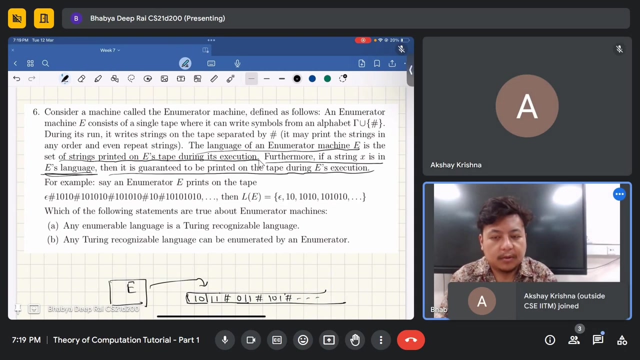 So what is the language? It is the set of all strings that are printed here, not counting the hash, And furthermore, if a string x is in ease language, then it is guaranteed to be printed on the tape during ease execution. Hello Akshay, am I audible? Yes, sir. 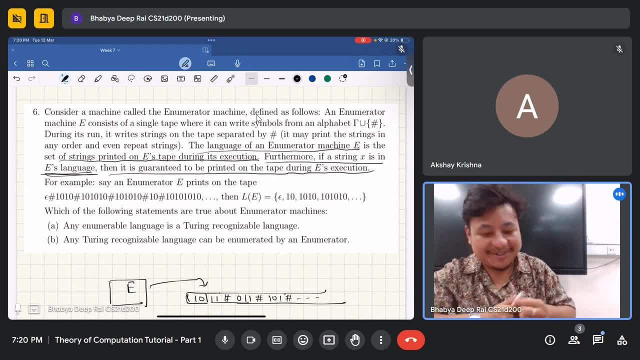 Today's session is a bit short, So this is the final question. actually, I will just discuss this one question. Okay, We will from the beginning and we will wrap up after that. Okay, Okay, So yeah, I will repeat the question. So consider a machine called the enumerator. 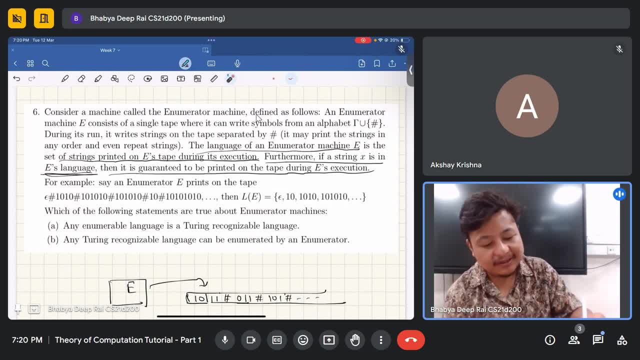 machine, and it is defined as follows. An enumerator machine consists of a single tape where we can write symbols. Well, it can write symbols from an alphabet, Okay, And then we can write numbers, And then we can write numbers, And definitely it can write symbols in a set of sounds. 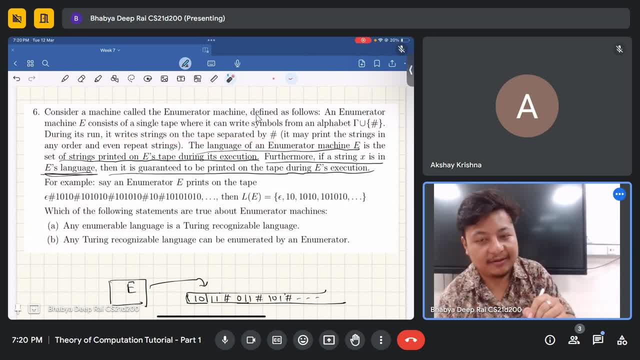 Okay, And during its run it writes strings on the tape separated by hash. Okay, And it may print the strings in any order and even repeat strings. So here is an example of an enumerator machine. It is, it is eeit is called e. 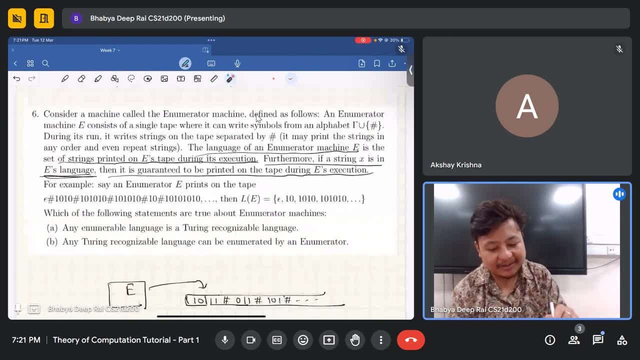 Okay, Like a tooling machine, it has a tape and an end and so on, But the tape is read-only, Okay, And it prints strings during its run here, Okay, Okay. So here is the enumerator machine. It writes all the strings and also the steps, Okay. 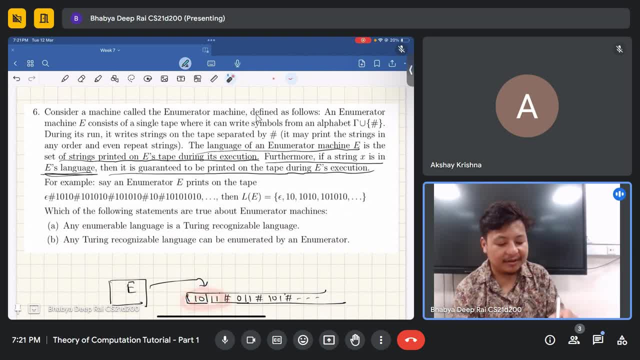 during its run it will print string as follows: 1011 and hash, then 011 and hash and 101 and so on. okay, the language of the enumerator machine e is a set of strings printed on e's tape during its execution. so whatever the strings are printed, okay. besides, the hash is together. they form the. 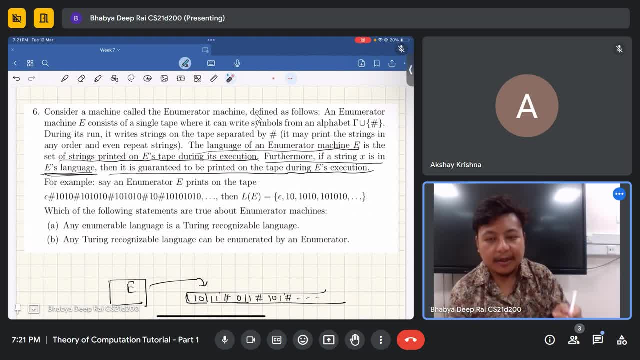 language of the enumerator machine now. furthermore, if a string x is in e's language, then it is guaranteed to be printed on the tape during e's execution. if it is in the language, then it will get printed. it may take a long time, but within a finite amount of time it will definitely print. 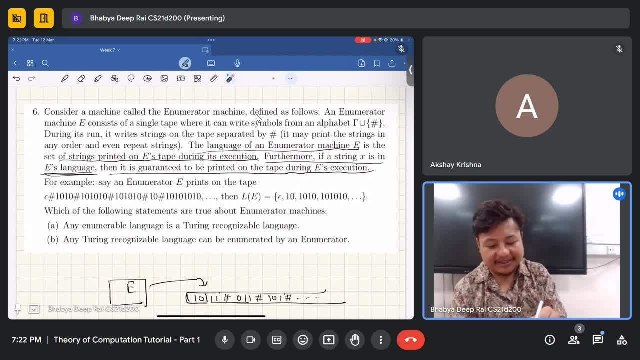 okay. now it says, for example: say an enumerator e prints on the tape epsilon 1010, 1010, 1010, 010 and this 101 and notice that it is splitting it in any order. it could print it in any order, it may not be increasing order, or something like that. um, and also that it may repeat strings. 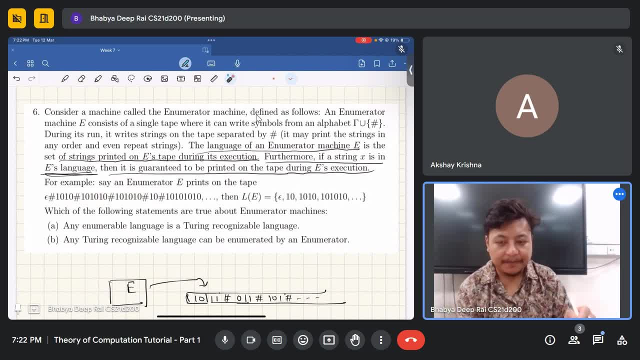 for example, this is repeated, so the repetition is possible, but when the language is all's, all the strings that are printed here is the language of the enumerator machine. Now the question says the following: which of the following statements are true about enumerator machines? 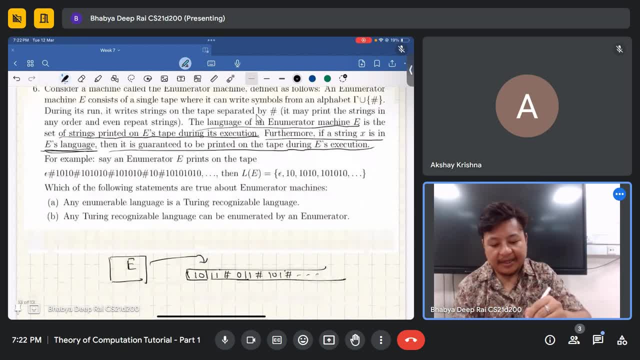 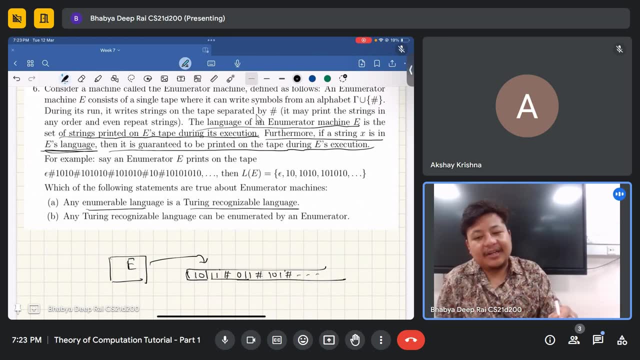 Firstly, any enumerable language, which means any language of an enumerator machine is a Turing recognisable language. And the second says: any Turing recognisable language can be enumerated by an enumerator, Which means any Turing recognisable language is an enumerable language. so it means that 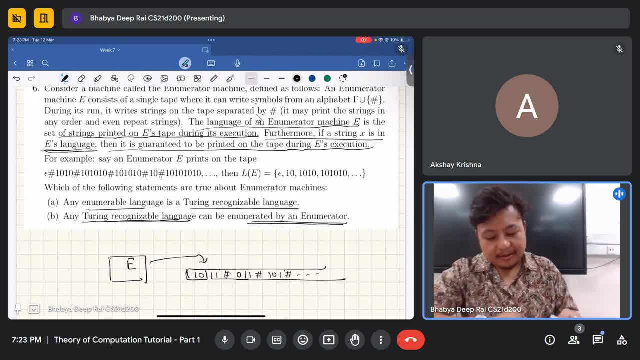 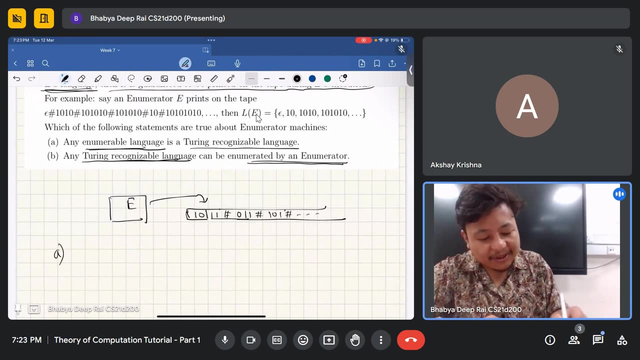 both of them are the same. If A and B, both are true, then it means the two languages are the same. so therefore, the models of enumerator machines and Turing machines are also equal. Let's see. let's see: A. Any enumerable language is a Turing recognisable language. 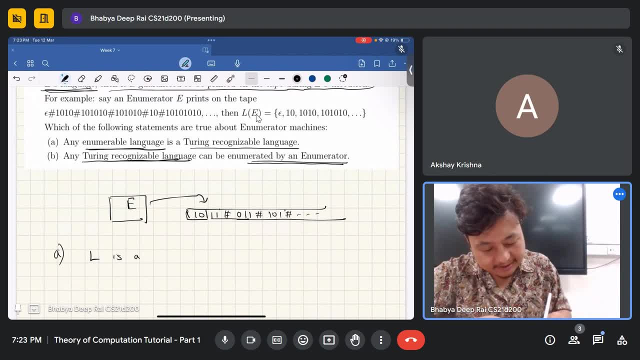 Okay, So let's say L is an enumerable language. What does it mean? L is an enumerable language. There exists an enumerator machine such that the language of that enumerator is L. Okay, Now we want to test if it is Turing recognisable or not. 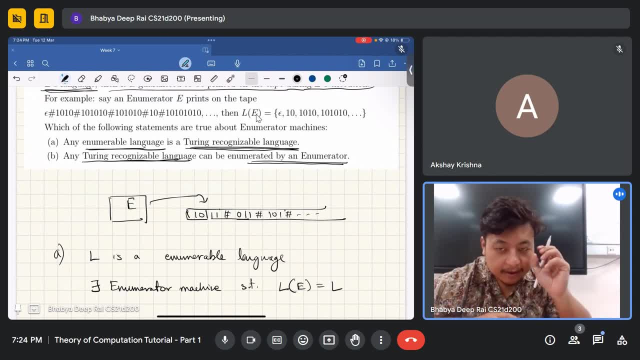 Okay, Now what is Turing recognisable Language is Turing recognisable If we can construct a Turing machine such that when the Turing machine is set to say yes, the Turing machine always alts. Okay, That is, if the string is in the language, then the Turing machine always alts and says: 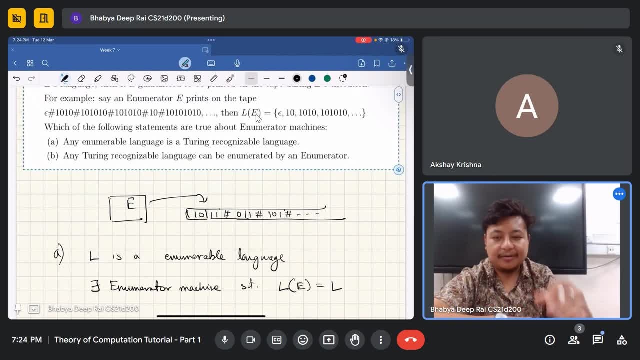 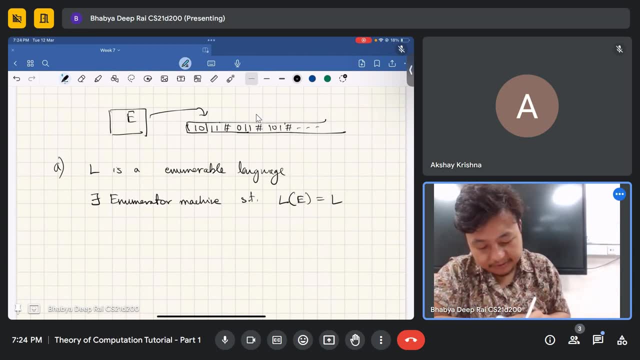 and accepts. If the string is not in the language, then the Turing machine may loop. Okay, So here is a Turing machine. okay, Turing machine M. on input, let's say X. Okay, The idea is very simple. We will just simply run the enumerator machine. 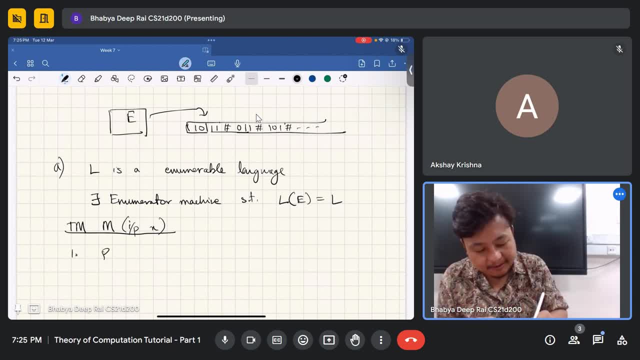 And it will start printing on the tape. Okay, Run E and use M's tape as E's tape. So what does E do? From the definition, it starts printing these symbols which are there in E's language. Okay, And if E prints, 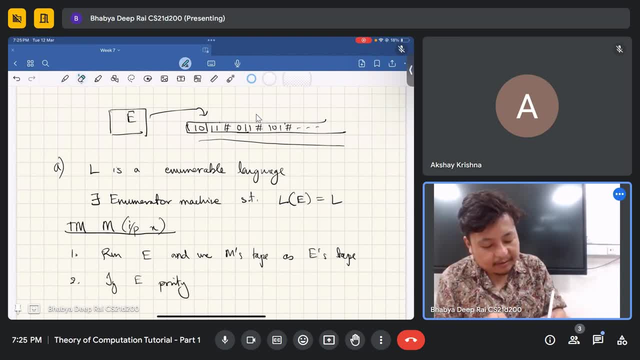 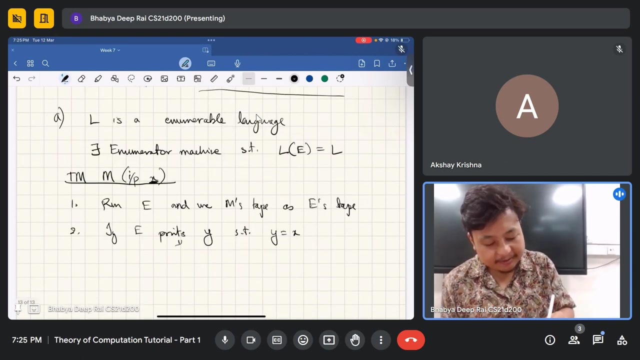 Okay, Okay, Okay. So let's say, if prints a Y, a string Y on the tape, Okay, Let's say this is Y, Okay On the tape, such that you know Y is equal to X. the input given to us then accept. 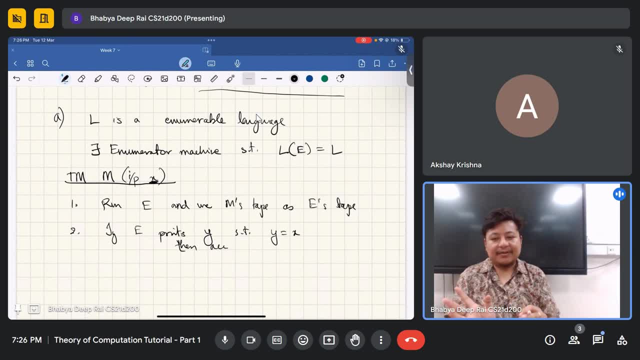 Then it means that that particular X was in Y's language also Was in E's language also. Okay, So now let's take this one also, And that's it. This is the description of the Turing machine. Now let's see why it is okay. 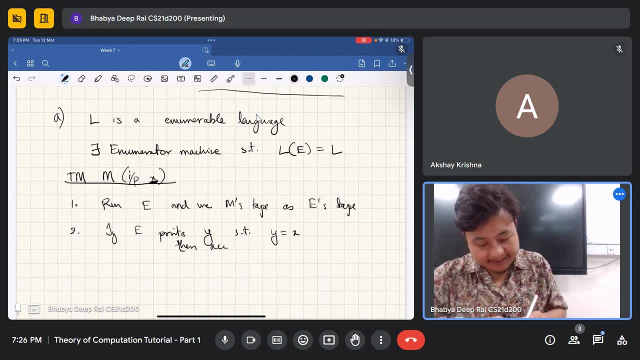 So if X is in the language L, then X is in the language of L of E. If it is in the language of the enumerator, then the enumerator of E is in the language of L of L, the enumerator. then what happens? Then E is guaranteed to what was written if 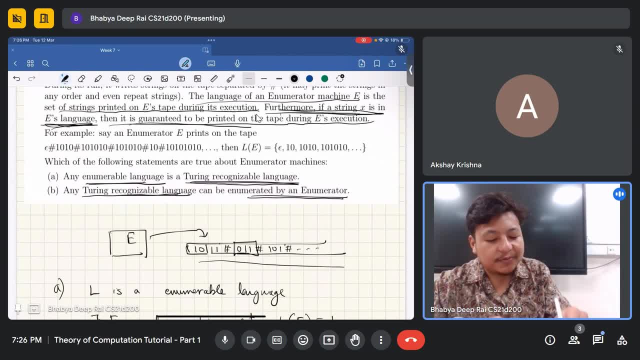 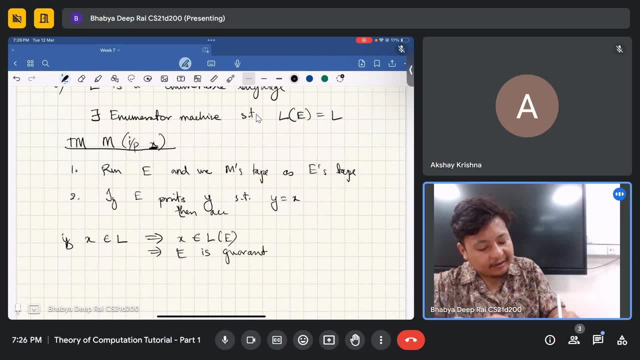 if a string x is in E's language, then it is guaranteed to be printed during E's execution. Then E is guaranteed to print x on tape. Now, if it is guaranteed to print x on tape, then y, such that y equals x, is always printed. Such a y is always found because x is in the language. x will definitely print. 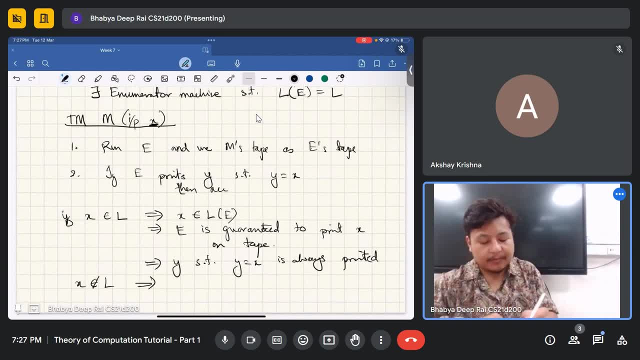 But if, let's say, x is not in the language, if x is not in the language, then what happens? E will never print a y such that y is equal to x. E will never print a y such that y is equal to x, and this means m will never halt. But even though m will never halt, it is fine, because we just want. 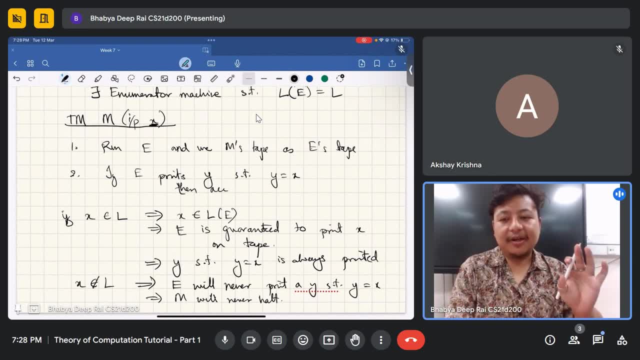 m to be Turing recognizable machine. I mean the language of m to be Turing recognizable. And we can see that y is in the yes case, that is, if x is in L, then there is Turing. And, for example, what is the language of x? 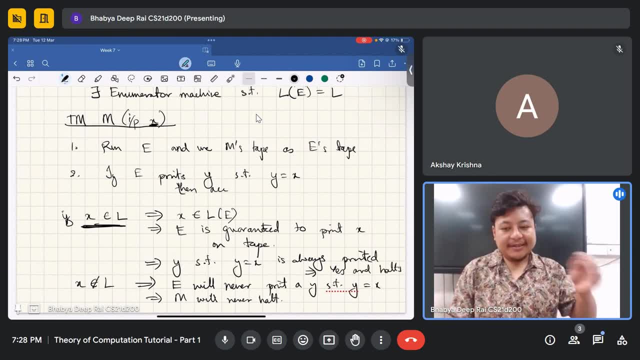 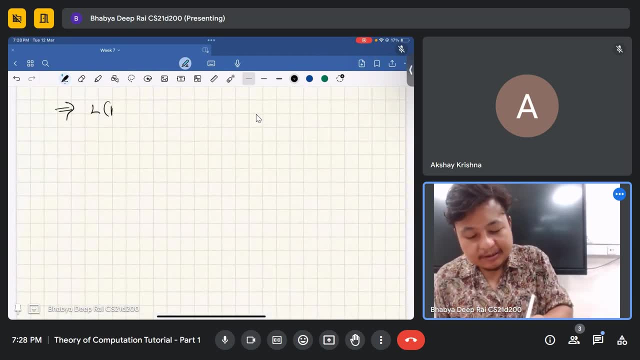 In the s case, it primts s and it halts always. So, during the s case, it always halts, which means that the language of the machine is Turing recognizable. And what is the language of the machine? it only accepts those strings which are printed by the enumerator. so which is? 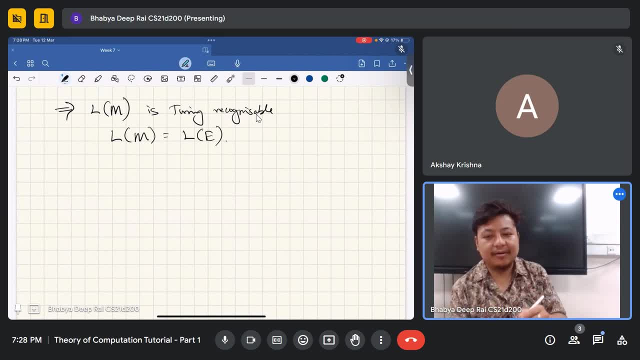 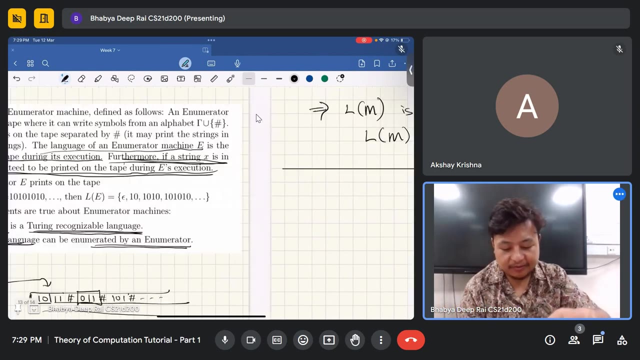 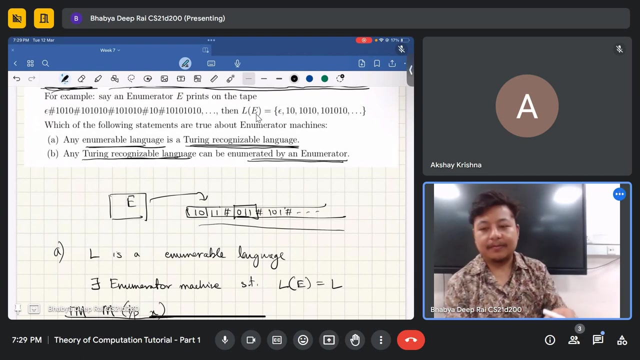 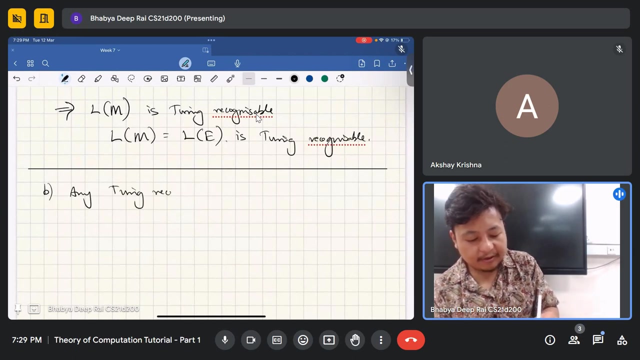 nothing but a language of e. so both are and both are same and therefore language of the enumerator is Turing recognizable. okay, so this is sort of the easier direction. so we'll look at the second direction. any Turing recognizable language can be enumerated by an enumerator. any Turing recognizable 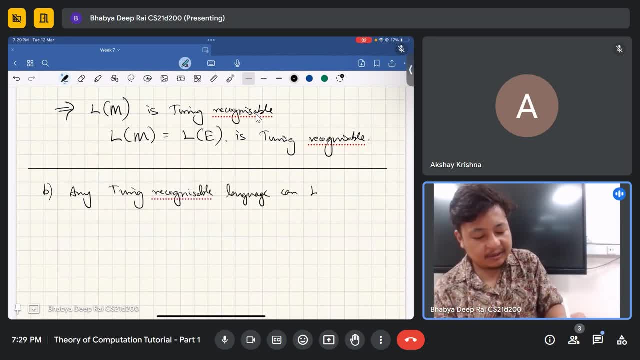 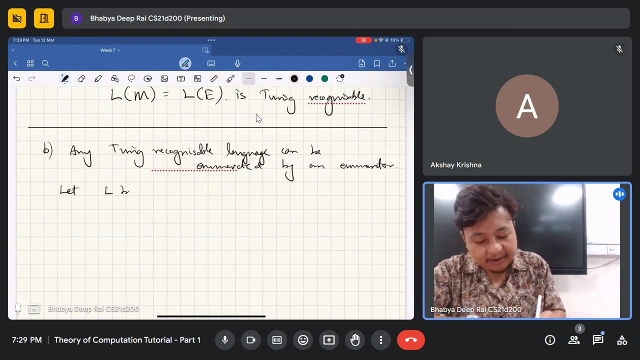 language can be enumerated by an enumerator. so this time we'll do the opposite. we'll take a Turing recognizable language, let. let let L be Turing recognizable, okay, and since it is Turing recognizable, there is a Turing machine for it. via a Turing machine, M right the Turing. 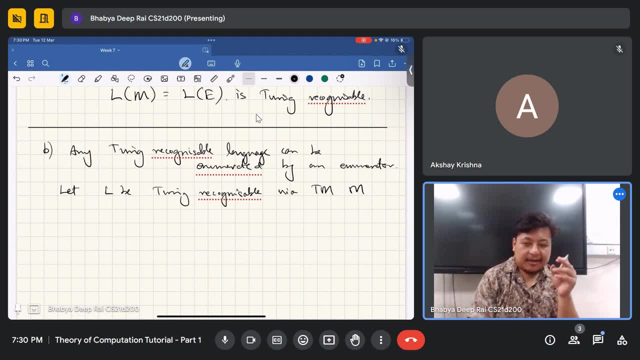 machine may not always hold. now we want to create an enumerator, which means we want to have a mechanism of writing on on on the tape and starting enumerate, behaving like an enumerator, basically printing all the strings in the language. so here is a simple way to. there is the. 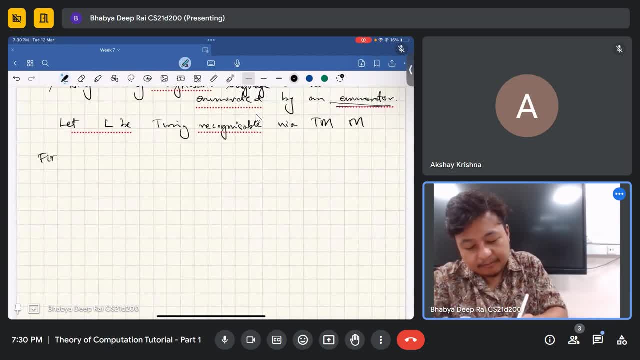 first attempt. okay, here's the first attempt. first attempt is as follows: description of enumerator e. enumerator e: see the examples C. by original methods: have sitting there already and the random edition: click text or again on othersubjective. okay, now enumerator E: there dot a mini inputs. few recalls it is just keeps. 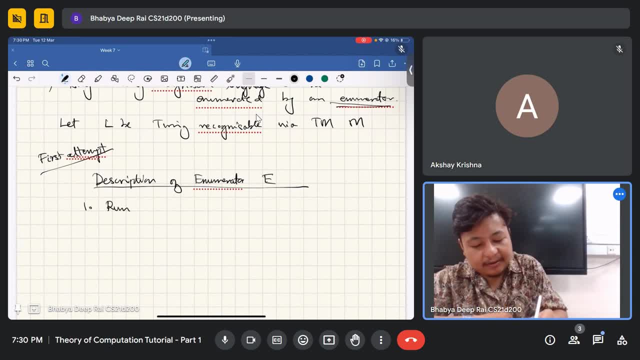 finally printing symbols on the tape. so first, what I'll do is I will go across all y, or I'll call it x. x equals aamız дел�� o Be a 많은 y. x, S, L, equals, you know everything x in sigma star. go across all x in sigma star for each of. 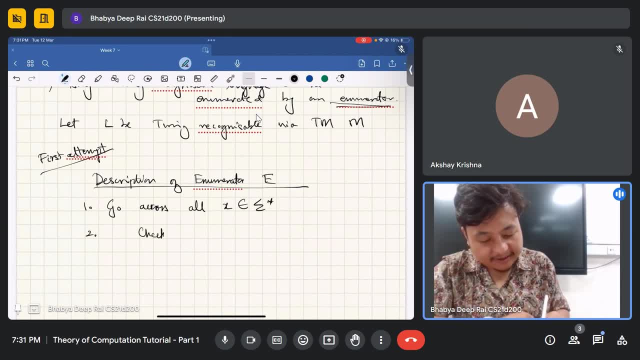 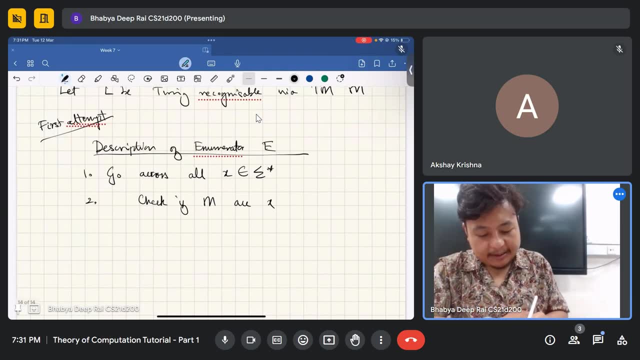 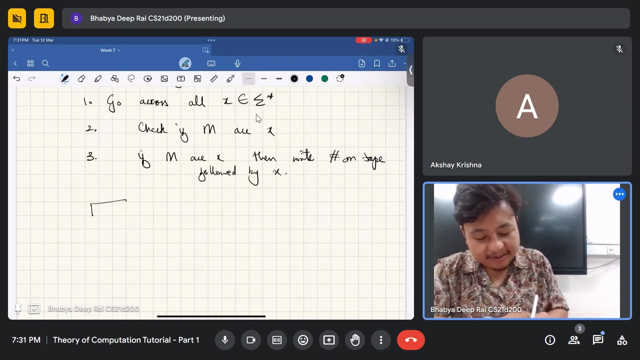 these x check. if m accepts x, okay. and 3 is: if m accepts x, then write hash on tape followed by x. for example, like if say, 101 is accepted by the Turing machine, then on the tape we'll write 101,. 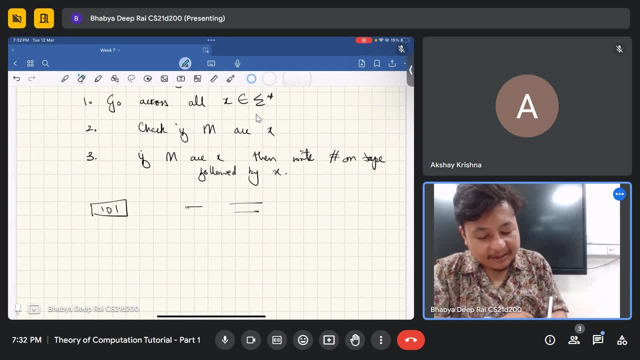 and then hash- okay, sorry, hash. and then 101, and let's say the next: we try on 110, and it is not accepted. then we won't write on the tape and let's say 111 is accepted by this. 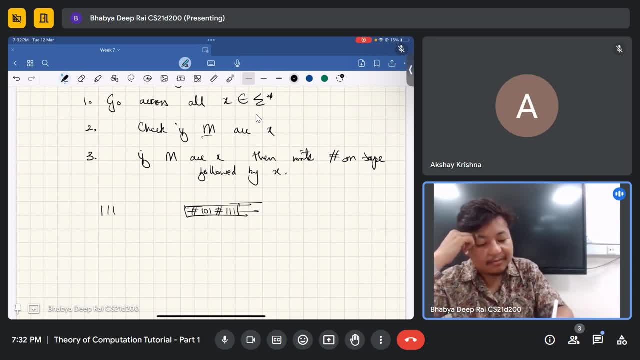 this Turing machine right by m, then we'll write 111,. so since the language of the enumerator is not nothing but the strings that are printed on the tape, right, since it is nothing but the strings that are printed on the tape, the language of the machine m is identical to the language of. 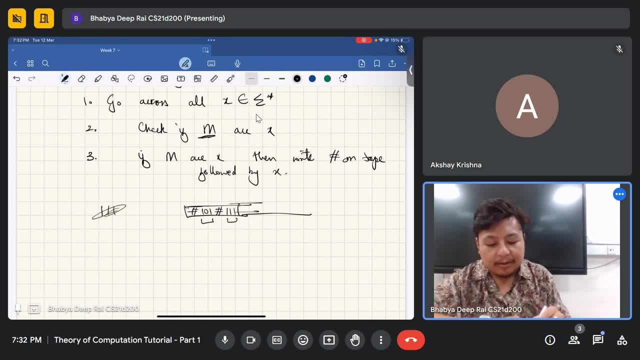 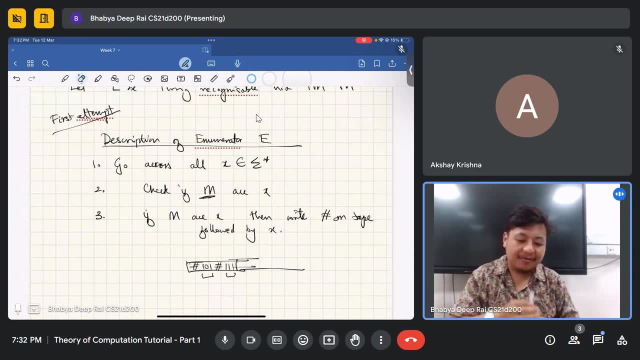 the enumerator that we constructed. but there's a slight problem with this small problem. can you think about? can you think about this for a while? what is the what may be the problem here? The logic is straightforward: we are trying to build an enumerator and we go across all possible. 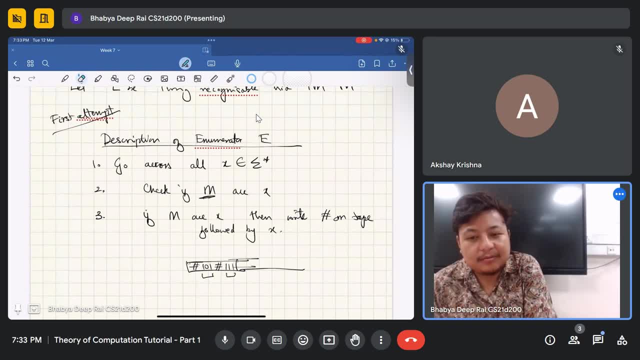 strings and we check whether the string is accepted by m or not. if it is accepted, then we write the string on the tape. and we keep doing this and we build an enumerator right whose language is same as the language of the machine: m. 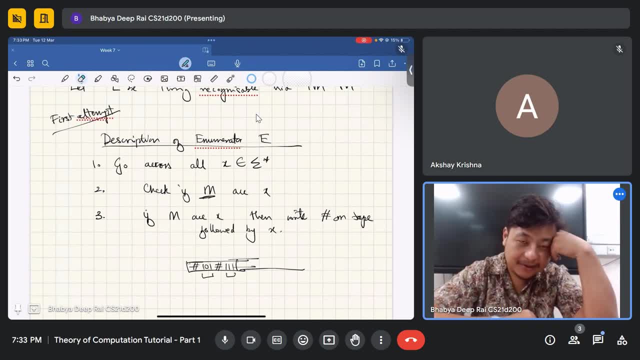 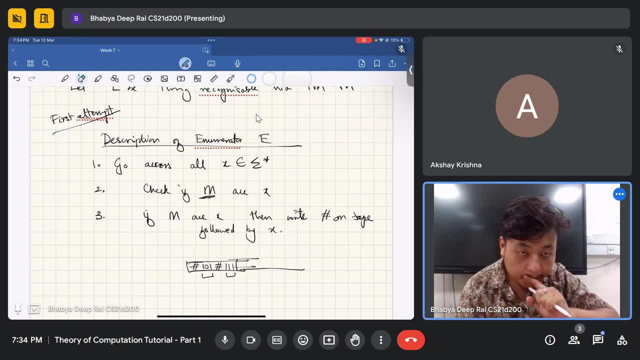 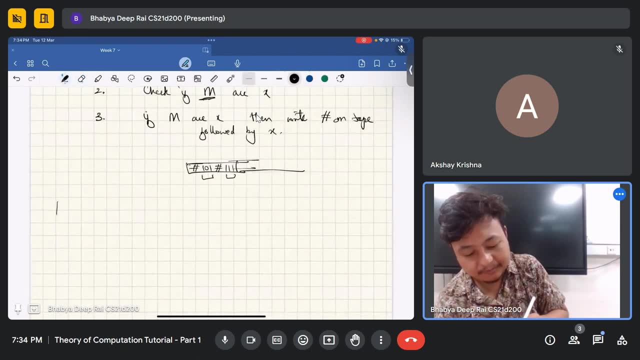 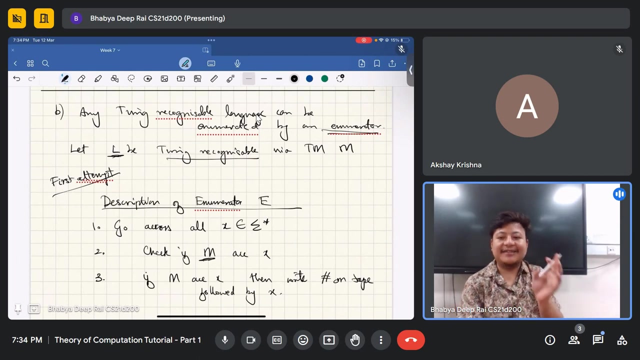 so Okay, here is the problem. Problem is that since the language L is Turing recognisable, we haven't said that L is decidable. So the Turing machine corresponding to it may not be always halting right, It may not always halt. 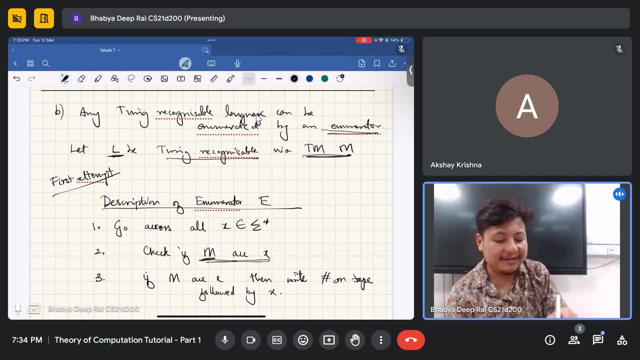 So if I do this check, if m accepts x, when I run it on x I may go across some bad inputs where it may never halt, And as soon as that is encountered, my machine, my enumerator machine, will never print anything after that because it will keep looping in step 2.. 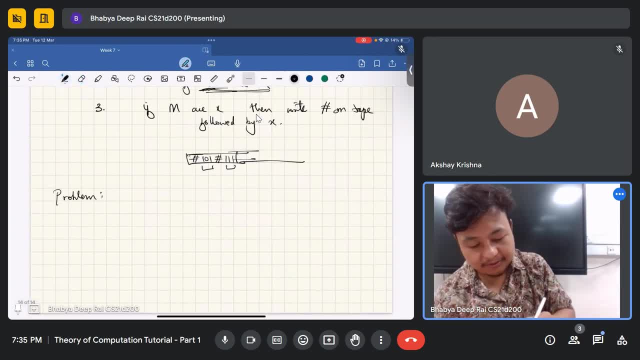 It will keep looping. It will keep looping in step 2.. So the problem is, problem is m may not halt in some inputs because L is only Turing recognisable. We didn't say they are decidable. Ok, Now this is. this seems like a huge problem, right. 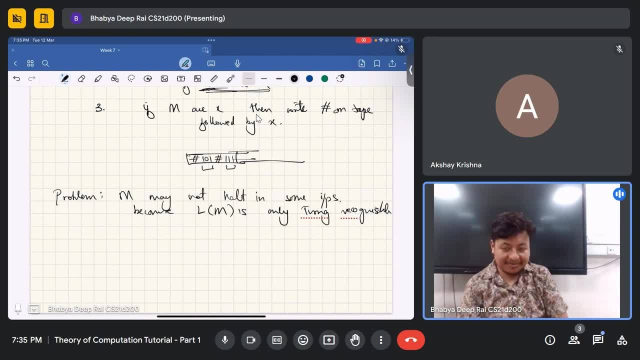 Because now we cannot build an enumerator, But there is a simple thing that we can do: We can do parallelisation. we can run on all inputs in parallel. We cannot run on all inputs in parallel, that is one thing, but we can run as follows: ok, 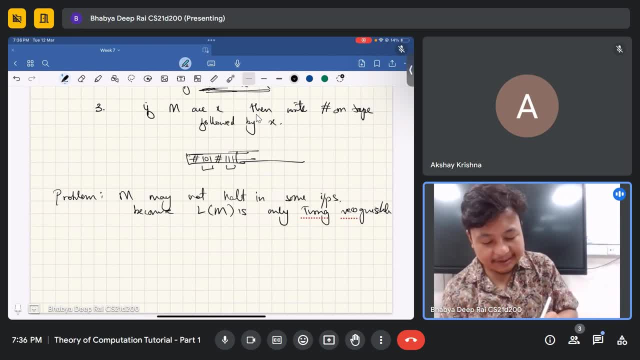 So this is one trick to do it, And that is, let's say, these are the inputs x That look like epsilon: 0, 1, 0, 0, 0, 1, 0, 0, 0, 0, 0, 0, 0, 1, 0, 1, 0, 0, 0, 1,. 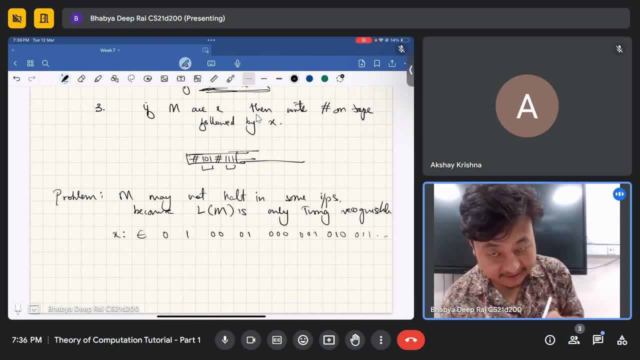 1, and so on. First, what I will do is I will run on epsilon for one step, Then I will run for two steps, And then I will run for one step, And then I will run for two steps And then I will run for one step. 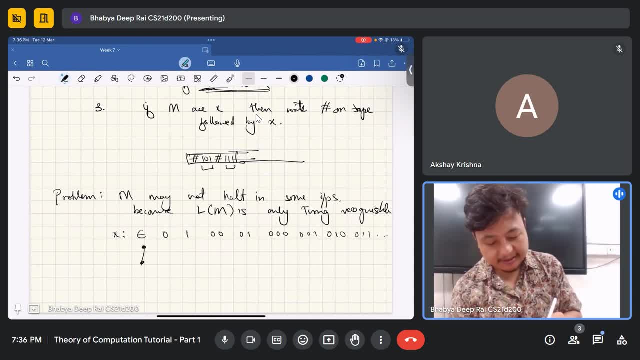 Ok, And this is for two steps. Then I will run on epsilon for one step And for three steps, And then 0 for three steps And one for three steps, And so on, Or I can even do one step each. 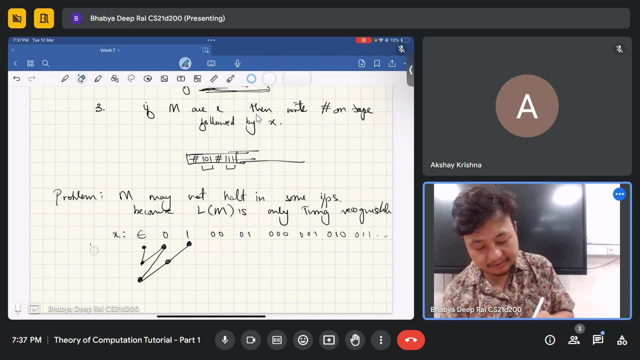 So I will do So: first step, Step two, Step three And ctced. I can run one step each and then zero for once, like I basically continue the computation. okay, so we recall some of the computation we recall on the tape. 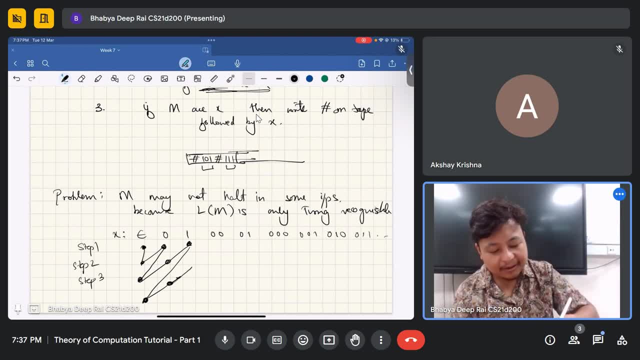 whatever computation we've done, and so this is similar to you know something you would do in operating systems. in operating systems, you, you have this problem of parallelizing processes. what do you do? you just run one process for one a while. okay, one clock cycle, what we call a few clock cycles, and then the 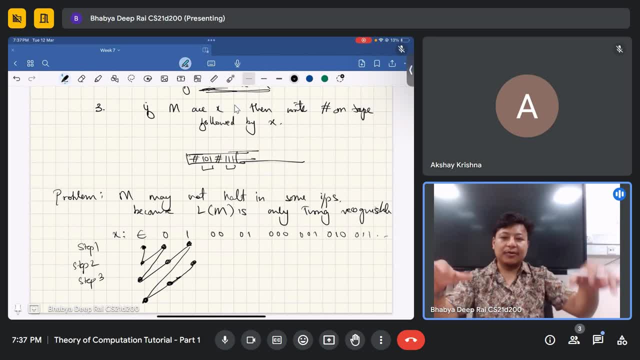 next clock cycle, you run the second process and then you keep doing this, and that is giving you the illusion of parallelization internally. the operating system is not doing parallelization unless you have multiple cores. if you have a single core, then it is achieving parallelization using similar. you are. 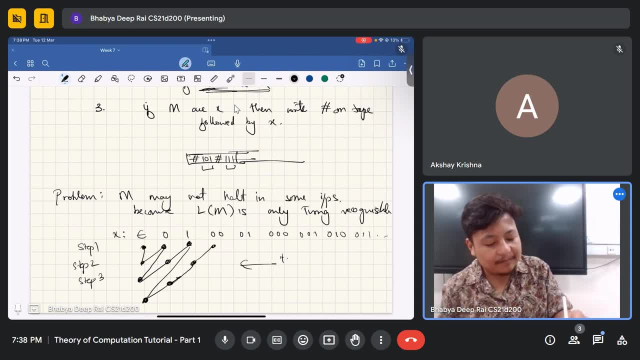 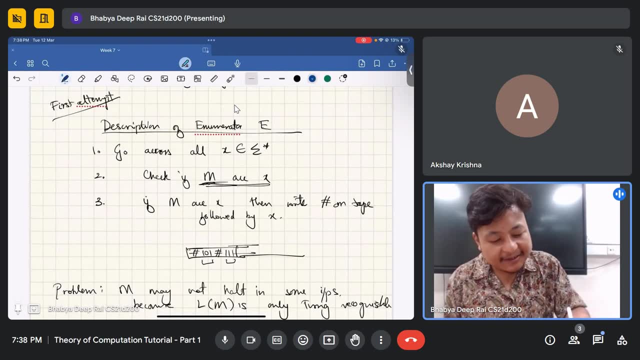 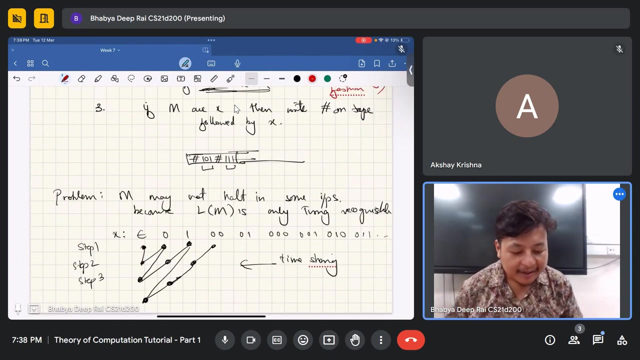 doing a similar thing. so this is what is also called time sharing of the net-term skills. so what do you do? you do: Check M accepts X in time sharing fashion. now if you do this time-sharing process, this time-sharing circus, then what happens is that even if the date say on an input one, it 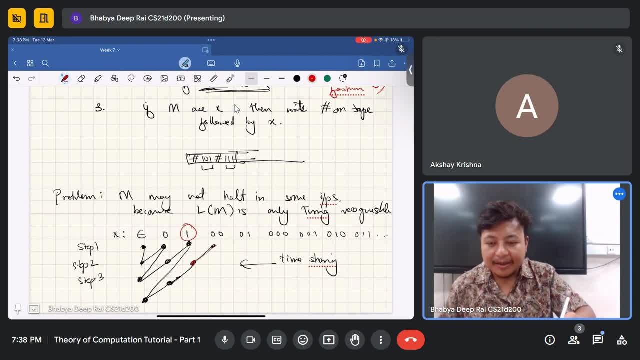 was supposed to loop this time circle would not happen. it would always loop. okay, why does it always loop, right? yeah, I was just watching short, short and I I bypass this and then move to the next input. Okay, fine, in one. it does not, it keeps looping. It's okay. I'll move on to the next strings and I'll try for. 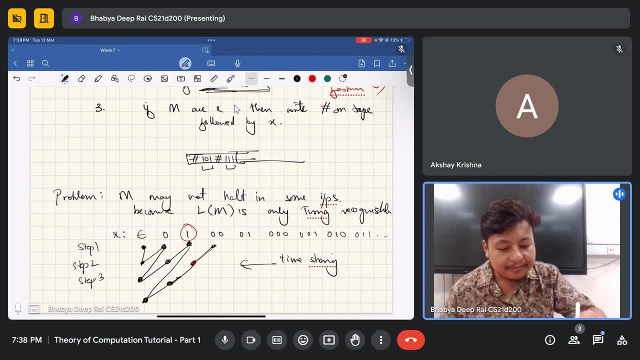 other strings, and if it so happens that you know, for other strings it suddenly says yes, then I'll just output that particular string, let's say 0, 0 for this case, and then the process will just continue without worrying whether for certain inputs my machine will halt or not. and yeah, so then we've built an. 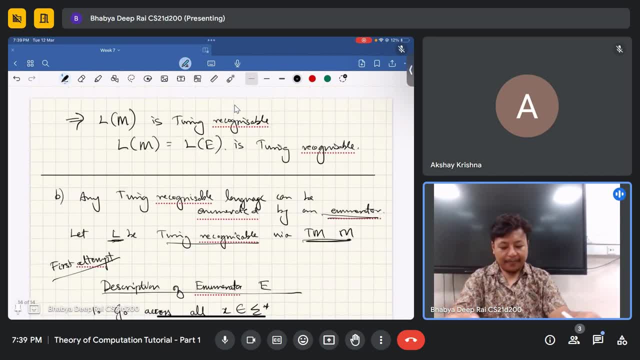 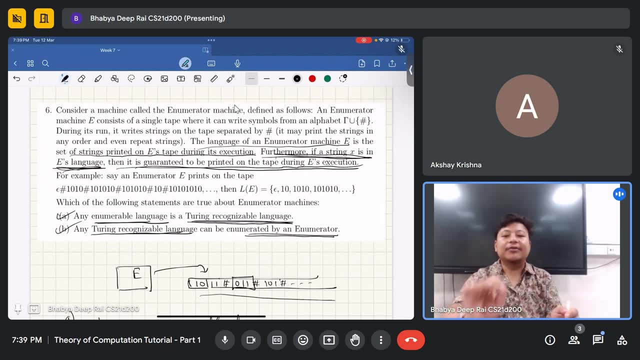 enumerator. so what does that mean? what is the key takeaway? any enumerable language is Turing recognizable and any Turing recognizable language is enumerable. that's why sometimes you may even hear that it is called a recursively enumerable language. Turing recognizable languages are also called recursively enumerable languages and because of this property- that they can be enumerated in this. 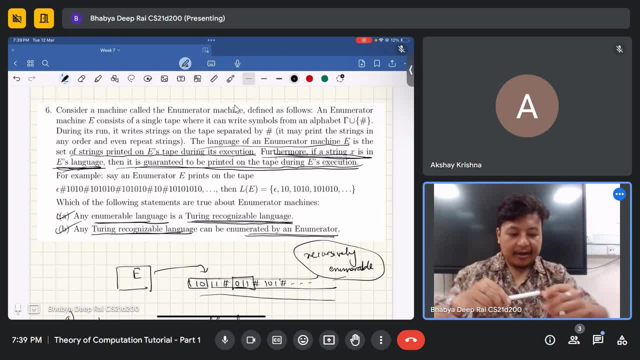 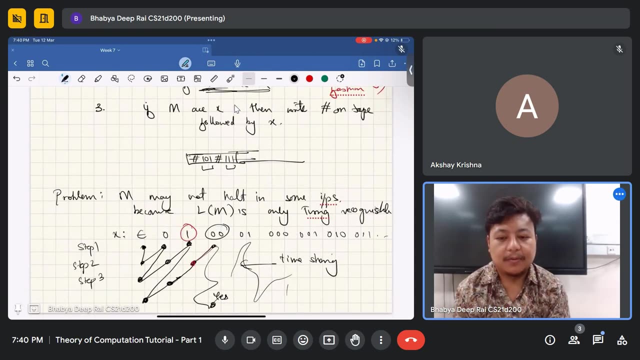 fashion. okay, and okay with that. we've come to the end of the session, so is there anything that you would like to ask? if any additional thing you would like to ask, then otherwise we can wrap up the session now, sir, okay, uh, okay, then the next session will happen on Tuesday, 6 pm, same. 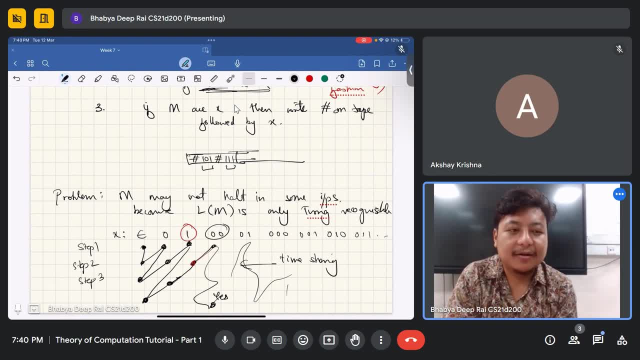 slot- okay, okay, then. thank you. good night, Akshay. thank you, sir, good night, okay, bye, bye.